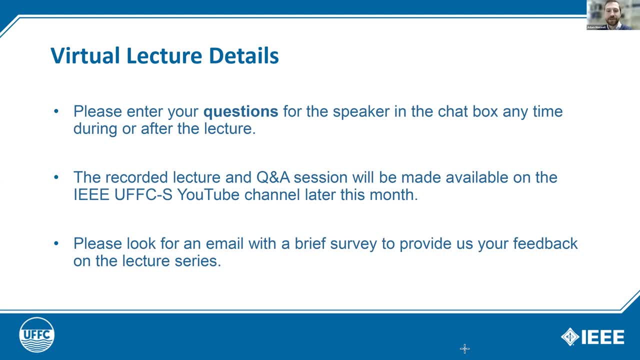 And please also keep an eye out for an email after the lecture With a very brief survey to share any suggestions, Questions or feedback that that you may have. one additional note: There was a hiccup with the naming of the participants in the webinar today. 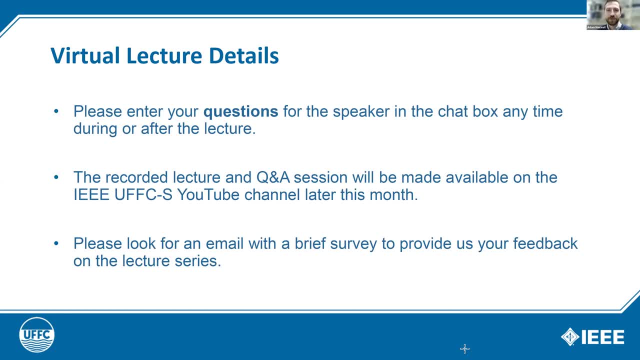 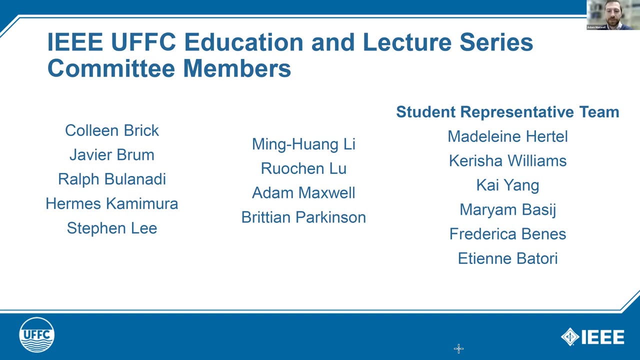 So if you notice that your name is not displayed, please feel free to, to change, to rename yourself, to, to identify yourself, if you'd like. Finally, a huge thank you to all the members of the education and the lecture series committees, as well as our student representatives. 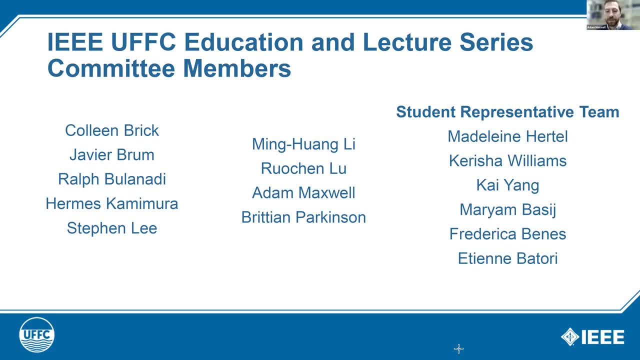 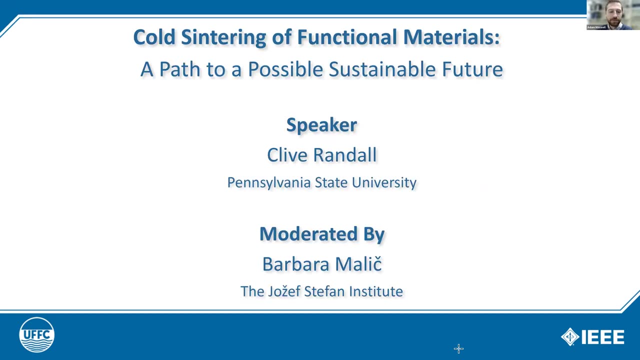 For their help in launching this program. In particular, I'd like to thank Stephen Lee, Ro Chen Liu and Hermes Kamemura for their help with the video editing and captioning, and calling brick for help organizing these lectures. So with that, i'll stop there and turn this over to our moderator. 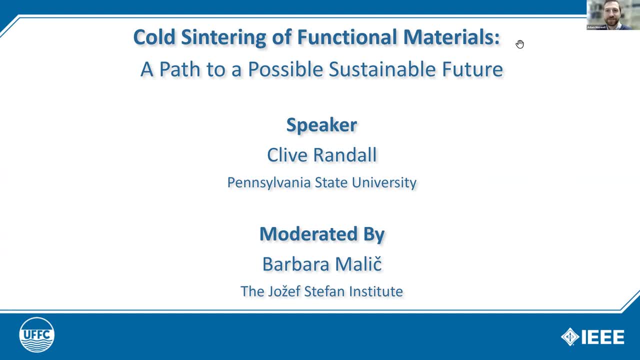 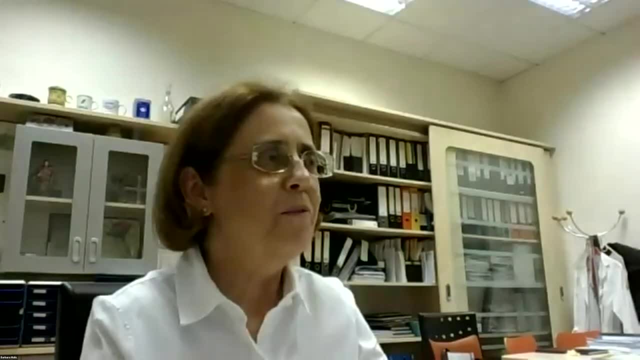 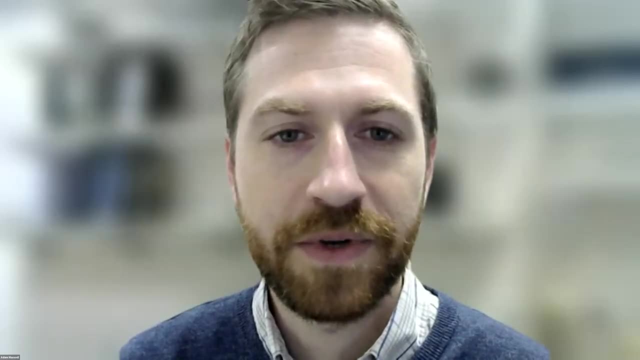 Barbara Malish for introduction of our speaker. Thank you, Adam. Are people saying that They can't hear you? Sure, Adam, someone wrote that they cannot hear you. Oh, they're not able to hear me. Yeah, Can you hear me? 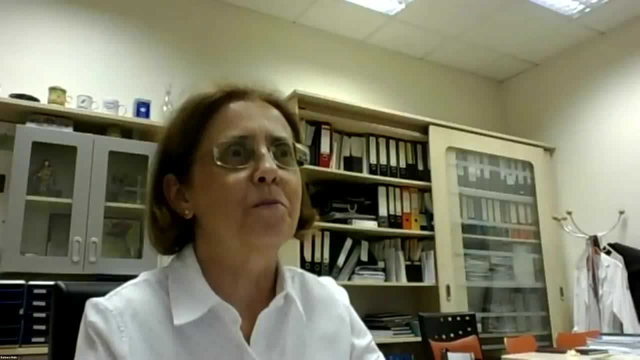 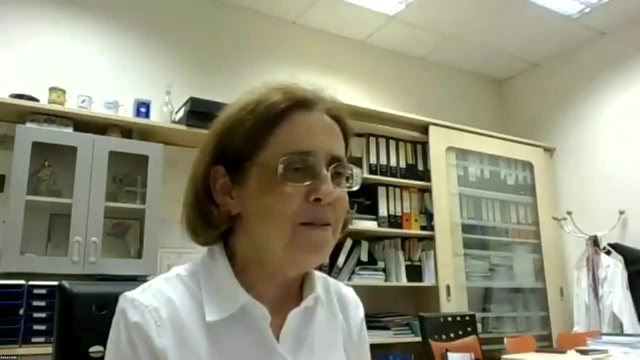 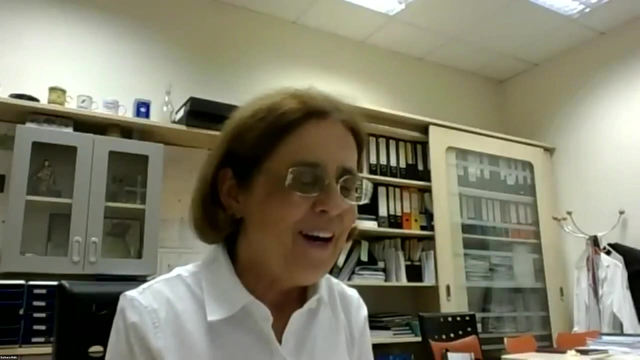 I can now. Yeah, there is a lot of responses, So I hope this problem will be solved as soon as possible. So greetings to everyone. I was introduced. My name is Barbara Malic. I come from Jozef Stefan Institute, from Slovenia, And it is indeed an extraordinary pleasure. 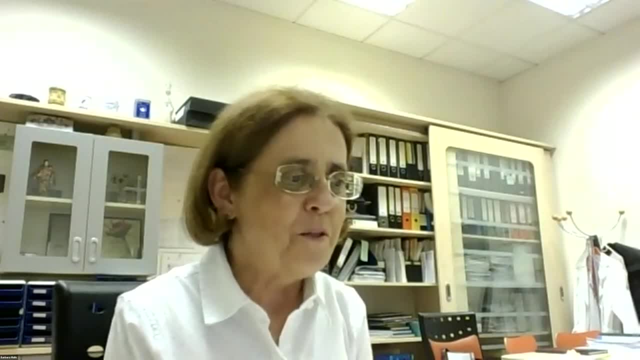 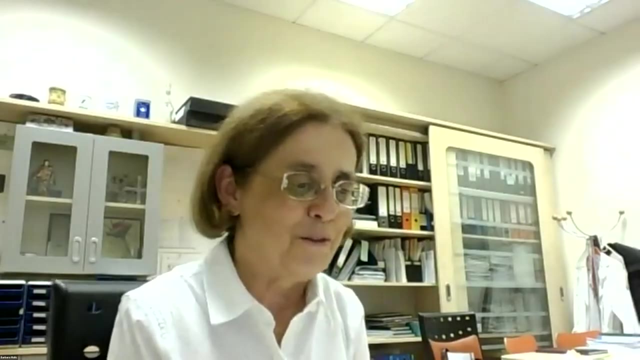 to introduce this inaugural lecture. Today's speaker, a colleague who always has no problem to help or advise, who is an exceptional scientist and teacher. So, Clive Randall, I'm really glad to be in this role. You could read his CV in the invitation mails. 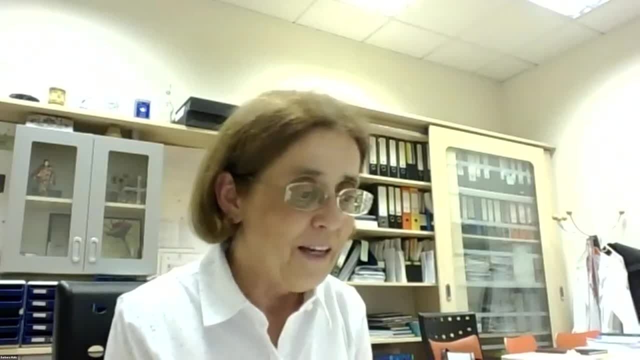 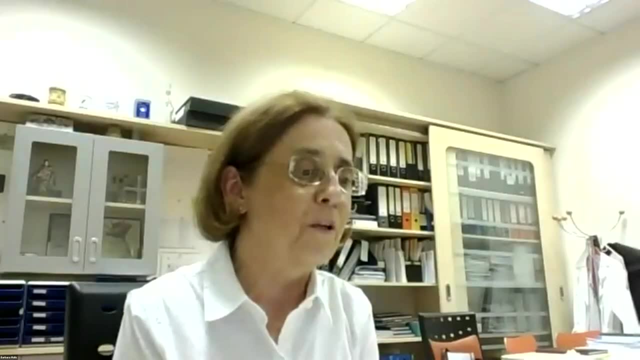 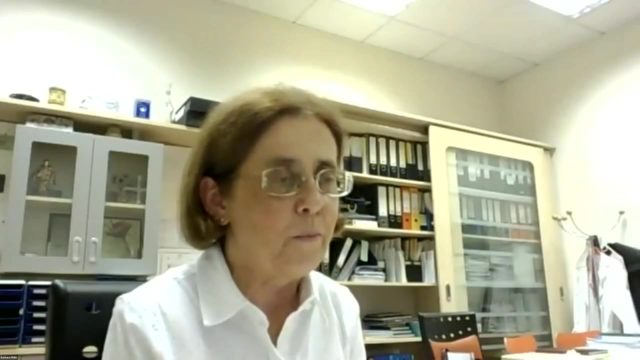 and if you haven't done it, please, It's worth reading. Today's lecture will be about cold sintering, an approach to consolidate materials at very low temperatures And even more. the method allows mixing materials which otherwise, by conventional methods, could not be mixed. I still remember. 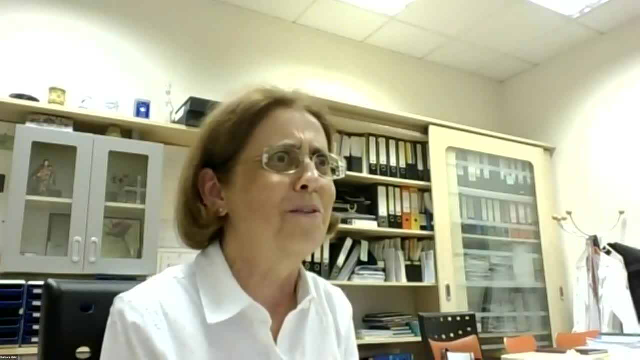 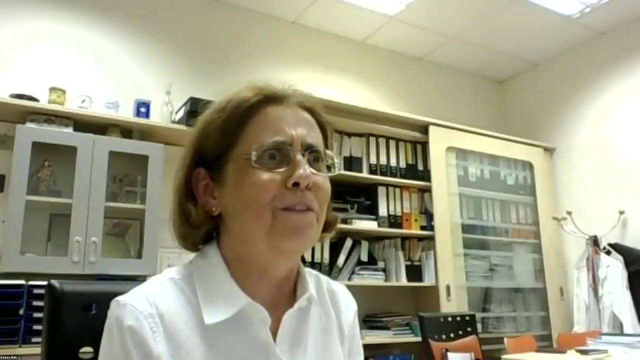 I think one of the first Clive's talks about cold sintering in Darmstadt and a bit earlier at Penn State, And I was really surprised- Keep in mind that I was- I was educated by the fathers of conventional sintering theories And it was such a surprise and such extraordinary result And I'm really 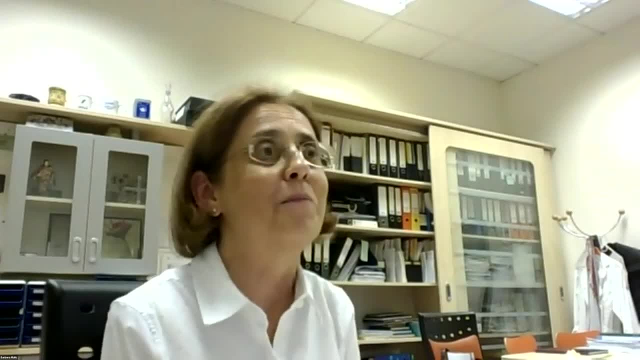 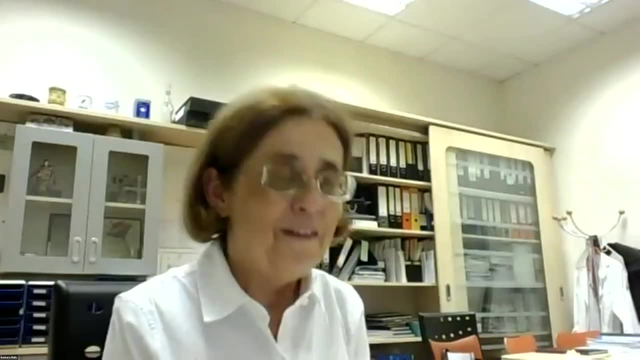 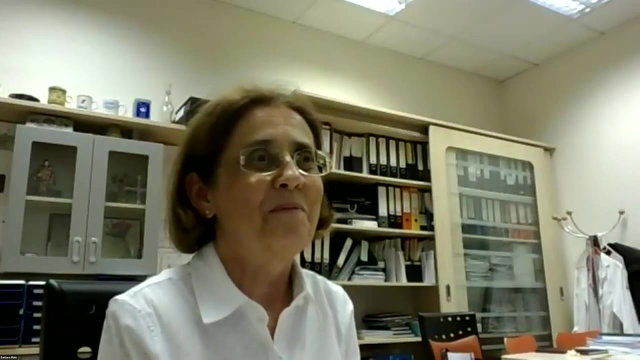 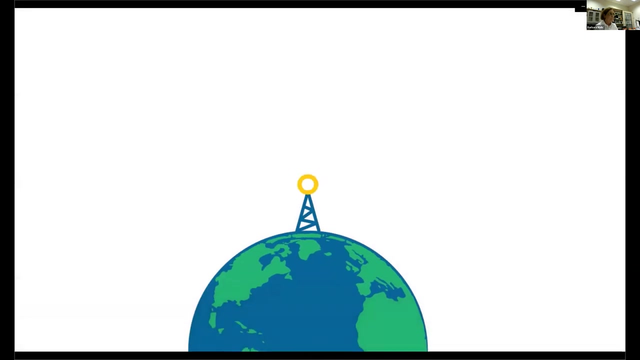 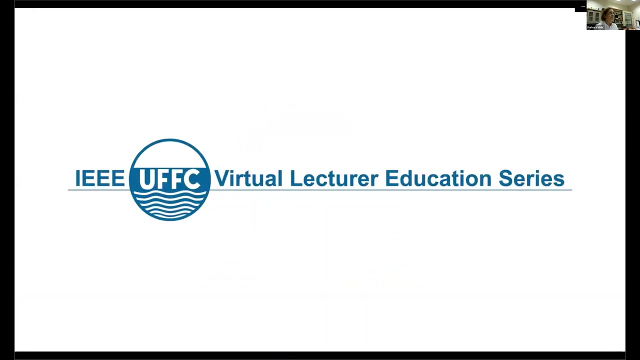 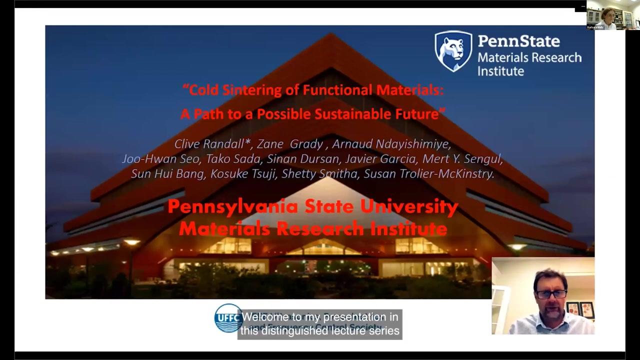 interested to listen to what Clive and his team and other people around the world have achieved in the only five years. So, Clive, the stage is yours and put the questions in the chat box, please. Well, hello everybody. I hope everybody's doing well. Welcome to my presentation. 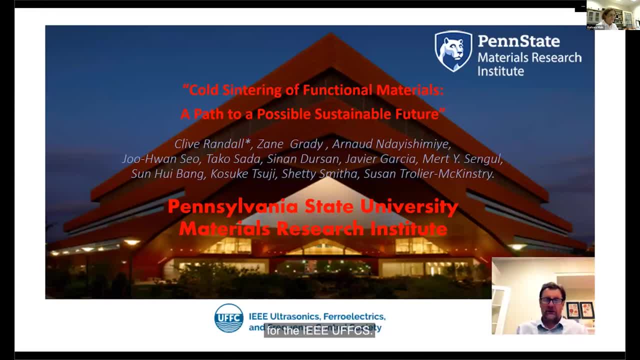 in this Distinguished Lecturer Series for the IEEE UFFC-S. Okay, so what I'm going to talk about today is around a new technology and how it could potentially impact electroceramic devices, dielectrics, ferroelectrics and piezoelectrics. 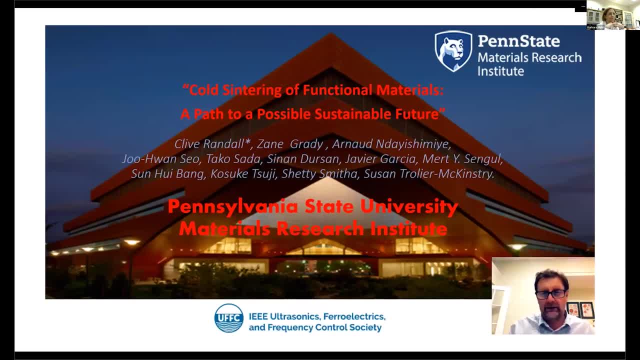 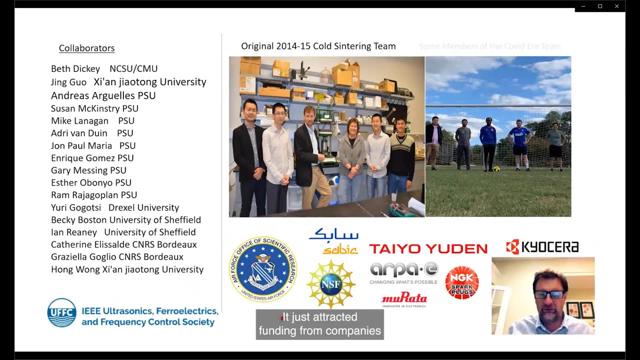 amongst other functional materials. The title is The Cold Scenery of Functional Materials: Apart Towards a Possible Functional Future. This has involved a number of co-authors and obviously a broad number of collaborators. It has attracted funding from companies and also had a number of really talented students and postdocs. 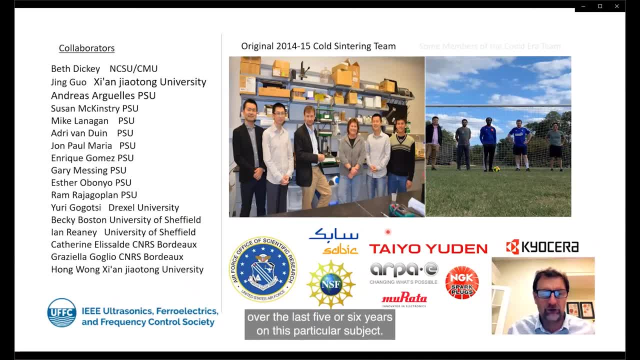 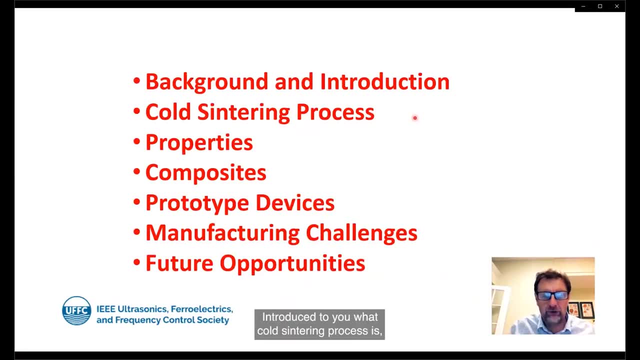 and visiting scientists working with me over the last five or six years on this particular subject. So I'm going to cover a background, introduce to you what the cold-scenery process is, discuss the properties, point out new composite technologies that are possible with it. 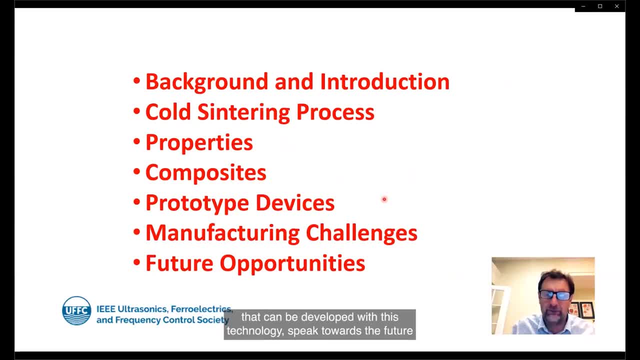 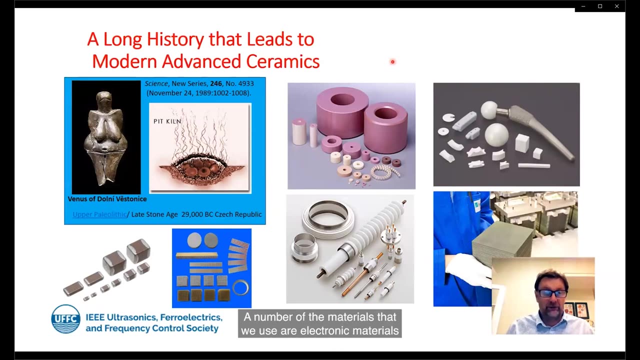 demonstrate some prototypical devices that can be developed with this technology, speak towards the future and their manufacturing challenges, and also talk about other future opportunities. So a number of the materials that we use in electronic materials and devices, including ferroelectrics and piezoelectric materials, include obviously ceramics. 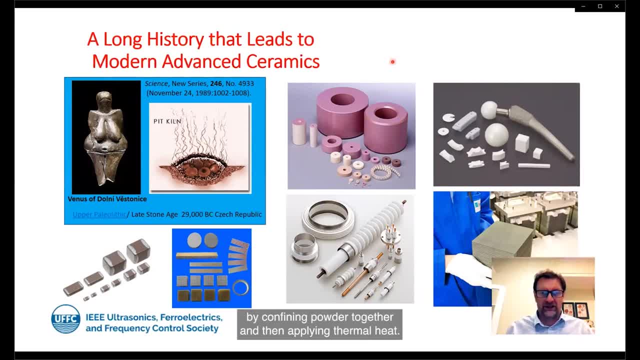 Polycrystalline forms of those are made by confining powder together and then applying thermal heat. That type of technology has been recognized for over 29,000 years. This beautiful artifact here was found in the Czech Republic and reflects from carbon dating. 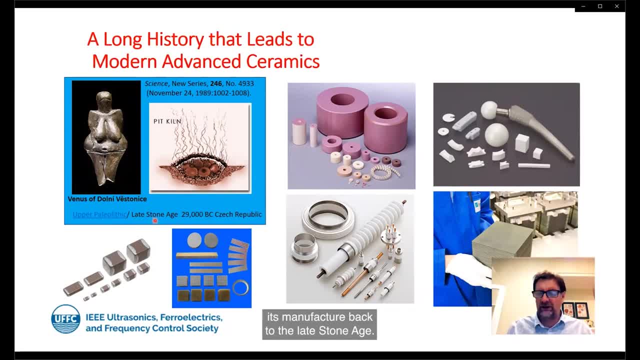 Um, um. it's manufactured back to the late Stone Age. Can you imagine that It's more recent? in the last 50 to 100 years in manufacturing of ceramic type materials has really taken off, and probably really in the last 40 years with the advanced ceramics knowledge. 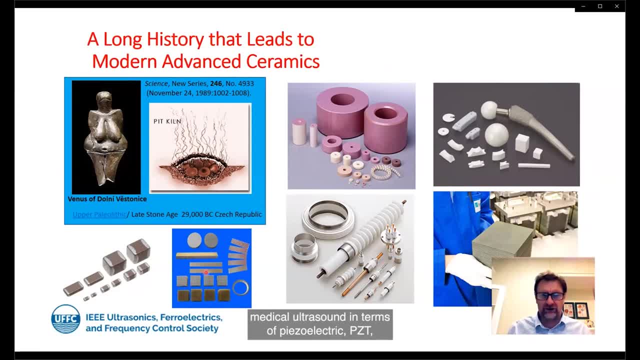 then things like multi-layer ceramic capacitors, medical ultrasound in terms of piezoelectric, PZT, um, uh composites being diced up and then infiltrated with polymers, insulations, fuel cells, biomedical devices and bio implants, and also microwave materials have all been developed, amongst others. 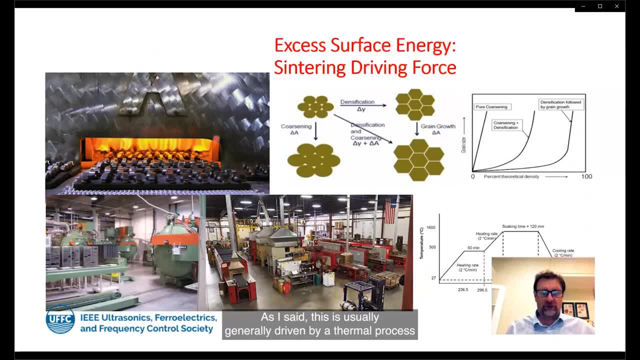 As I said, this is usually generally driven by a thermal process of where particulate matter, where you're taking powder and consolidating it and then driving it with heat in the diffusional processes that are there to basically accommodate the excess surface. energy will then create a dense body by either coarsening the material or creating new interfaces at grain boundaries in order to then drive the densification. 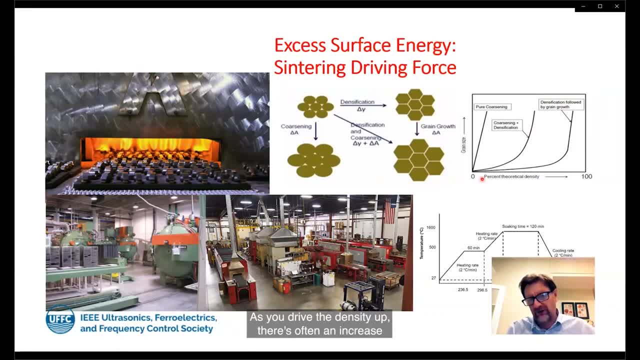 the elimination of porosity. So as you drive the density up, there's often an increase in the grain size as you do this particular process And, generally speaking, most of the ways of doing this- all involve excessive heat at around temperatures anywhere between 80% of the melting temperature of the material in question. 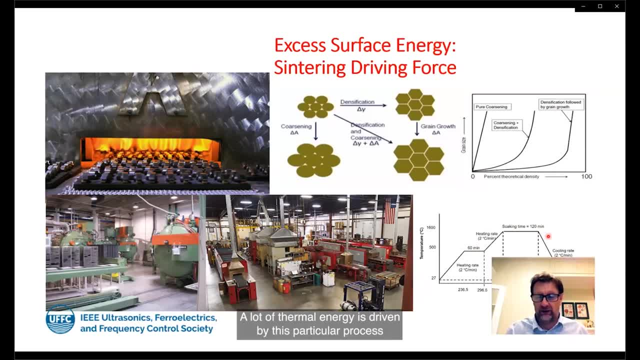 And so a lot of thermal energy is driven by this particular process where you're heating the temperature up, to say, remove binders, to then heat it up to the soaking temperature. you hold it to develop the microstructure and then cool down at different rates. 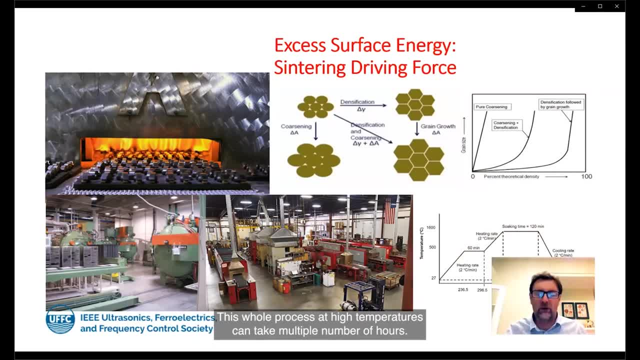 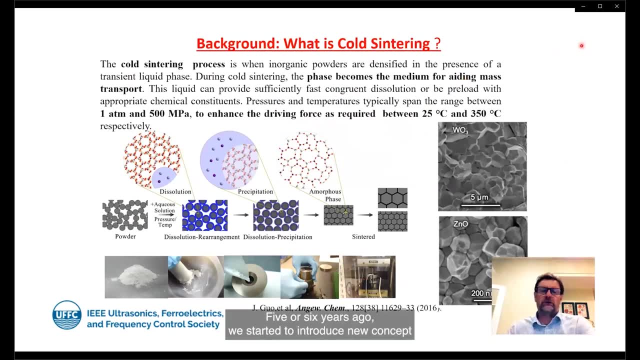 And so this whole process, the process at high temperatures, can take multiple number of hours. About five or six years ago, we started to introduce a new concept which we called cold sintering. We pointed out that cold sintering is linked to a phase. 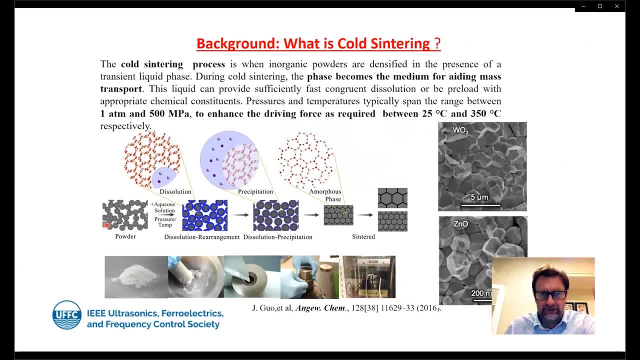 a transient phase that we apply to the powder and in that transient phase must allow dissolution, re-precipitation and densification when having moderate heat supplied to it, anywhere between 25 to 350 degrees Celsius and an intermediate pressure somewhere between 30 megapascals to 500 megapascals, let's say. 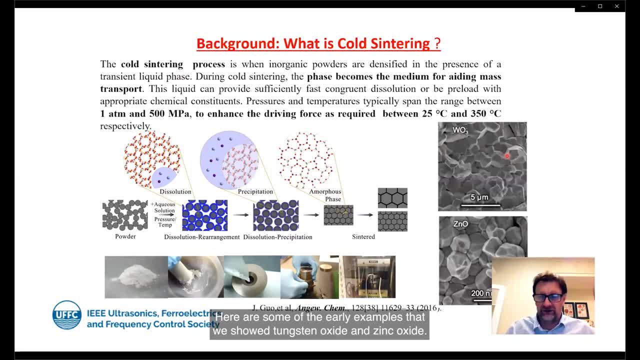 And here are some of the early examples that we've shown: tungsten oxide and zinc oxide. Now we've done over a hundred different materials with this basic process And, as we outline here, it is absolutely a very simple process, I mean. 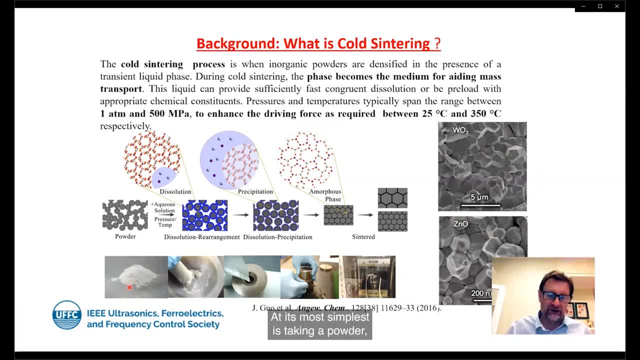 that is most simplest is taking a powder, adding a small amount of transient phase, often in the form of a liquid, And that amount of phase is about five volume percent of the total amount of powder that you're adding, So that powder still flows easily into, say, a dye. 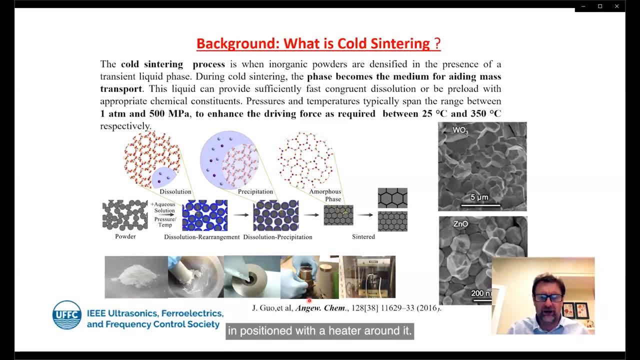 That dye is then positioned with a heater around it and then put under pressure and temperature for anywhere between 10 minutes to two or three hours to then drive a densification process of the ceramic material that we're talking about. So this is what we call cold sintering. 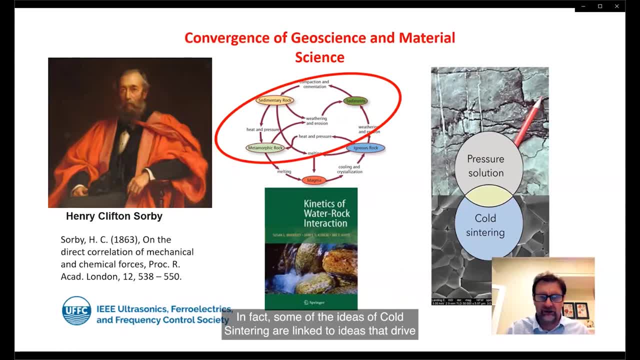 In fact, some of the ideas of cold sintering are linked to ideas that drive the mechanisms that do the densification of, say, sedimentous rock. It was the British geologist, Henry Clifton Thor, who is often honoured at Sheffield University, and he was the first in 1863 to really really start using microscopy to understand rocks at the time. 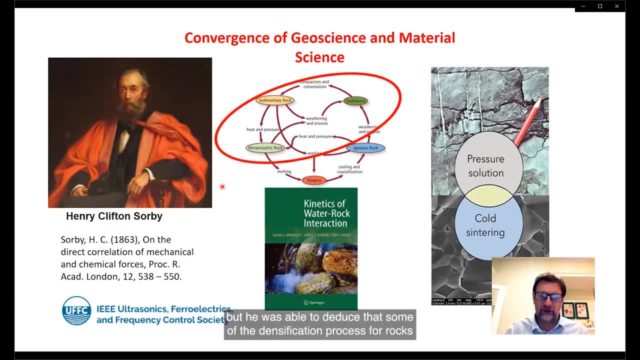 Obviously, the microscopy techniques was optical, but he was able to deduce that some of the densification process for rocks was based upon a mechanical, chemical force, And it is that chemo mechanical force that we are embracing with: cold sintering. It may seem strange to you that we're sintering materials. 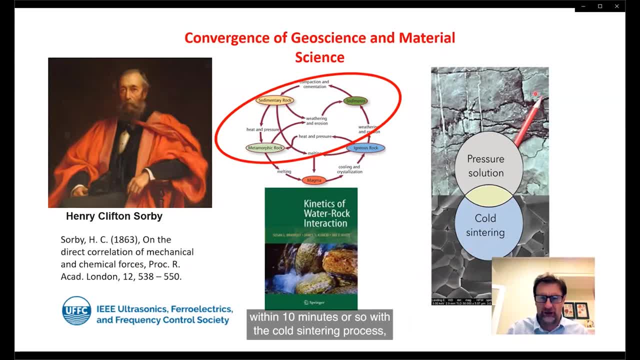 which within 10 minutes or so, with the cold sintering process, but talking of a geological process that can take tens of thousands of years to form densified rocks. But obviously in this day and age we understand the science behind this type of process. 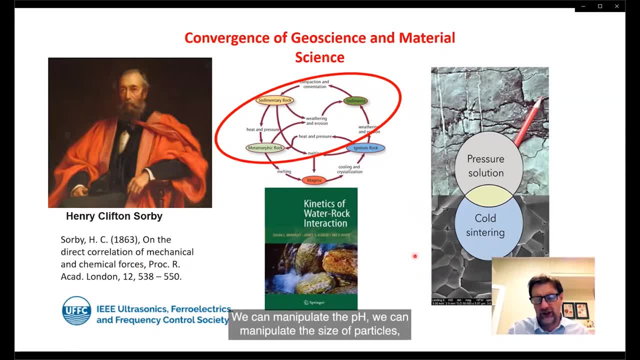 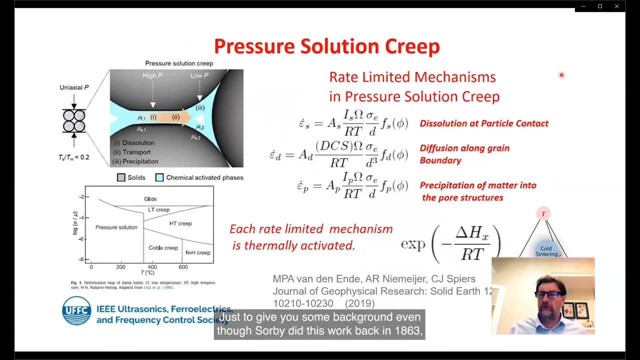 We can manipulate the pH, We can manipulate the size of particles and so forth to really build the kinetics to then drive this densification to a rate which is very interesting for for manufacturing. Just to give you some background, even though Sorby did this work back in 1863,. 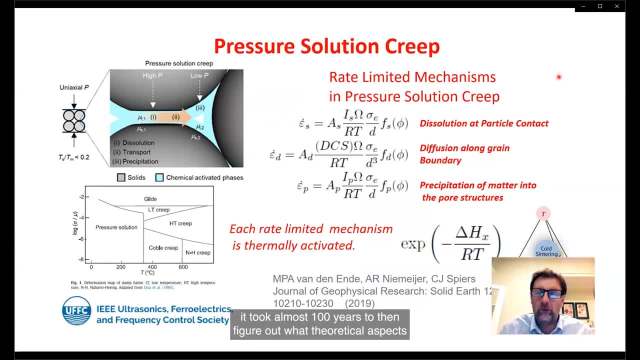 it took almost 100 years to then figure out what the theoretical aspects were that was driving densification. But he did his research and he got what he wanted. And just to give you a little bit of a basic insight into what we're doing in the process, 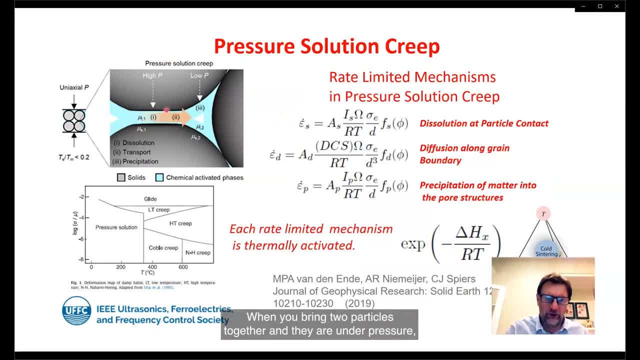 the process is called the pressure solution creep. It's a very, very complex process. It's a very complex process, but it's a very complex process in terms of the nature of the material And that is, you know, this is a very complex process. 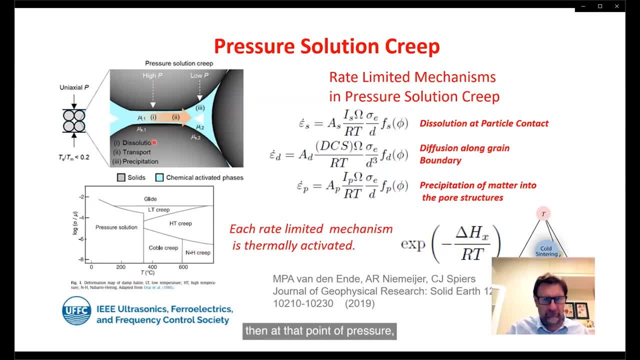 The pressure is often called the sedimentous rock And that process is often called pressure solution creep. And when you bring two particles together and they are under pressure and there is the presence of a liquid phase, say say here, then at that point of pressure 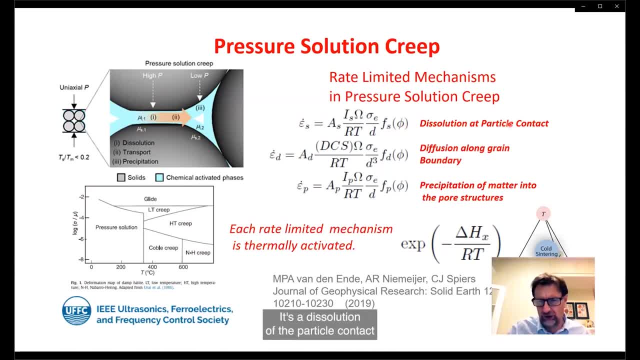 the contact between the materials that can drive a dissolution process. So it's a dissolution of the particle contact. That is the first of the important processes to take place: transport. there's then a concentration gradient that builds up at the point of contact. 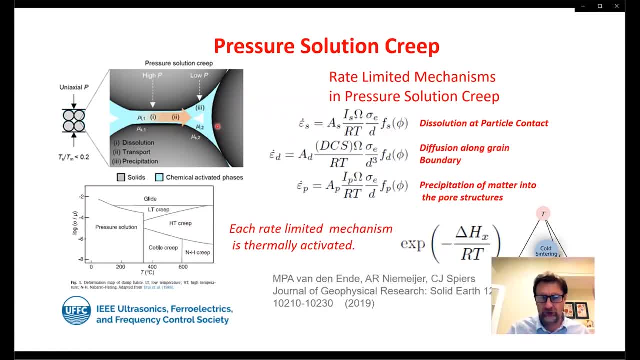 so then regions away from the point of contact, say in the pores, So that builds a non-equilibrium chemical activity difference between these two points, which can then in turn drive a diffusion along those grain boundaries, And then finally in these regions there is also a chemical potential. 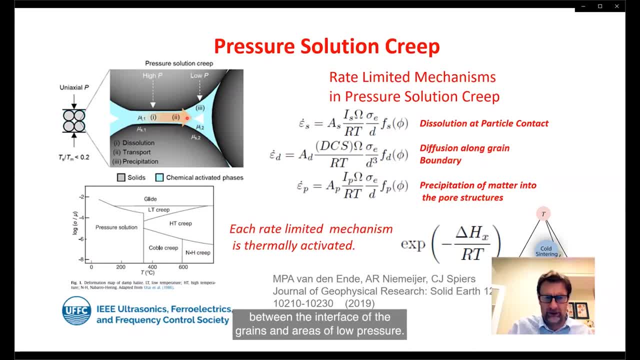 difference between the interface of the grains and areas of low pressure. And there again we then have a driving force to then diffuse this solute and then recrystallize the material epitaxially on these surfaces. So there's three sequential processes: the dissolution, 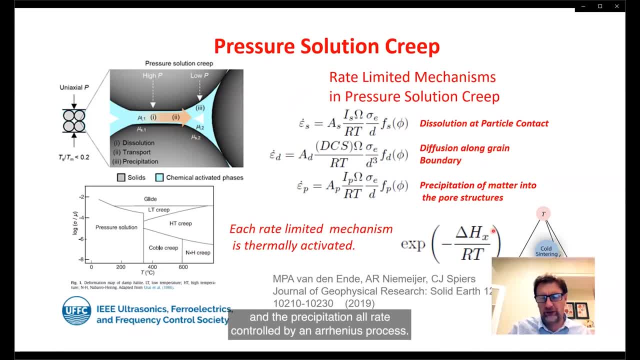 the diffusion and the precipitation. They're all rate controlled by an Arrhenius process. So there's three sequential processes- the dissolution, the diffusion and the precipitation- And each one of these types of processes can be rate limiting to the overall process. 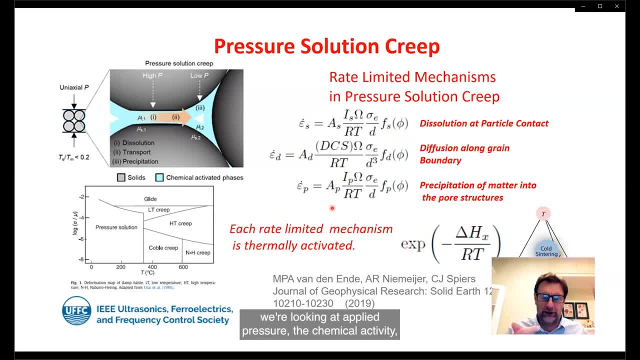 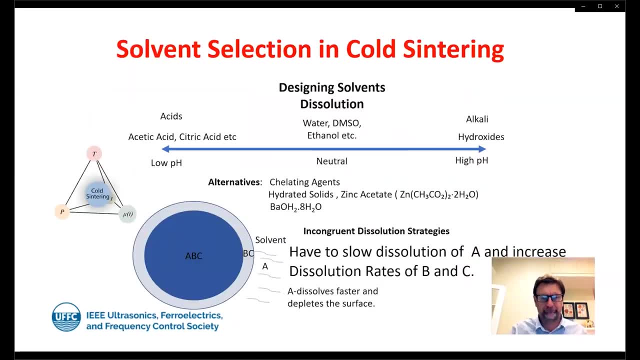 So at the end of the day, we're looking at temperature, we're looking at applied pressure, the chemical activity in time to then drive the overall densification process. Now the dissolution itself can be quite a complicated process. In fact, it is the chemistry and the understanding of the chemistry at those interfaces. 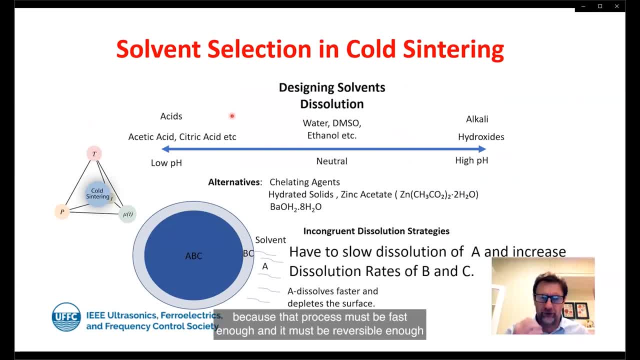 is the most critical thing to do, because they must. that process must be fast enough and it must be reversible enough to drive the dissolution and re-precipitation. So this could take, say, solution chemistry from acids all the way to alkalize. 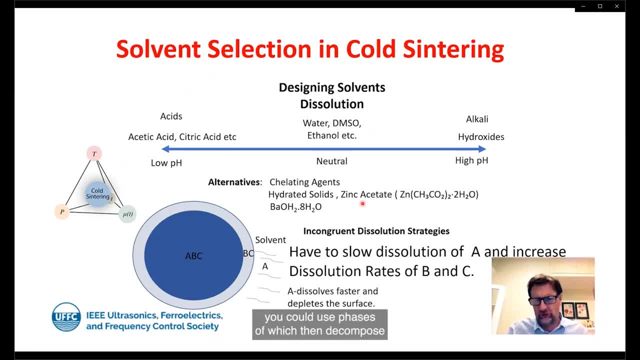 You could use intermediate chelating agents. You could use phases of which they decompose, And drive the decomposition with a dynamic exchange and with zinc acetate, for example, or barium hydroxide hydrate. What you'd be very careful of is understanding that. 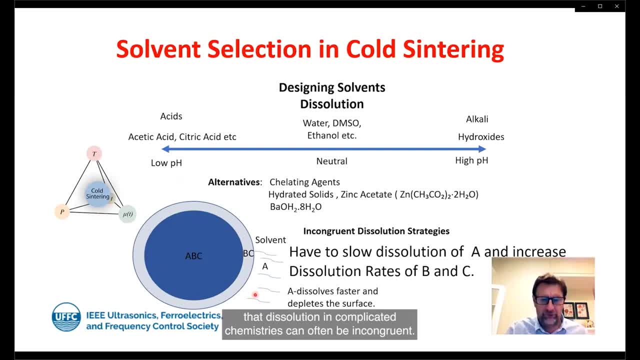 dissolution in complicated chemistries can often be incongruent. Incongruent dissolution is where you have a number of chemical constituents of which there is a difference in the overall dissolution rate between each of those constituents. So, for example, in the case of this hypothetical system, ABC, if A is a very fast process, 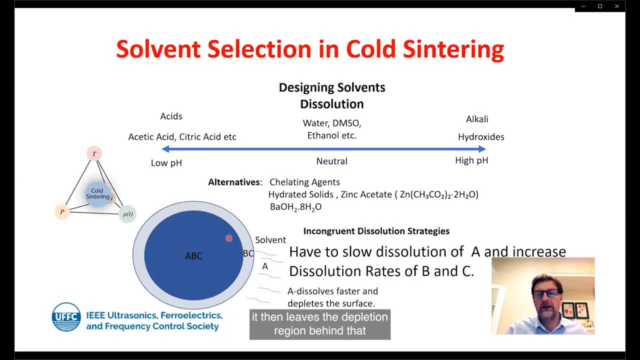 it then leaves the depletion region behind. that then is often of a very different stoichiometry and will obviously then be impactful to then the re-precipitation process and would limit then the re-precipitation on this And obviously you won't have the right chemical constituents. 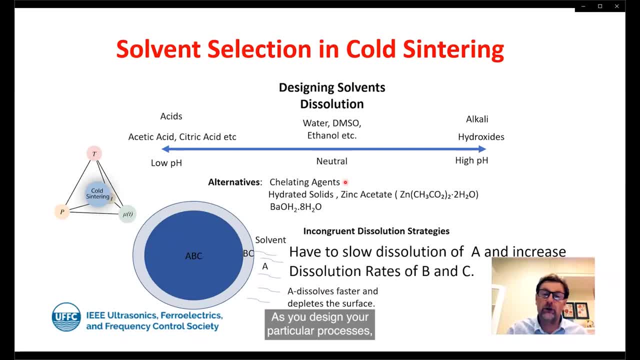 in the solvent chemistry. As you design your particular processes, it's important to try and balance the dissolution process with respect to the bulk rain that you're trying to make and also the kinetics of the dissolution process, to maximize the overall dissolution process and its re-precipitation. 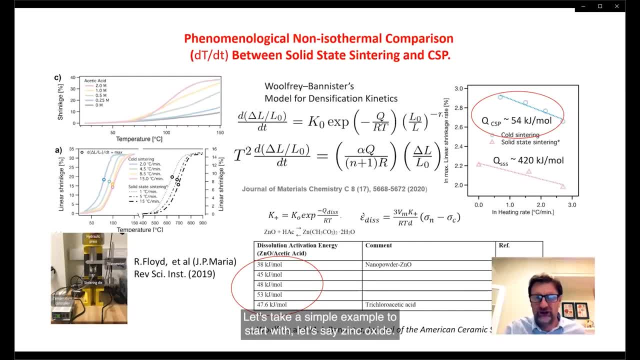 Let's take a simple example to start with. Let's say zinc oxide And zinc oxide, if you just add water, has very little effect in terms of the dissolution and, obviously, densification. So here you're looking at the shrinkage against temperature and all these. 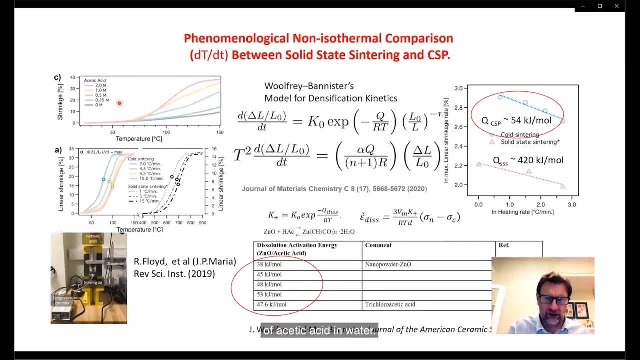 different lines represent different concentrations of acetic acid in water. So all the way up to two moles of acetic acid. You can see. at two moles of acetic acid you're then able to densify with a shrinkage of over 33%. 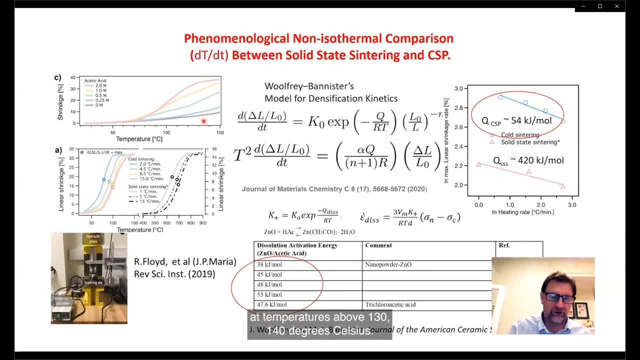 At temperatures above 130, 140 degrees Celsius. You can then look, say, with concentrations of about two moles of zinc oxide And then look at the different heating rates it takes to then drive the densification, And you can see here various different densification rates between two degrees per minute. 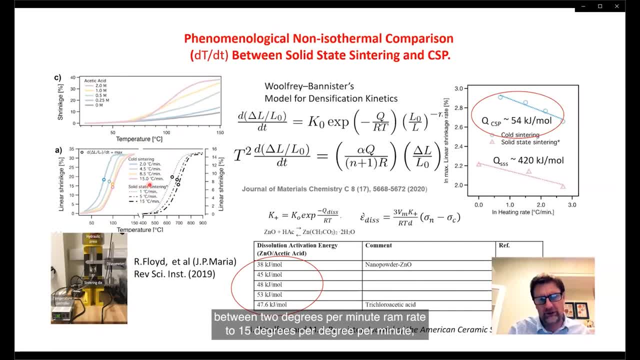 ramp rate to 15 degrees per degree per minute, it being studied against more conventional sintering. with the case of zinc oxide, and in analysis of these types of densification data with techniques such as the wolfrey banister densification model, you can extrapolate out what the controlling rate kinetics are in terms of the 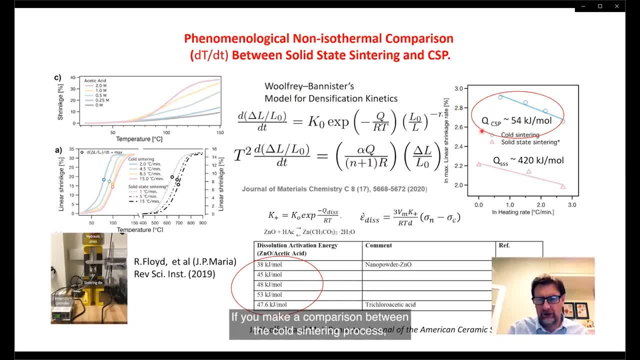 activation energy. and if you make a comparison between the cold sintering process- it's about 54 kilojoules a mole- to the normal solid state sintering, which is around 420 kilojoules per mole. so a massive difference in the kinetics of these two systems. and if you then make a 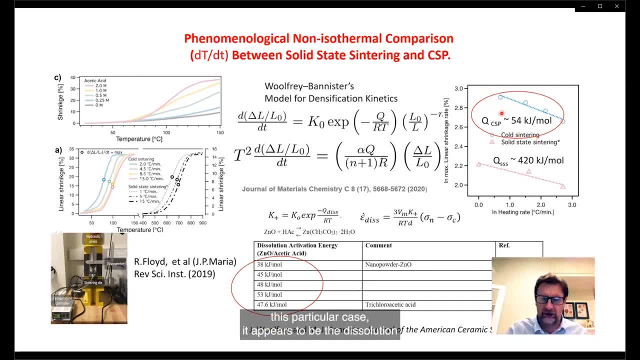 comparison to what could be controlling this particular case, it appears to be the dissolution of the zinc oxide in in the acetic acid. here's some data that is published by a number of different authors of that particular dissolution rate and you can see this matches very well with the types of rate control kinetics that we are seeing for this. 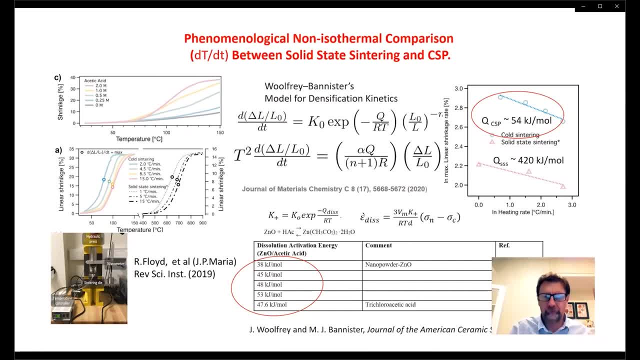 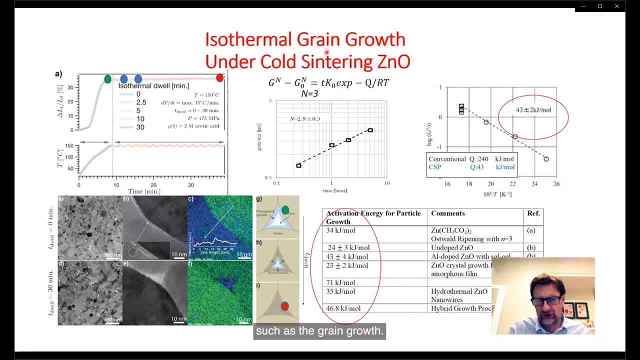 particular densification, and we can also look at the kinetics under isothermal conditions, such as the grain growth, and we have seen that with grain growth this fits a activation process of where there is an exponent n and that n turns out to be three, which is a very attractive 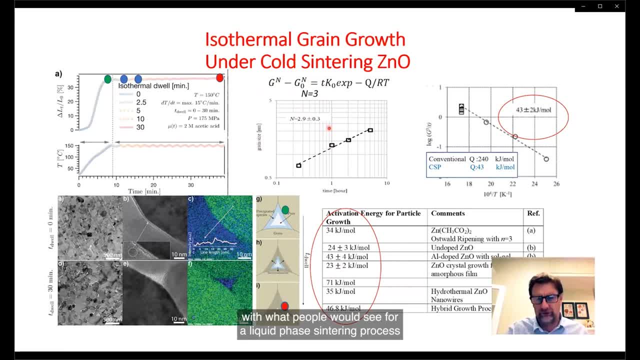 number, because that's very consistent with what people would see for a liquid phase sintering process of where there's a diffusional step between the liquid phase interface and the growing grains and the activation energies for this in the case of zinc oxide is around 43 plus or minus. 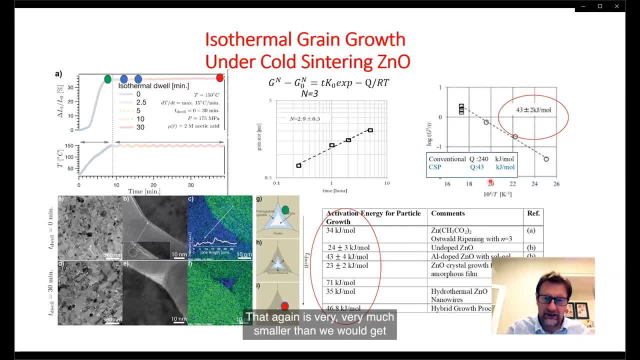 two kilojoules per mole, and that again is very, very much smaller than you would get with conventional sintering, which is about 240 kilojoules per mole. and again making comparisons, we see that the actual coarsening of a grain or costing of a particle in solution, growth of zinc oxide well matches this. 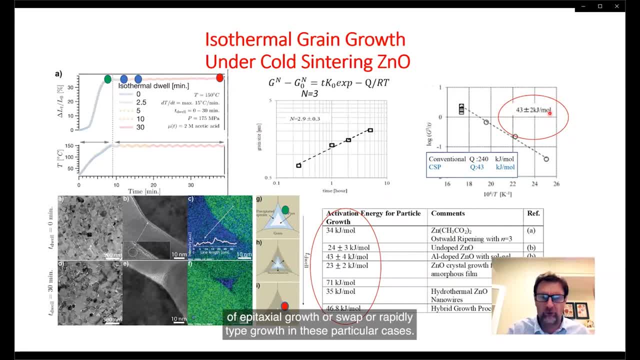 type of of epitaxial growth or also ripening type growth. in these particular cases we can see some details, even in this one simple ramp up to 150 degrees and then, looking at them, the evolution of the microstructure between eight minutes which we call zero time, but eight minutes to heat it up. 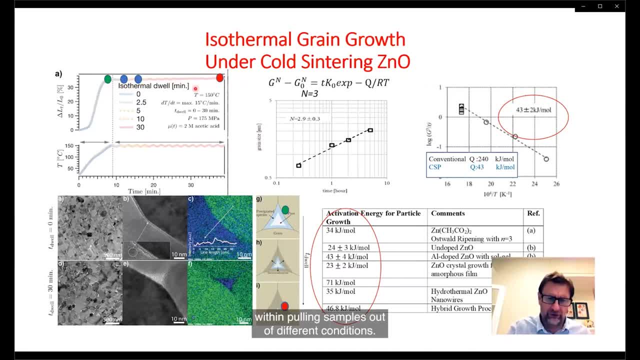 and then over the next 30 minutes. we've been pulling samples out at different conditions and what we've seen is that there's grain coarsening occurring even at this low temperature, in this little window. but, more importantly, the interface has been very well maintained and we have seen that. 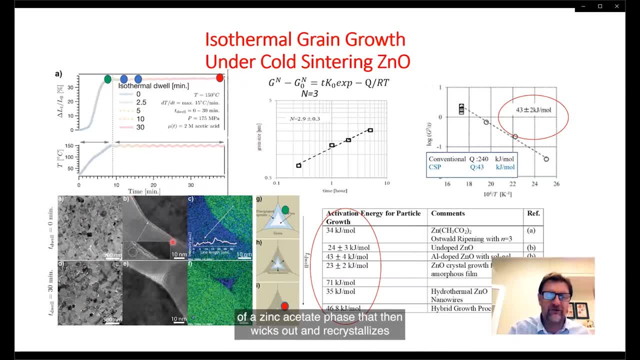 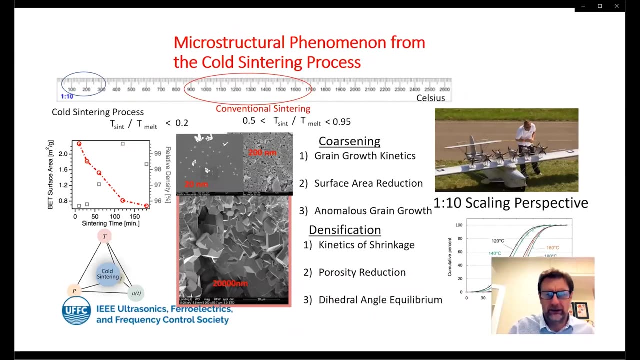 there seems to be change to. we can see the performance of the amount of lead in the compositionbridged level of the MAGQ. energy do the temperatures, and that gives us completely new perspectives on how to make materials and it ticks off all the boxes that you can associate with scenery, grain growth, surface. 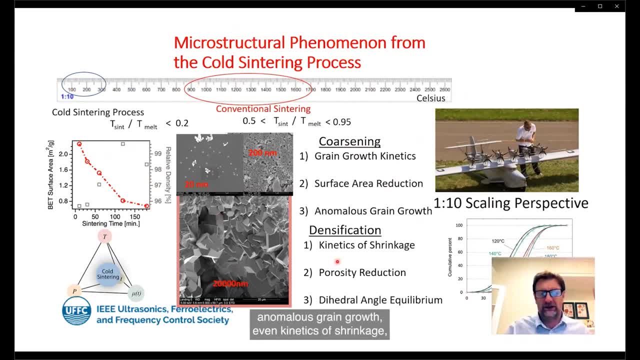 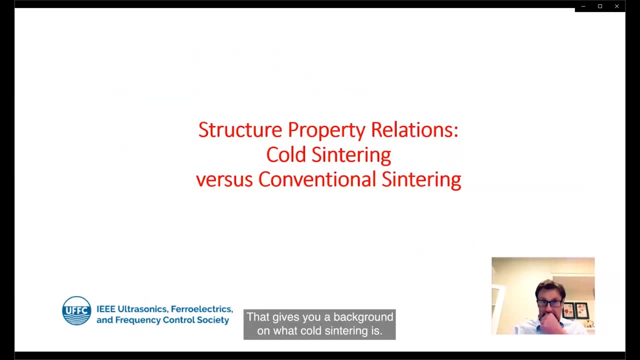 area reduction, anomalous grain growth, even kinetics of shrinkage, which i've just talked about, porosity reduction and dihedral angle variations driving towards an equilibrium state. okay, so that gives you a background on what cold centering is. now, how does cold centering impact? 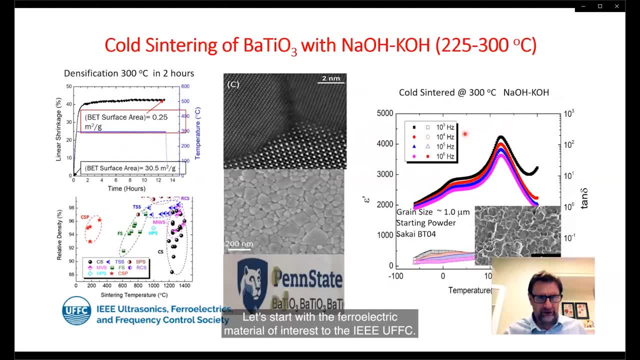 properties. so let's start with a ferroelectric material, material of interest to the ieee uffc. so let's look at the cold centering of barium titanate. well, this, we started off with annealing this, enabling this with a sodium hydroxide, potassium hydroxide, and was able to center. 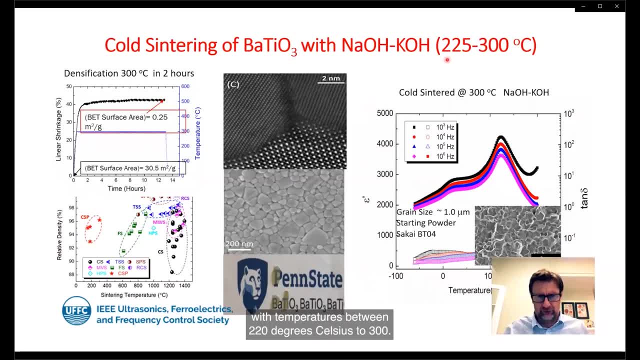 barium titanate in a single step with temperatures between 220 degrees celsius to 300. typically you center barium titanated 1200 or more. you can see here within an hour. we are able to densify the material, but there is continuous coarsening within holding at this particular isothermal condition of 300 degrees. so when? 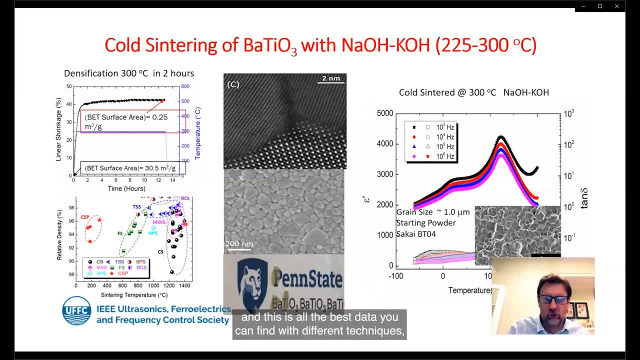 you compare the relative density to all the other methods- and this is all the best data. you can find techniques: Fast sintering, two-step sintering, microwave sintering, hot ice, static pressing, cold sintering, etc. This really stands alone as a new technology. 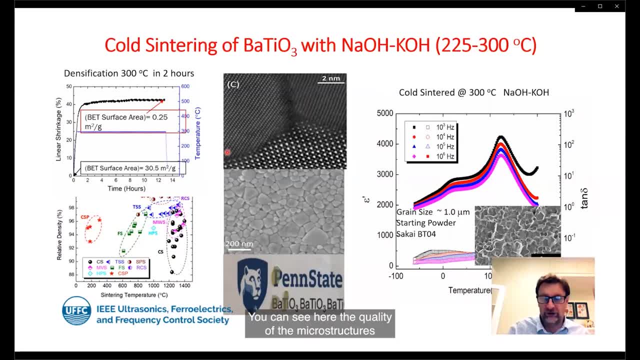 for them developing dense materials. And you can see here the quality of the microstructures and even see that these fragments, here that there's a path towards making very transparent barium titanate based materials. The dielectric properties are also quite spectacular. You can see here: 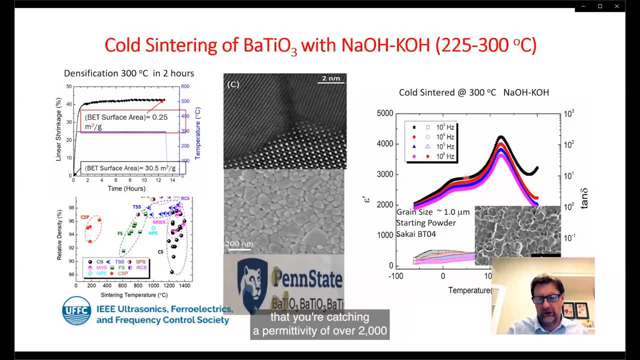 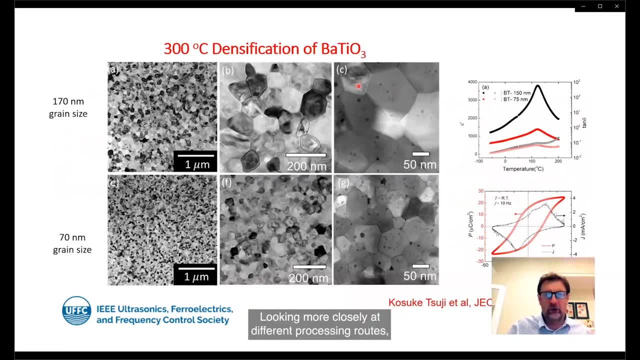 at room temperature, in this particular case, that you're catching a permittivity of over 2,000 with a very nice microstructure. Looking more closely at different processing routes, you can see that you have a chance of controlling the overall grain size in these materials. 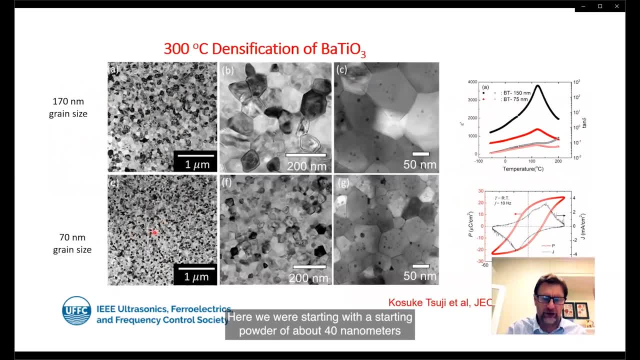 Here we were starting with a starting met powder of about 40 nanometers, but you can see here 70 nanometer grains and here 170 nanometer grains, And here is the differences in the two respective grain size: permittivity temperature. 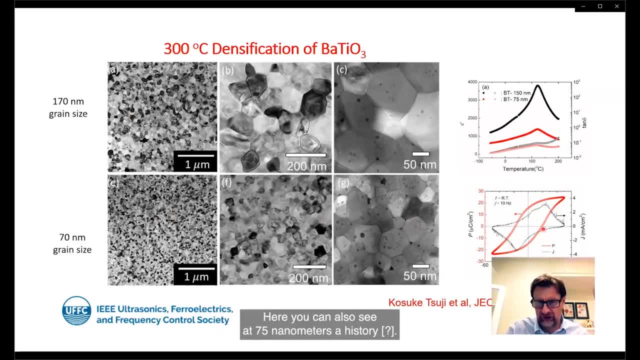 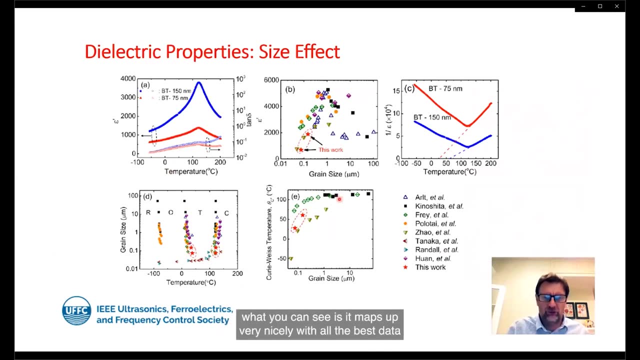 dependent properties, And here you can also see, at 75 nanometers, a history sysloom. When you look in detail at all the size effect data that could come from that type of study, what you can see is that it maps up very nicely with all the best data that you can see in regard to size effects. 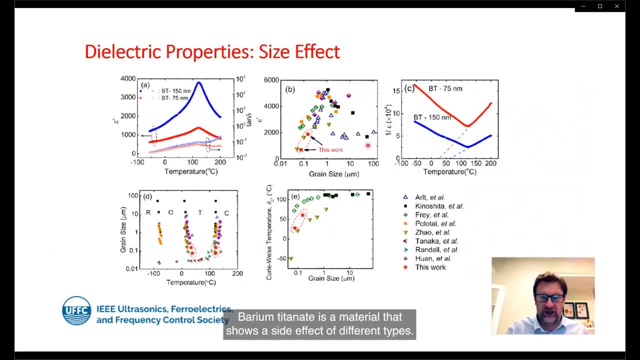 And barium titanate is a material that shows a size effect of different types. There is a first of all enhancement of the permittivity up to about one micrometer. below that it then drops down And then eventually there is also a shift of the Curie temperature. 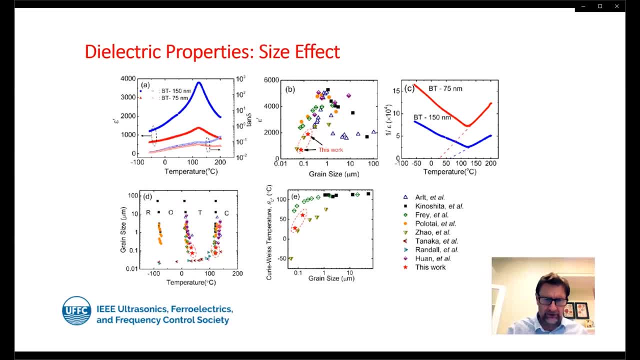 And then eventually there is also a shift of the Curie temperature. And then eventually there is also a shift of the Curie temperature. You'll notice that with respect to smaller and smaller sizes, Eventually the ferroelectricity can more be sustained in a single particle or a single grain, and that's below sizes of about 13 nanometers. 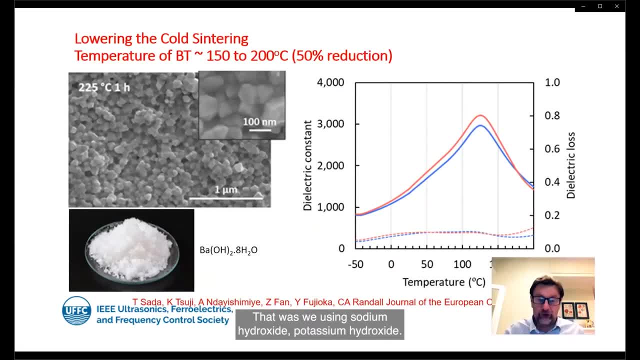 So that was using sodium hydroxide, potassium hydroxide. We moved on to then see what we could do at even lower temperatures. The hashes later why that is important. So we'd see the total desulfur kissed around 150 nanometers. so when that's out, the takes activity's a percentage and thenricked. So then it would be about lubricating the hashes in a way that would allow them to Sasha likely to act, and they're full of oxygen. So there was this. So that was what we were talking about. No matter what you're trying to do, it might not be done. 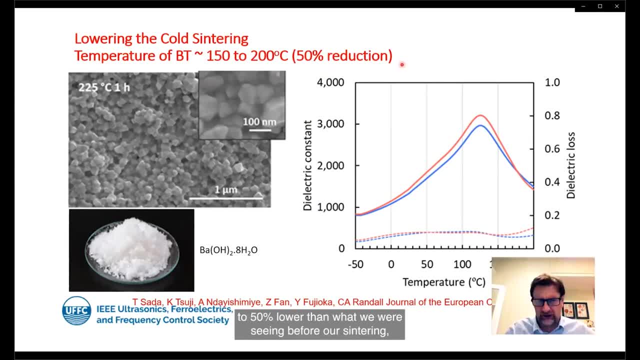 So we worked very hard to reduce the sintering temperature to 50% lower than what we were seeing before. So now we're sintering as low as 150 degrees just above the Curie point. Can you imagine? Even the thin film processes that people use with Sol-gel are much higher temperatures than this. 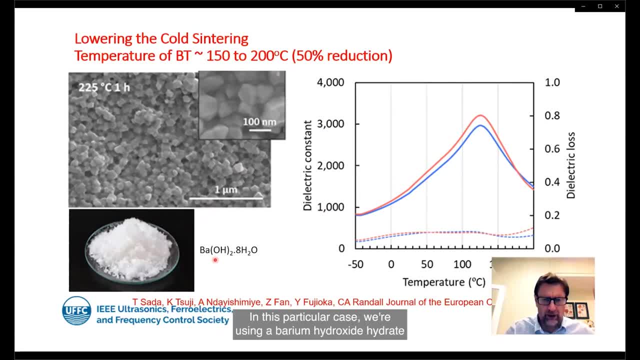 And in this particular case, we're using a barium hydroxide hydrate, which is a solid phase that is intimately mixed with the powder and then, on the controlled dehydration conditions of this hydrate, which then drives a densification of the barium titanate powders. 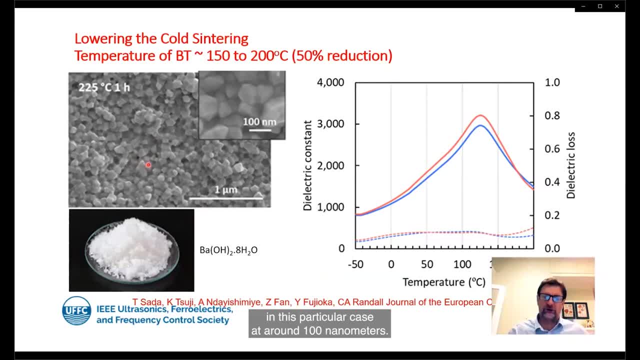 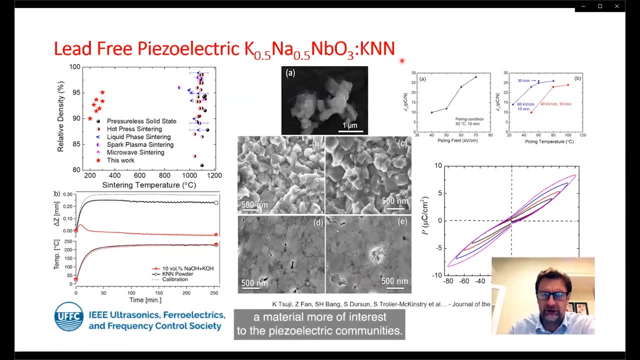 that were starting, in this particular case, at around 100 nanometers, And you can see here again very attractive permittivity data and loss data. Okay, so to show another ferroelectric material. in this particular case, a material that we're using is a ferroelectric material. 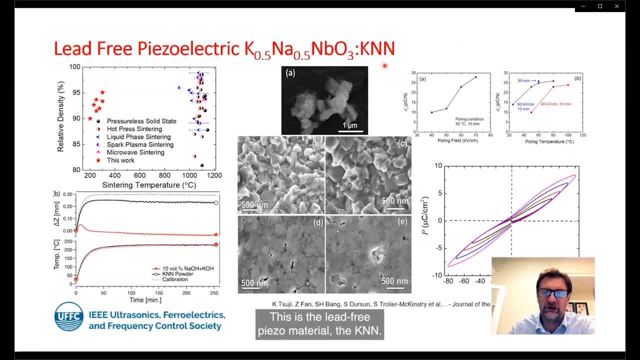 that we're using is a ferroelectric material. This is a material more of interest to the piezoelectric community. This is the lead-free piezo material, the K&N, And in this case, again, we use a sodium hydroxide, potassium hydroxide. 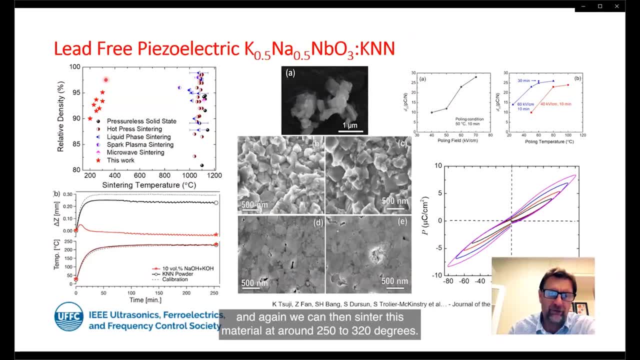 And again, we can then sinter this material at around 250 to 320 degrees, And this is very low compared to most of the other techniques. You can see here a variety of other techniques being all limited to around 1,000 degrees. 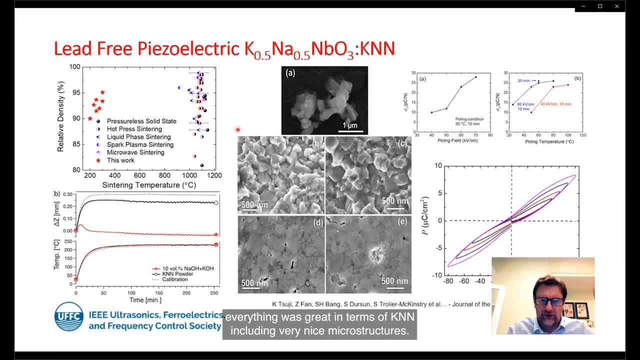 So, densification-wise, dielectric property-wise, everything was great in terms of K&N, including very nice microstructures. The bad news was, in this particular case, that the overall dielectric properties were rather limited compared to conventional sintering. 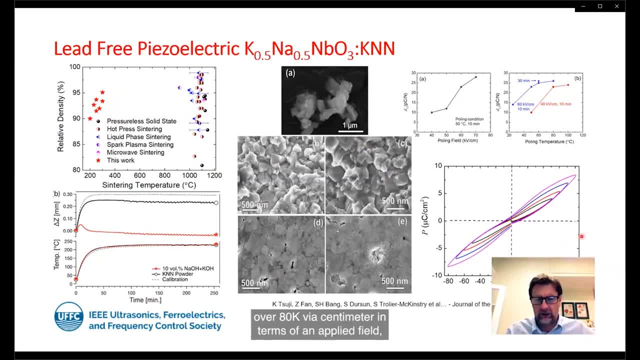 And you can see here with the PE loop, even though we're exceeding over 80 kV a centimeter in terms of an applied field, the loop is very pinched And this implies a very difficult switching of the ferroelectric domain to then pole the material and hence limiting the overall piezoelectric properties. 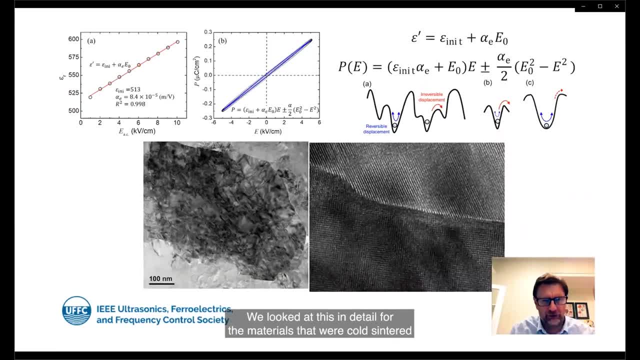 We looked at this in detail for the materials that were cold-sintered And what we concluded? through the use of a Raleigh analysis, which is a great way to analyze nonlinear domain contributions to the overall piezoelectric properties, we found that there was a lot of permittivity in piezoelectric properties. 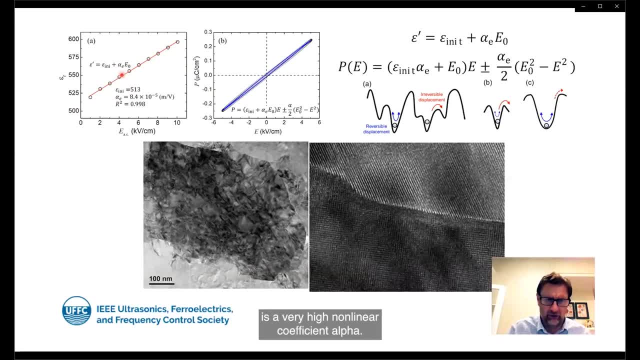 And what typically you need to have in a very good piezoelectric material is a very high nonlinear coefficient alpha. Now, this was about an order of magnitude lower in the cold-sintering cases relative to the sintered cases. The reason for that was revealed through a TEM study. 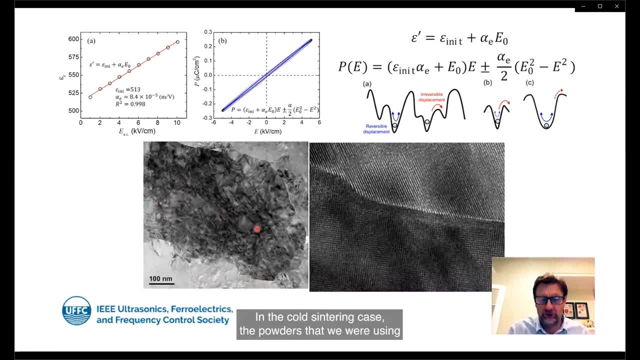 In the cold-sintering case, the powders that we were using had very, very high densities, densities of dislocations. Grain boundaries were very clean. so it was not the result of any problem with the grain boundaries. It was all to do with the interior of the grains. 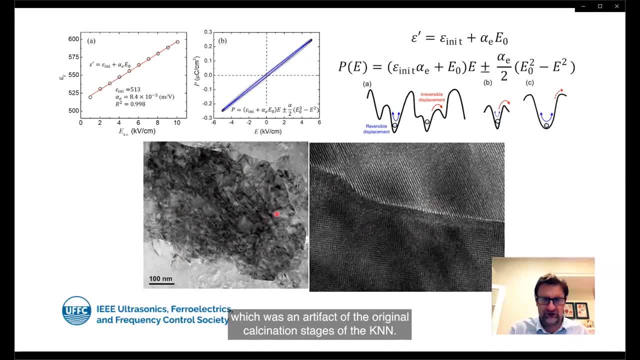 which was an artifact of the original calcination stages of the K and N. So we are now looking at this type of material much more closely from the calcination stage and then seeing if properties can then improve with the cold-sintering. But what this points out is that in the cold-sintering case, 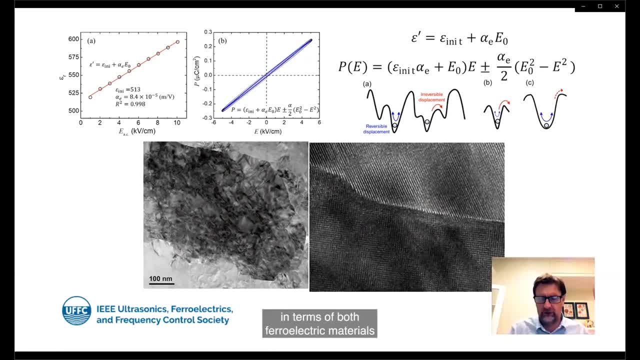 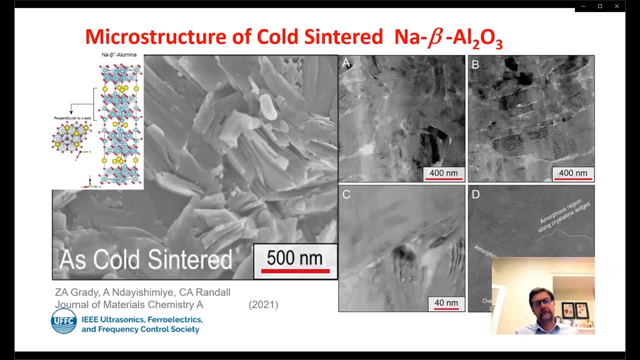 there is a lot of promise in terms of both ferroelectric materials for dielectric applications and or piezoelectric applications. And just to point out it is not just about ferroelectric properties- and to just show you an extraordinary result, 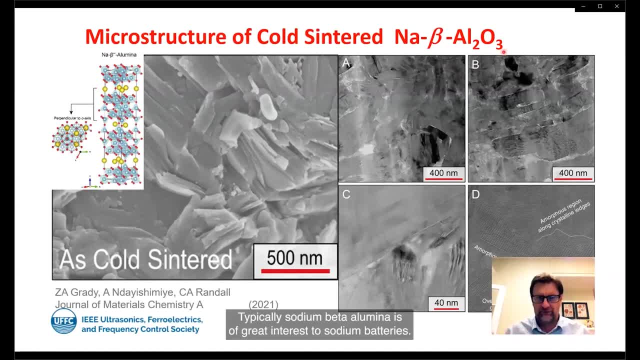 So typically sodium beta or aluminum is of great interest to sodium batteries And as an electrolyte this material typically centers between 600 and 1,650 degrees to 1,700 degrees Celsius. We are sintering this material around 350 degrees to a very high density. 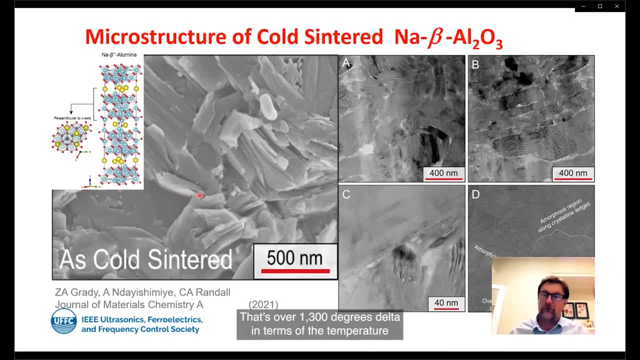 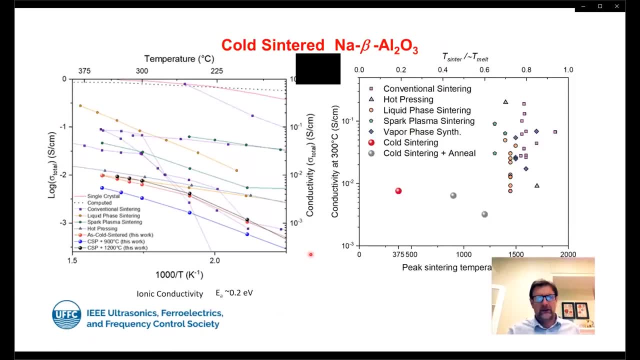 So that's over 1,000 degrees, over 1,300 degrees delta. in terms of the temperature of making this particular material, The properties are a little bit down, but this is within an order of magnitude given the differences in the temperature. 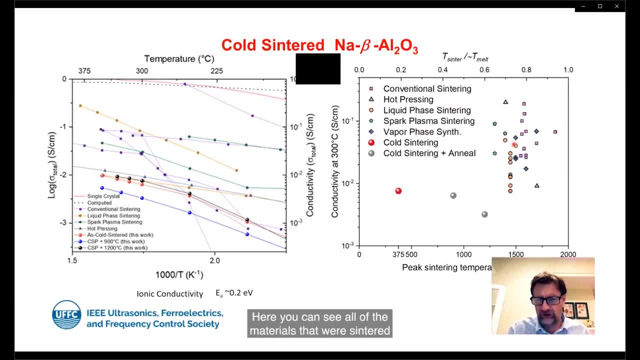 Here you can see all of the materials that were sintered, say, above 1,500 degrees, where the grain sizes get a lot larger and there's a lot less interfacial resistance at the grain boundaries. Obviously, here the grain sizes are very, very different. 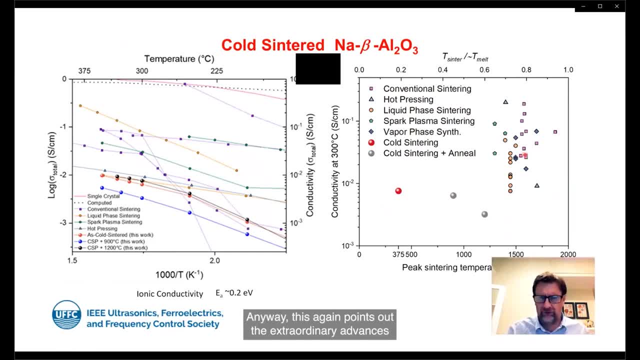 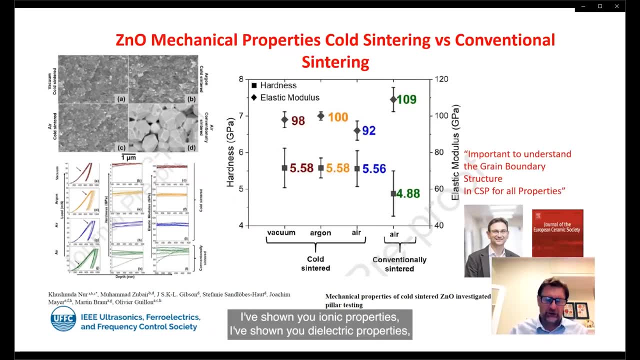 But anyway, this again points out the extraordinary advances that can be made in the cold-sintering. So I've shown you ionic properties, I've shown you dielectric properties, I've shown you some of the challenges for piezoelectric properties. 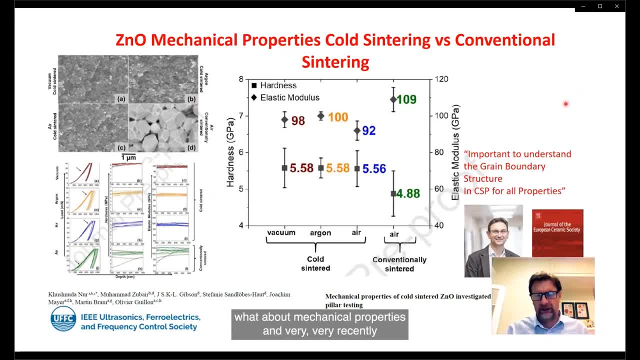 And there's often a question: at these low temperatures, what about mechanical properties? And very, very recently, so recently. you can see the preprint is still in process online, But the group in Jülich has done an excellent job in terms of understanding the cold-sintering. 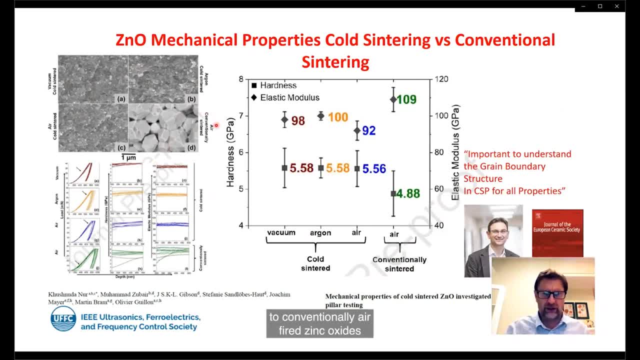 across a number of different conditions And of course, we have in the lab looking at the different conditions and making comparisons to conventionally air-fired zinc oxide. Zinc oxide is obviously becoming a model system after our original work And what was concluded is that if you get the grain boundaries correct and you understand, 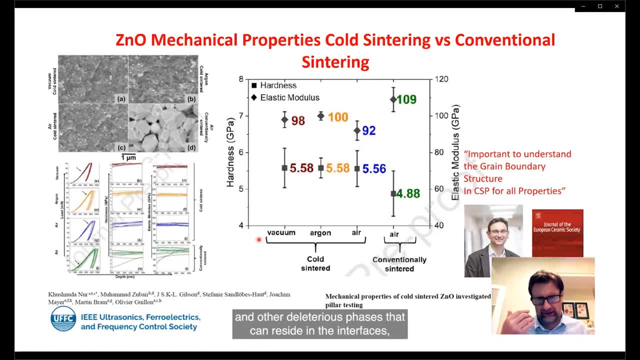 the decomposition of, say, zinc acetate materials and other deleterious phases that can reside in the interfaces, then you might be able to get a lot of different results. So that's a good example of the problem. Thank you, Thank you. 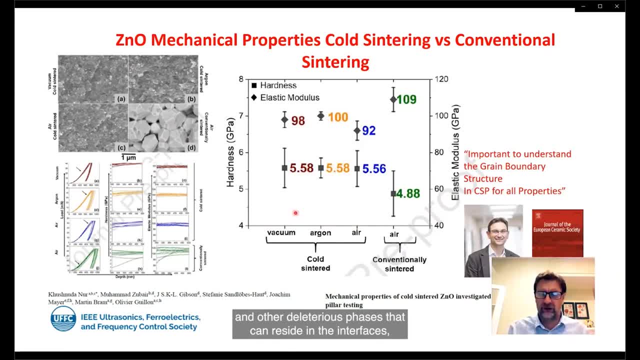 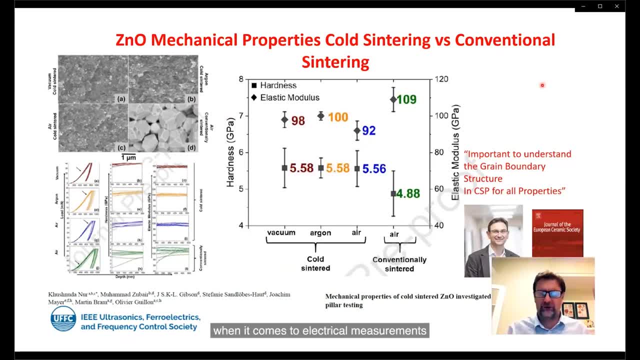 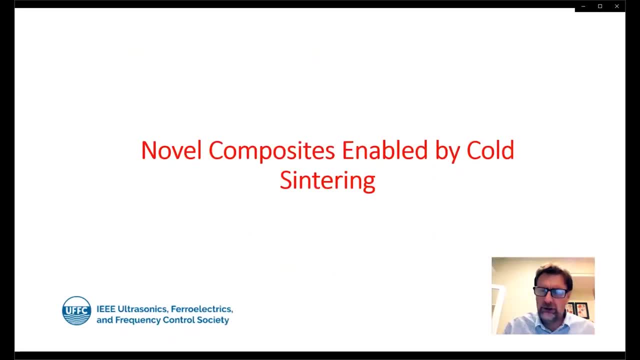 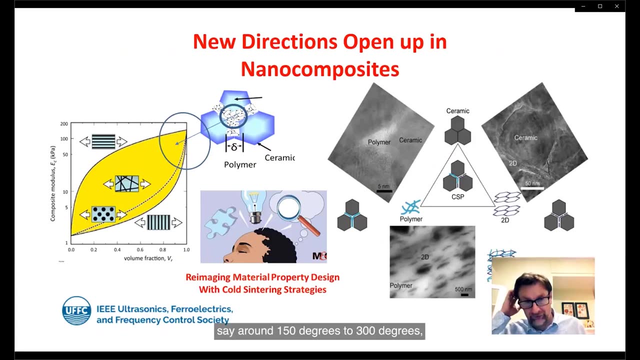 And we've seen this also in our own properties when it comes to electrical measurements such as conductivity. In the case of zinc oxide, you've got to get rid of the zinc acetate. Okay, so when you bring sintering temperatures down to temperatures, say, around 150 degrees to 300 degrees, 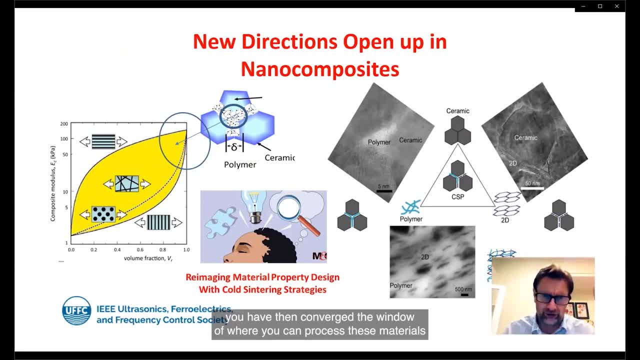 you have then converged the window of where you can process these materials with other materials, including polymers, And so now the door opens to then designing really interesting types of new types of composites, And we are particularly interested in nanocomposites, Where phases can be added to grain boundaries in such a way that you're really redesigning the grain boundary characteristics of a particular material. 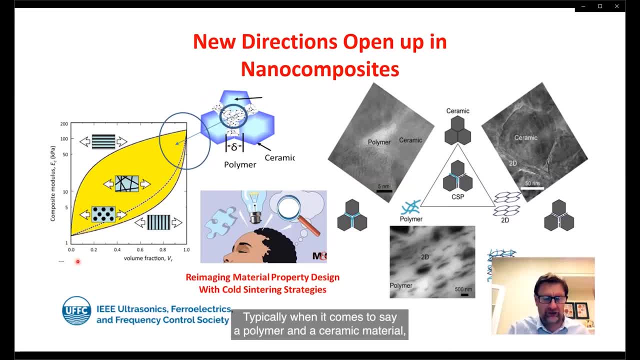 Typically, when it comes to, say, a polymer and a ceramic material, we are typically adding filler materials, But it becomes very difficult to get a high density of ceramic material, for example, into such a composite. So most of the composites are limited to the perculation level, which is about 60% by the volume of the ceramic material. 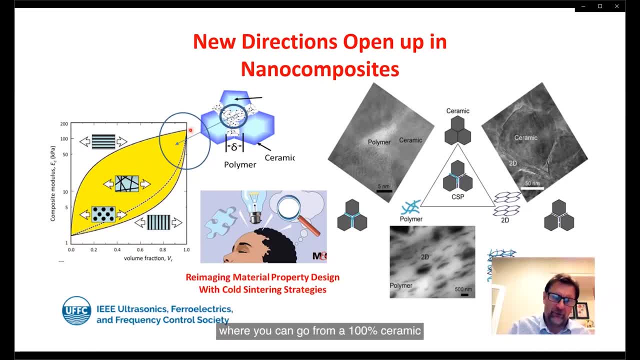 In the case of cold sintering, we are considering it the other way, where you can go from 100% ceramic down to up to say, 30% polymer into the system And the polymer is confined into thicknesses of around 1 to 10 nanometers in thickness. 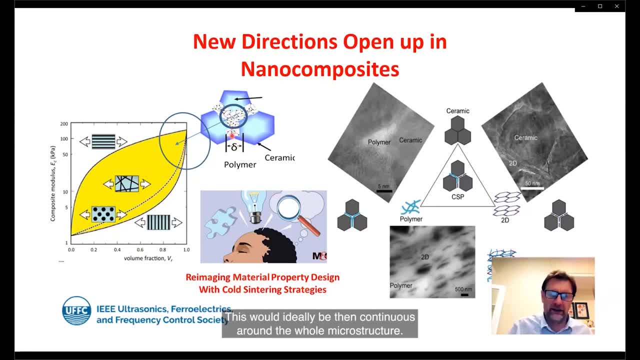 each of the respective grains, and this would ideally be then continuous around the whole microstructure, and we've also been able to add 2d materials into the grain boundaries of such materials. so, in terms of building composites, and in fact, there's been tremendous work, as you may. 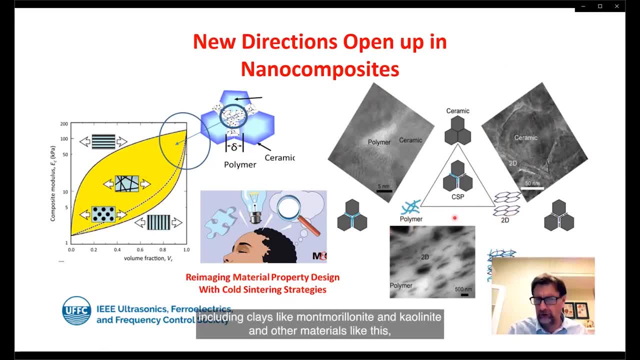 all well know. in terms of combining polymers with 2d materials, including clays like monorite and kaolinite and other materials like this, then this has really been the focus over the last probably 25 years. in terms of nanocomposites, when you're using particulate materials and polymers, 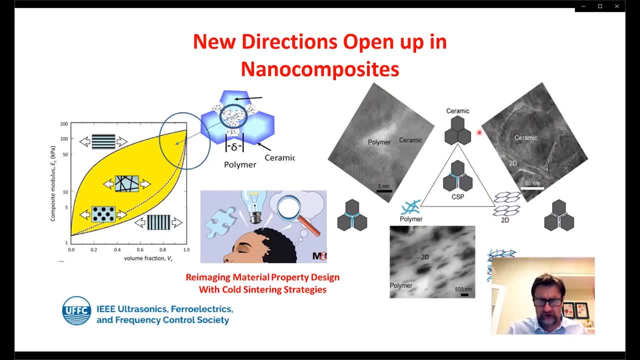 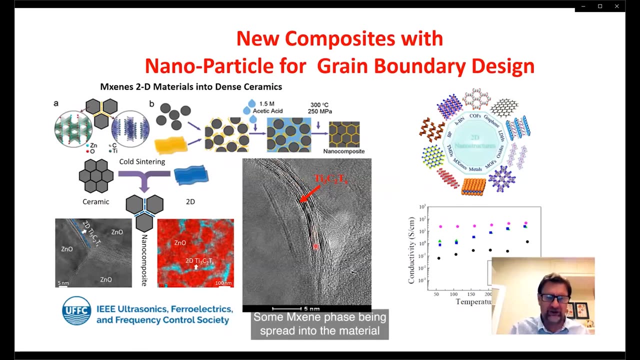 but now we think that this opens up a completely new space and allows you to then have a lot more variation between the way you design grain boundaries. here's an example of a 2d material being put into a zinc oxide material. it's a maxine phase being spread into the material to 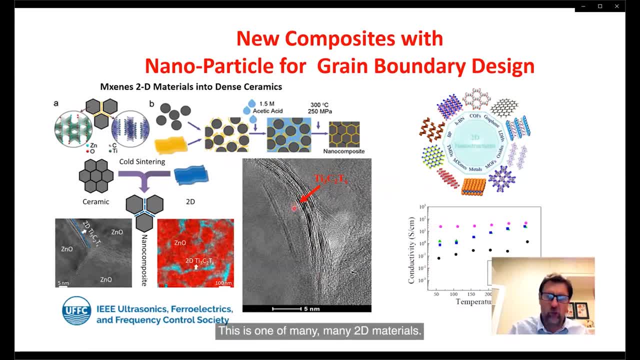 haunt the overall electrical conductivity. but this is one of many, many 2d materials. this can be hexagonal boron nitride for thermal conducting purposes. it can be a moth material for, say, chemical catalysis or chemical sensing. many, many different types of materials can all 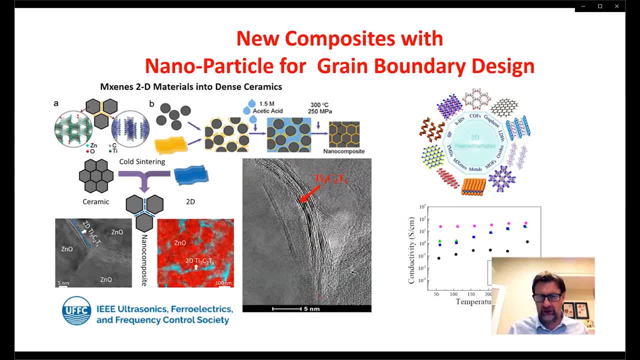 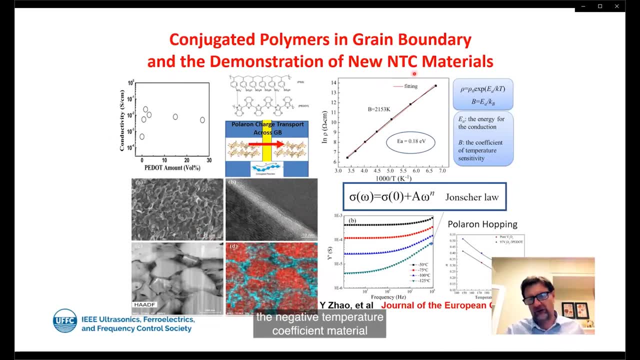 be incorporated into the grain boundaries of a densified microstructure. here's an example of making a semiconductor and a negative temperature coefficient material and so-called ntc material, of where we enhance the electrical conductivity in vanadium oxide by adding a conjugated polymer such as pdot into the green boundaries. here you can see about a 10 nanometer. 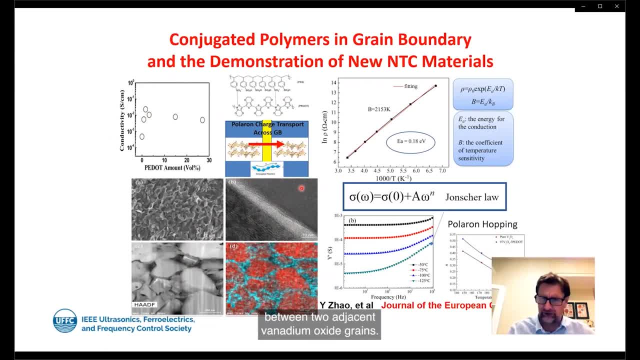 layer of pdot between two adjacent vanadium oxide greens, and this led to very attractive ntc type and essentially what we were doing in terms of conduction. the vanadium oxide has polaron conduction and so so does the conjugated polymer, so we essentially were teasing the conjugated 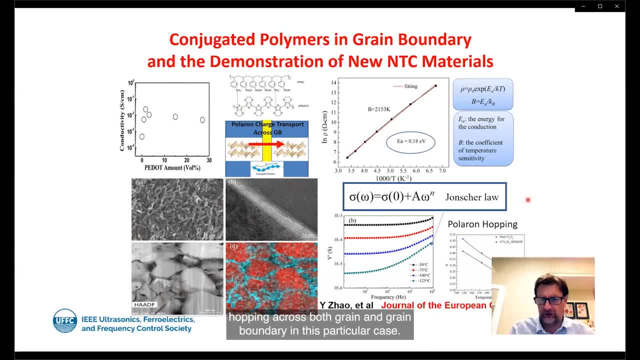 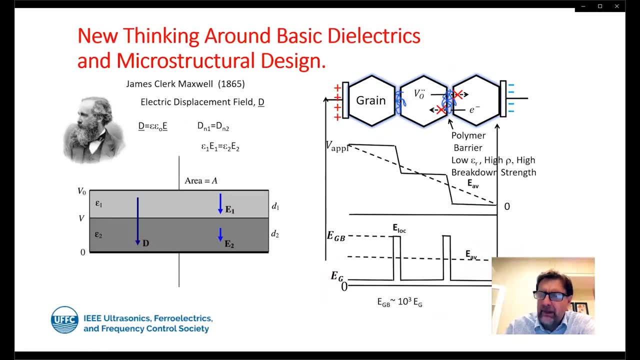 polaron, hopping across both grain and grain boundary in this particular case. okay, let's get back to dielectrics and ferroelectric materials. um, what we're trying to do in the case of making new types of capacitors is thinking about taking high permutivity materials to a subcontractor, or another type of capacitor or other type of capacitor. 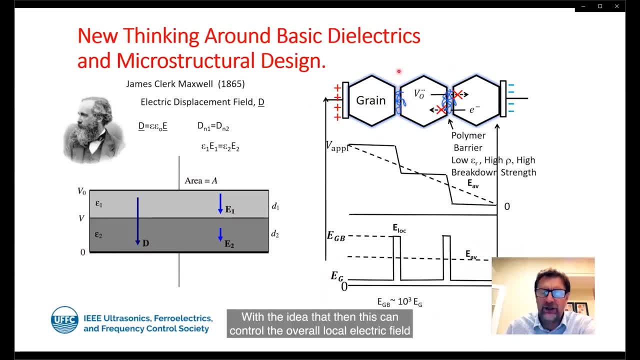 materials with a low permittivity grain boundary, with the idea that then this can control the overall local electric field and you're no longer just considering the average electric field that you're applying across a microstructure. so it was James Kirk Maxwell in 1865 that introduced to us 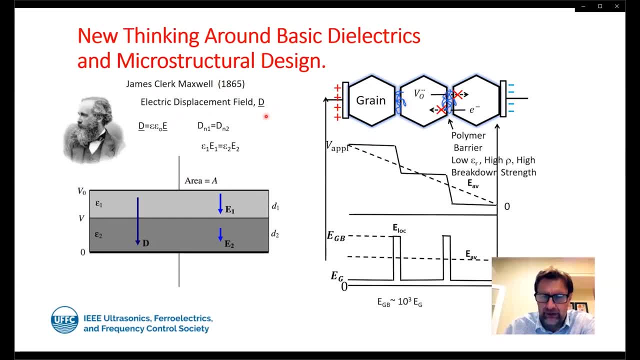 the electrical displacement field and he pointed out one of the boundary conditions for this with two adjacent dielectric materials is that the normal of that displacement field is constant across two dielectric media of permittivity, epsilon one and epsilon two. but the magnitudes of the field change in accordance to the constant of the normal displacement field. 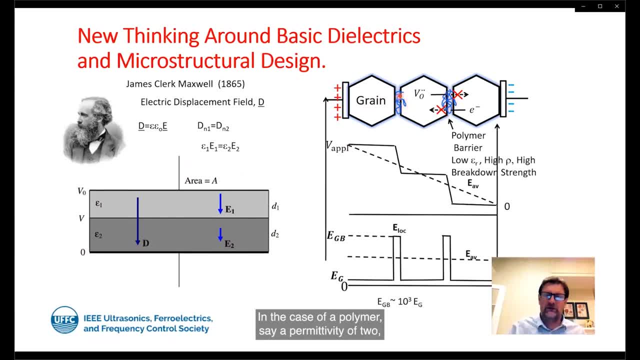 so in the case of a polymer, say, a permittivity of two, a barium titanate, say, a permittivity of 2000, then the electric field will be enhanced by essentially a thousand times. in the green boundary region that offers a lot of opportunities. 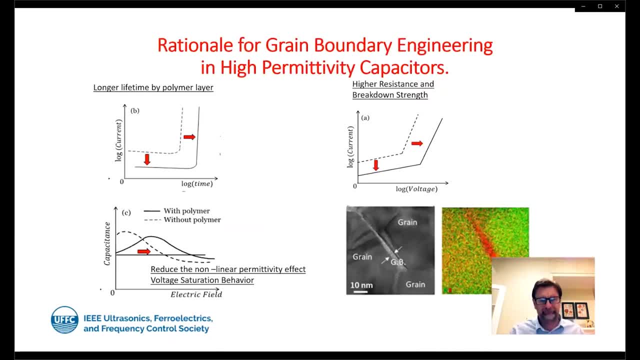 now we can enable this type of process with. first of all, it allows us to then reduce the overall insulation current and also improves the overall non-linear processes and wear out processes that can occur. it also can enhance the breakdown strength and in terms of non-linearities you apply. 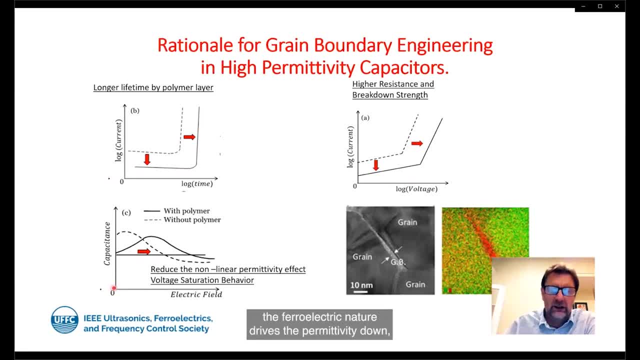 more and more field to a non-linear material. the ferroelectric nature drives the permittivity down. this is so-called the multi-saturation effect. you can you can suppress that, because now the field is much more focused in the green boundary regions. here's some of the microstructures. this is a case of teflon in a barium titanate ceramic. 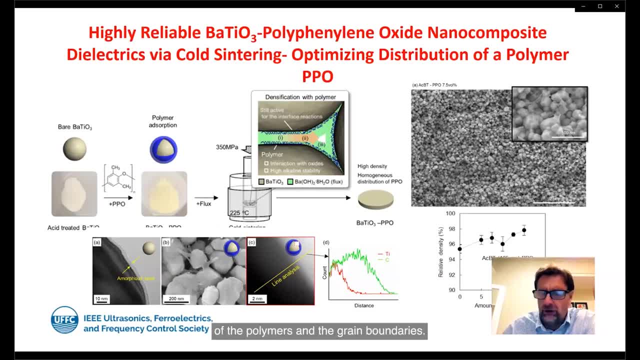 there are various ways to enhance the overall distribution of the polymers in the grain boundaries and i will emphasize to you that it is very important to make sure that that is maximized in terms of the uniformity of this polymer for the best results that i will be. 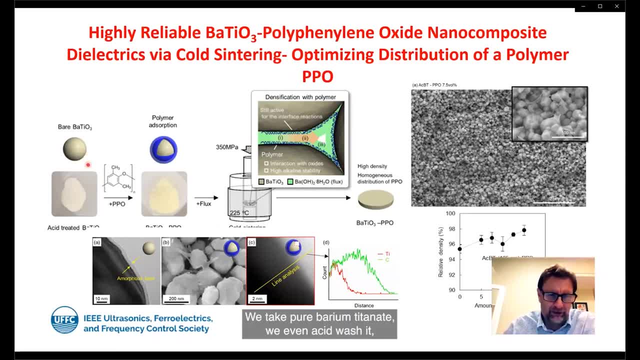 showing below um. so we take a pure barium titanate, we even acid wash it, we absorb polymers to the grain boundary and then we add the overall transient phase, the barium hydroxide high rate, and then center the material after very good mixing and then you can see we get densities. 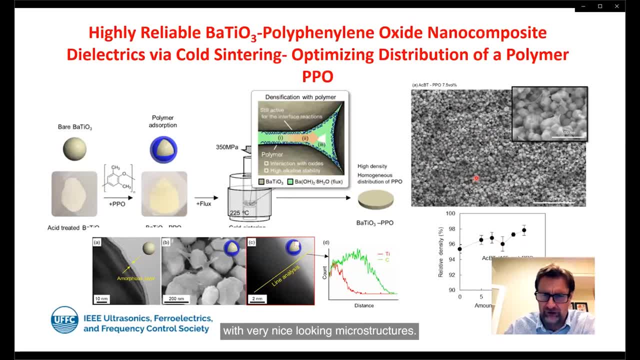 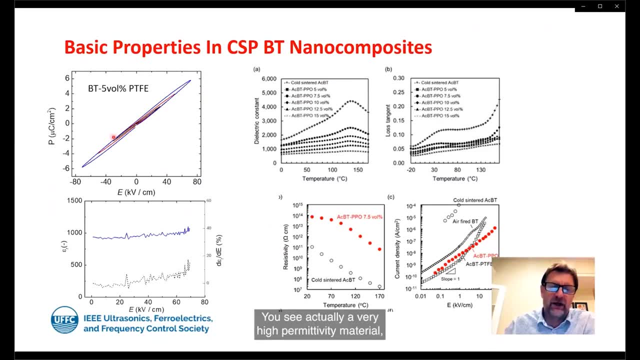 above 96, dense with very nice looking microstructures. okay, and what you see for properties? you see actually a very high permittivity material now behaving like a linear material. you see that, a permittivity of about a thousand in this particular case, going out to fields way beyond the coercive field. you see permittivities. 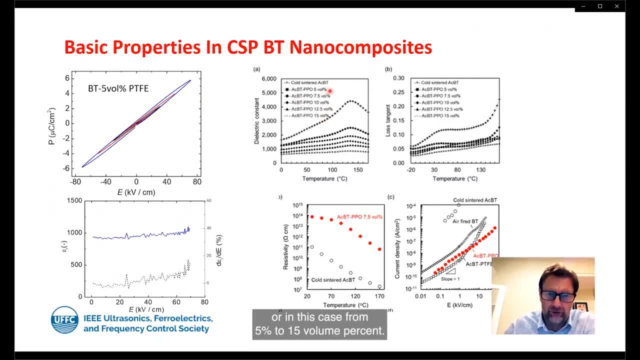 um, varying with the amount of polymer that you've got in it, or in this case, from five percent to 15 volume percent and you can see the see that the electric are normally becoming washed out, but still still around a thousand degrees permittivity, a thousand permittivity over. 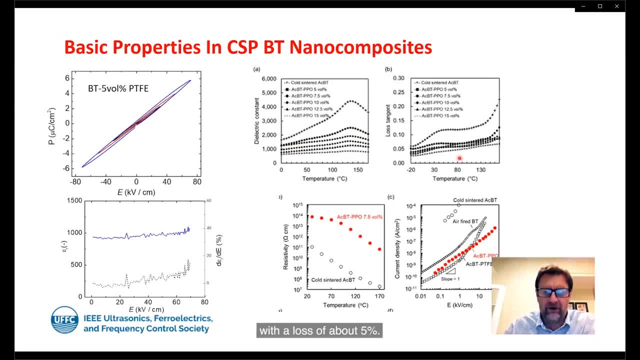 a broad temperature range window with a loss of about five percent. you can see the resistivity jumps to about 10, to the 14 ohm centimeters and you can also see the advantage of these red dot so that remaining ohmic and not being taken off with the non-omic conduction of the typical. 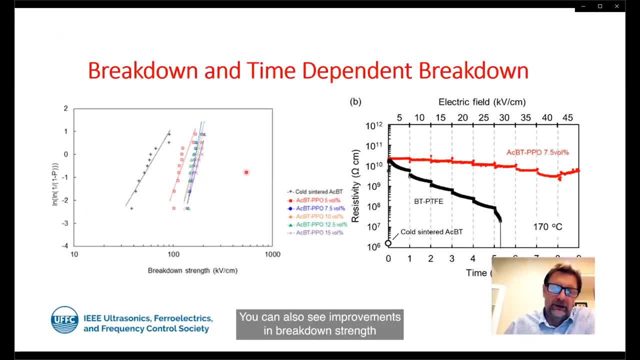 ferroelectric material. you can also see improvements in breakdown strength and in the so-called time-dependent breakdown, where oxygen vacancies can migrate and pile up at the cathode electrode and then limit the overall um resistance of the material as a function of time and field and temperature. and you can see here now, we believe, to be stopping those. 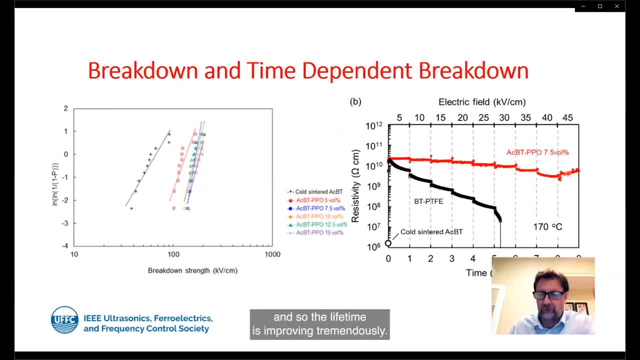 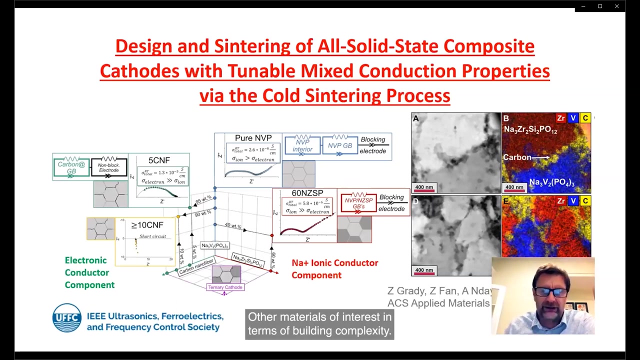 migrations at the individual grain boundaries, and so the lifetime is improving um tremendously. these are very, very early results, but i think it shows you that we are on the path to really rethink how to design dielectric materials for high permittivity capacity, other materials of interest, um in terms of building complexity, um say we're taking here a cathode for an all solid state. 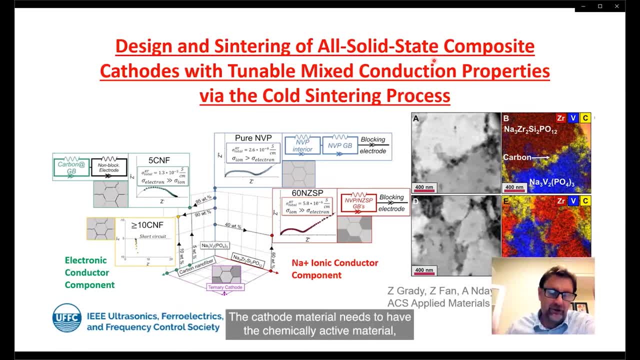 of battery material. um. cathode material needs to have the chemically active material, it needs to be able to undergo the redox reactions, but it also needs to have pathways of having the ions- the appropriate ions move backwards and forwards to shuttle from anode to cathode through the 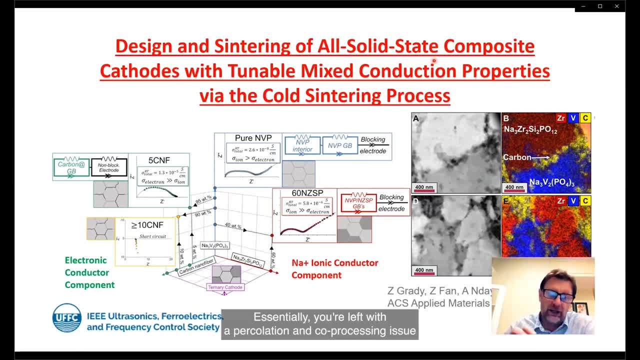 electrolyte. so essentially, you're left with a percolation and co-processing issue to then maximize the distribution of each of these functions: the electroactivity of, say, in this particular case, the sodium bannanate phosphate, the ionic conduction of the nasa corn and the electronic conduction being managed by the carbon. 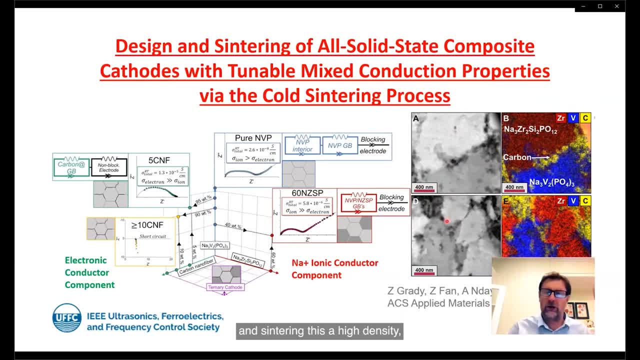 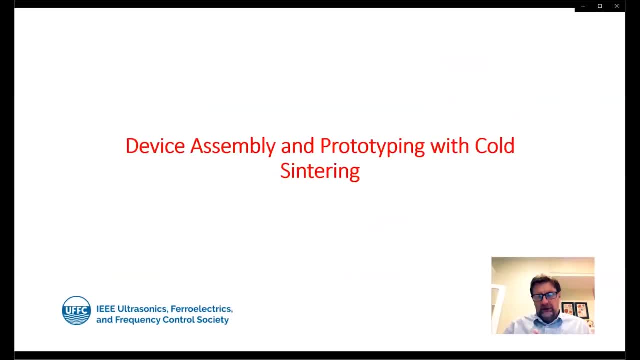 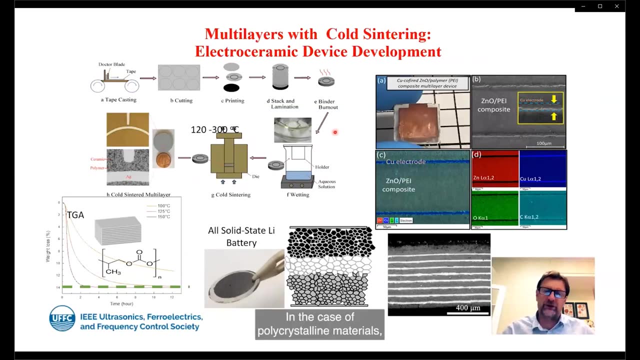 and here you can see us now taking these materials and centering this to a high density, but a high level of functionality for this particular battery application. all right, how about devices? can we make devices? and so, in the case of polycrystalline materials, often they are assembled with thick film technology. 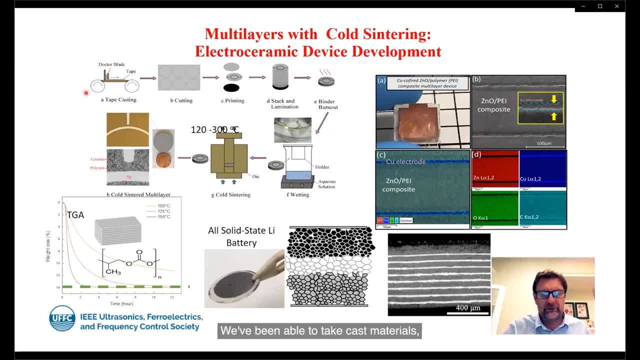 which means screen printing and tape casting. so we've been able to tape cast materials and work with new types of binder systems and add binders, multiple phases, to materials and still center the materials between 120 degrees to 300 degrees. here's an example of a barista. 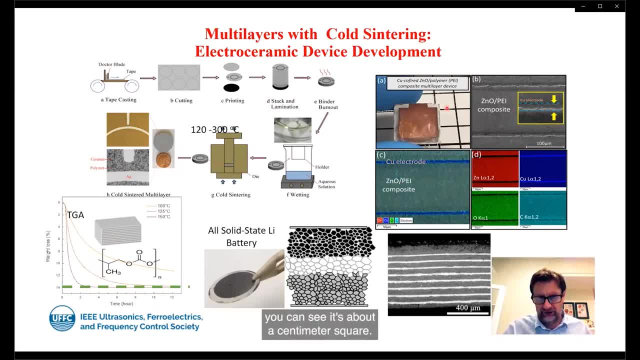 of which you can see there's copper electrodes. you can see it's about a centimeter square. you can tell by the by the luster that it's metallic copper, and here you can see a cross section. and the zinc oxide also has polymer within it as well. 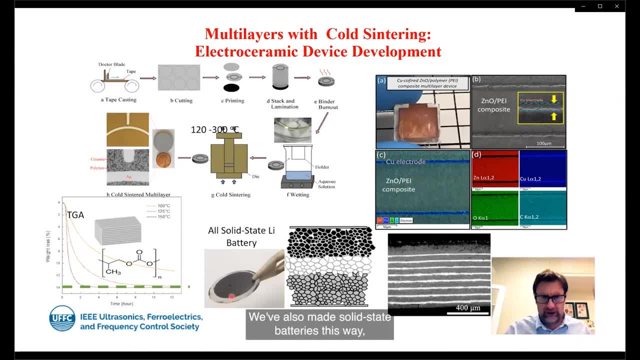 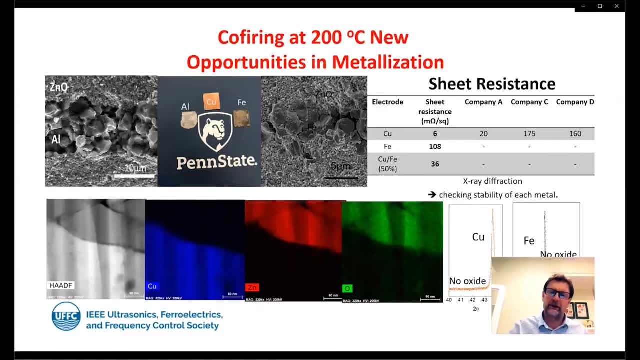 so they make a barista type characteristic. we've also made solid state batteries this way and also multi-layer capacitors this way. um, it opens up a whole bunch of chemistries that you can now address. for the electrodes, typically you use silver or copper or gold or platinum or other types of highly conductive. 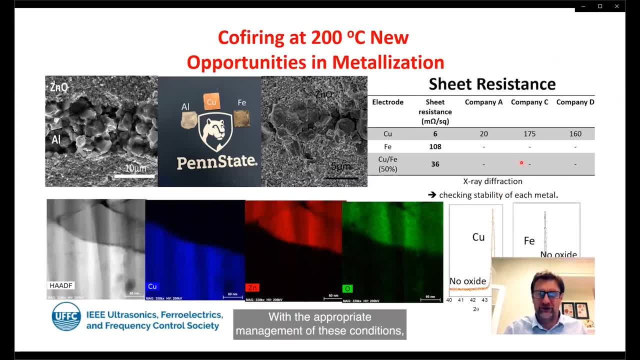 materials. but with the appropriate management of these conditions you can actually use much cheaper or or alternative metals. so here is just a benchmark against a thick film, some thick film, the. this is the sheet resistance. so it's in um million per square and the best company out there has one. 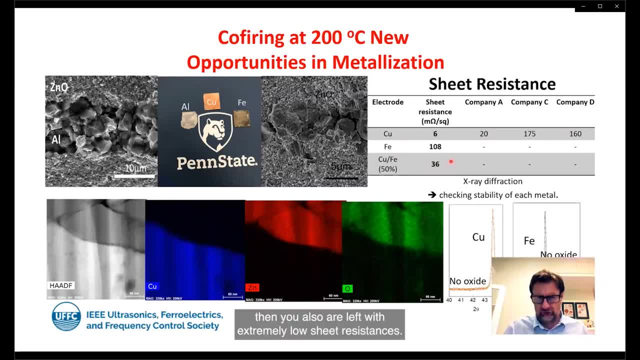 about 20 million per square in our cold cinder. in cases we went down as low as six. and even iron itself would match some of the companies making pure copper. and when you make composites of the copper and the iron together, um, then you also allow the copper to be a little more solid and 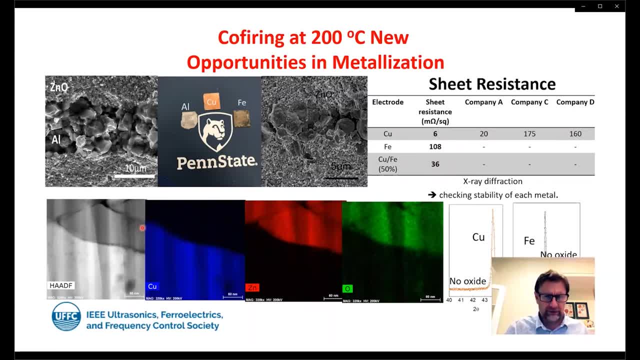 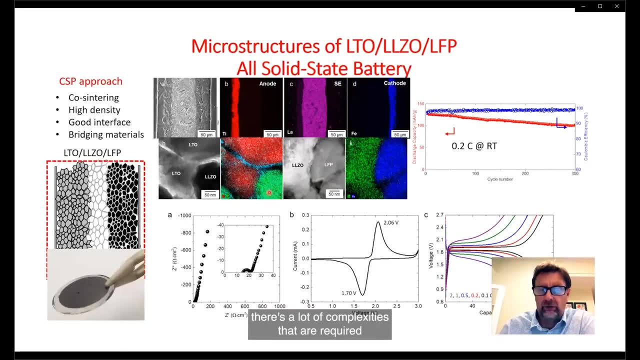 and it's. it's a lot of work to get out of the very thin layer of the metal and then you'll find with extremely low sheet resistances. so there's a lot of opportunities here. when it comes, to, say, a battery for example, there's a lot of complexities that are required to bring the anode electrolyte. 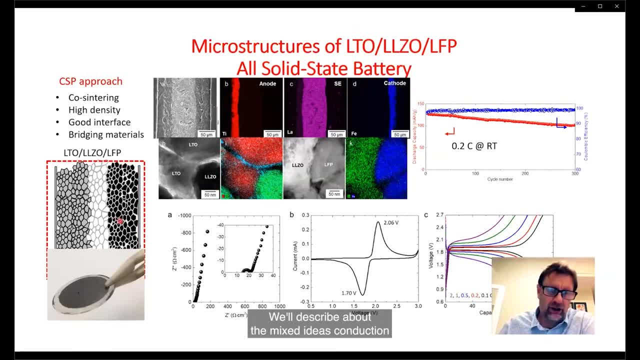 and cathode together. i've already described about the mixed ionics conduction of both the anode and the cathode, then also the interfaces between each of these respective phases is also important. so the ability to co-sinter to high densities with good interfaces and use other materials that can also withstand. 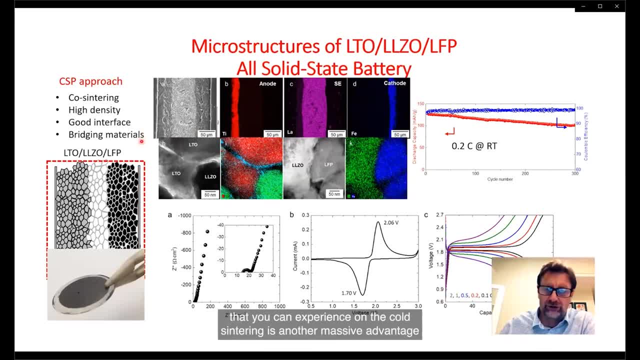 the densification conditions that you can experience on a cold sintering is another massive advantage that we're experiencing with this technology, And so here is an example. the LLZO is a very difficult garnet material to use. This is the lithium titanate material. 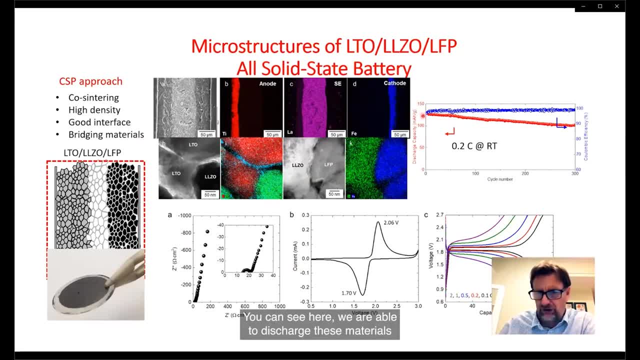 and this is the lithium ion phosphate olivine material, And you can see here. we were able to then discharge these materials over a number of different cycles, and I will also draw your attention to very low insulation resistances because we're able to control the interfaces. 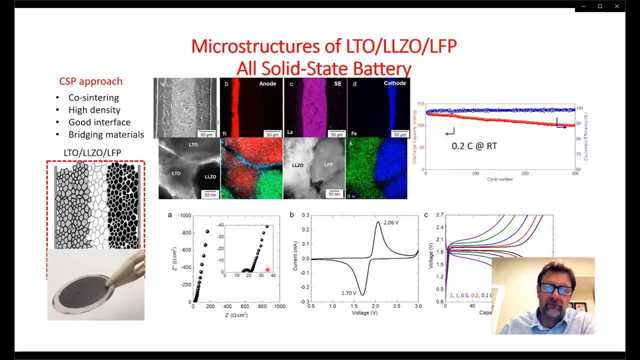 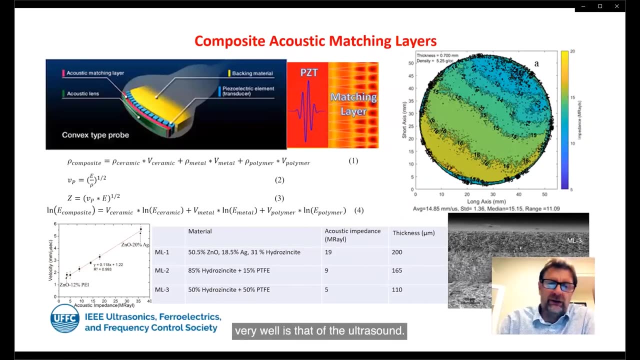 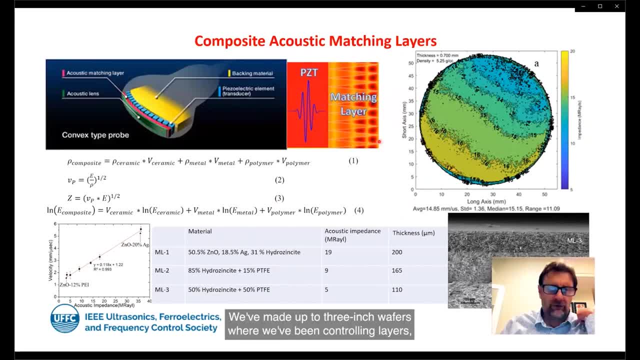 sintering process. So we've made up to three-inch wafers of where we've been controlling layers of different levels of acoustic impedance. So here you can see the uniformity of the system and over here you can see a tri layer being assembled with this particular design for the matching layer. 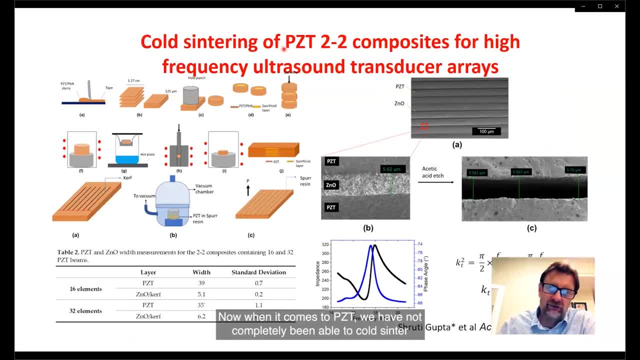 Now, when it comes to PZT, we have not completely been able to cold sinter the material and get great properties at the cold sintering conditions. So in the case of PZT we've had to then take the cold-sintered PZT and take it to higher temperatures. We've reported on this with Srudy's work. 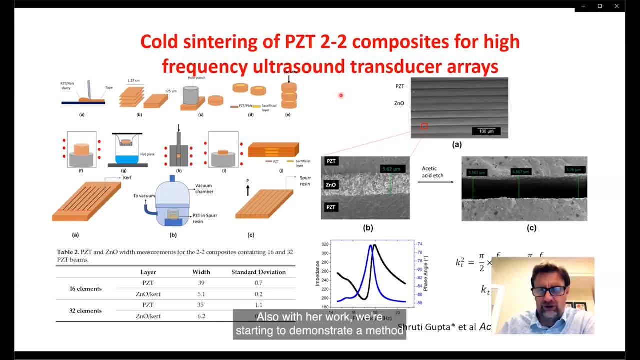 And we've reported on this with Srudy's work, And we've reported on this with Srudy's work, But also with her work- we're starting to demonstrate a method of making very, very interesting 2-2 type composites. 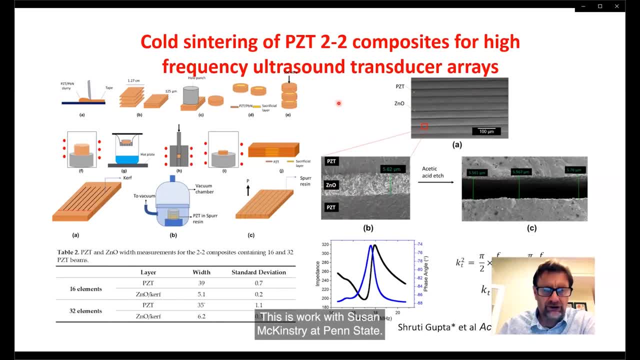 And so this is work with Susan McKinstry at Penn State, And what we've been able to do is to be able to assemble different tapes- PCT tapes and zinc oxide tapes- to then make a multi-layer structure And then coals into this material, heat it to a temperature and then remove later the zinc oxide and then backfill with polymer to then show resonance type behavior. 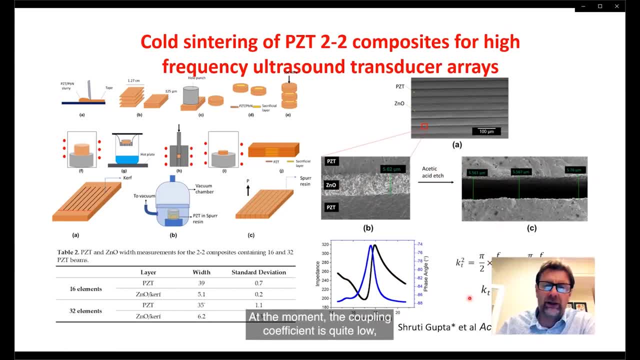 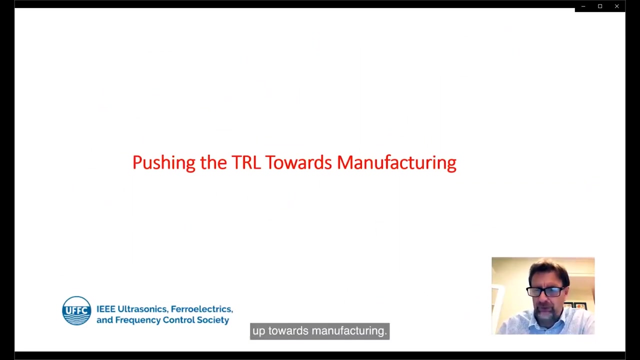 Now. at the moment the coupling coefficient is quite low, but at least this shows you a pathway to making thicknesses of cuts that are previously very, very difficult to do. This is just a first-time demonstration of this technology, So as we look forward, we've got to push the technology readiness level up towards manufacturing. 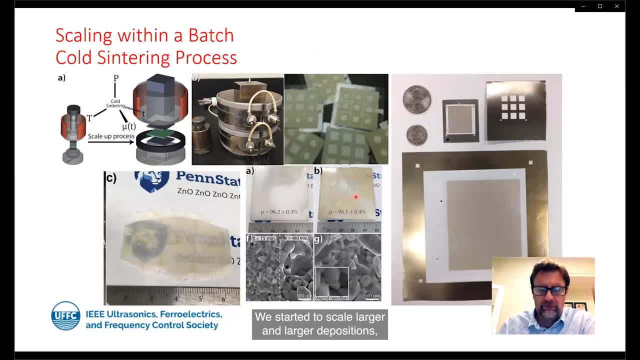 We've started to scale larger and larger depositions, both on polymers and on foils and, in the case of plates, We've also started to look at a continuous process to then make dense ceramics, as you can see by the translucent nature of this particular zinc oxide. 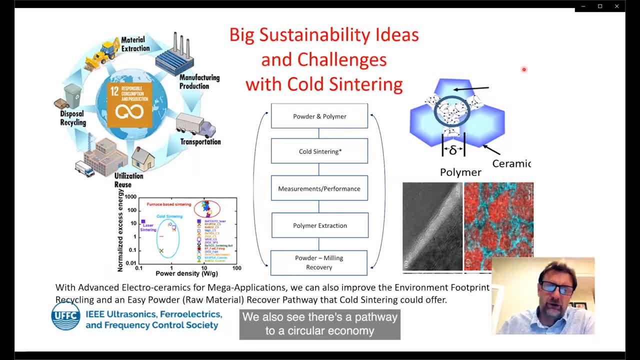 We also see there's a pathway to a circular economy with the coals centering process. The fact that we can make very high performing composites with very small nanometer levels of polymer in them. it gives us the option of then being able to make materials. 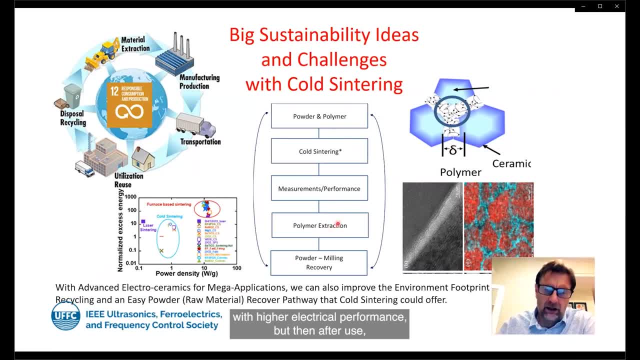 with high electrical performance, but then after use then extract the polymer and then recover the powder and then drive it through the process again. So coals centering is not just about the energy savings and the firing process itself. it may also allow us a way to drive some of the materials in the IEEE. that could help to push the whole process. 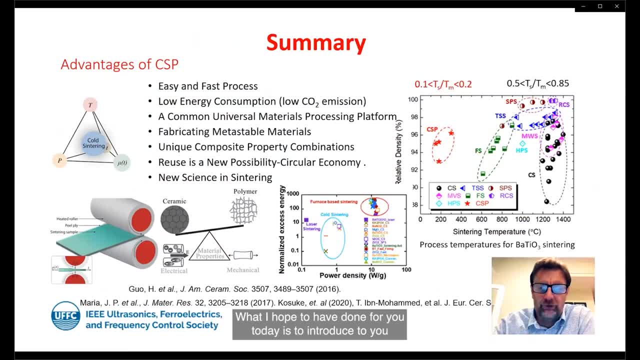 circular economy approach. What I hope to have done for you today is to introduce to you how cold sintering can impact functional electrical ceramic materials. I hope I've pointed out that, at least in principle, once you know the recipes and the appropriate chemistries. 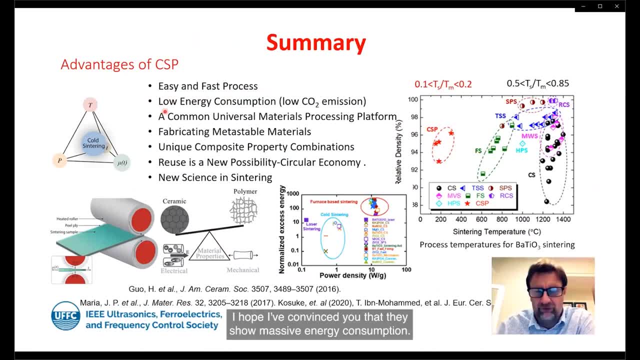 they're easy and fast to process. I hope I've convinced you that they show massive energy consumptions that, if could be scalable, would give us an enormous way of controlling CO2 emissions from these high temperature sintering processes, Because it's a low temperature process. 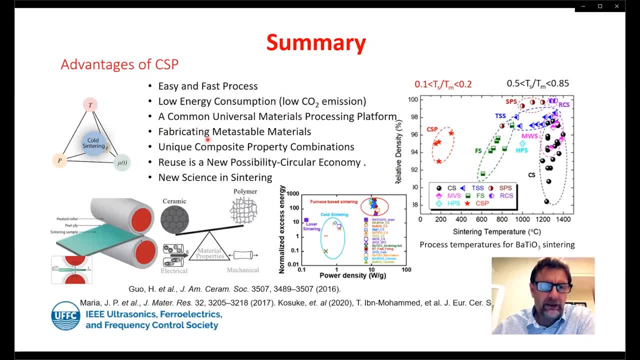 it's also a common and universal processing platform. It allows us to fabricate metastable materials, develop unique types of composites, the reuse aspect for a new possible circular economy, and there's obviously a lot of new science to be done with this particular. 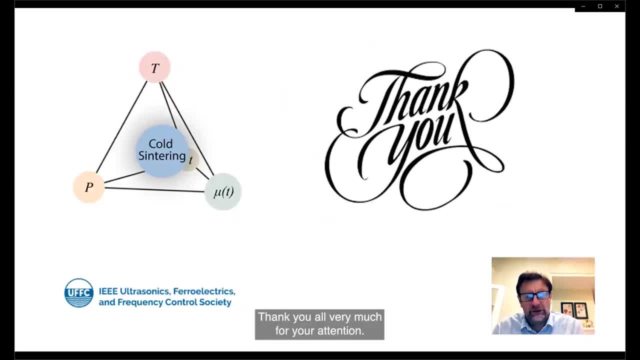 technology. So thank you all very much for your attention. Thank you very much to the organizers for bringing together this distinguished lecture series for the IEEE UFFC and hopefully we'll be able to talk about this in the Q&A section and also be looking forward to seeing people at. 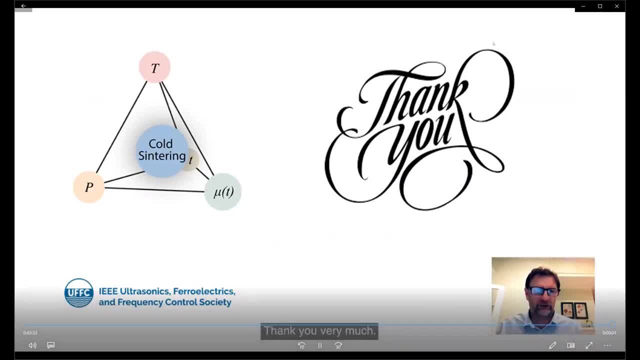 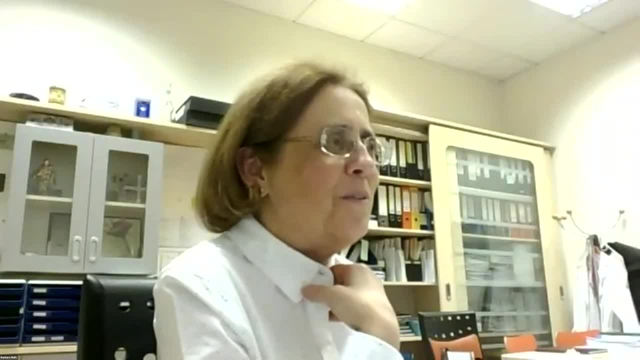 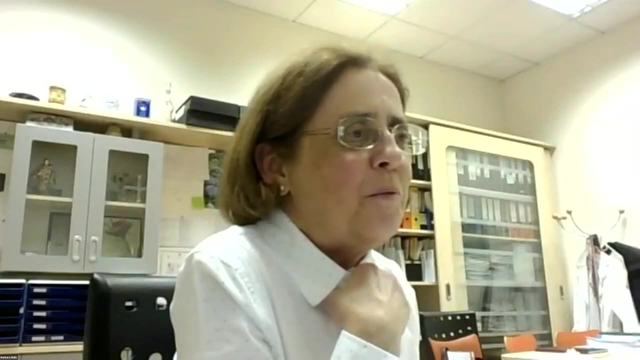 conferences in the next few weeks. Thank you, Thank you very much, Congratulations. Thank you very much, Clive, for this really interesting lecture. There is already the first question in the chat box: When does the dissolution process? Just a minute, It's a long one. 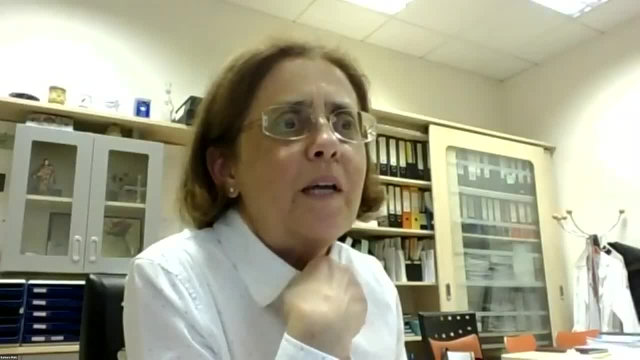 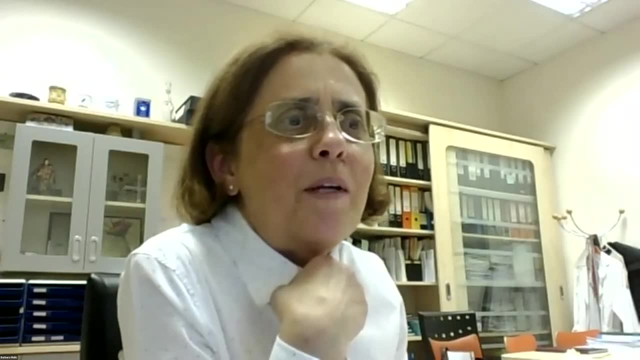 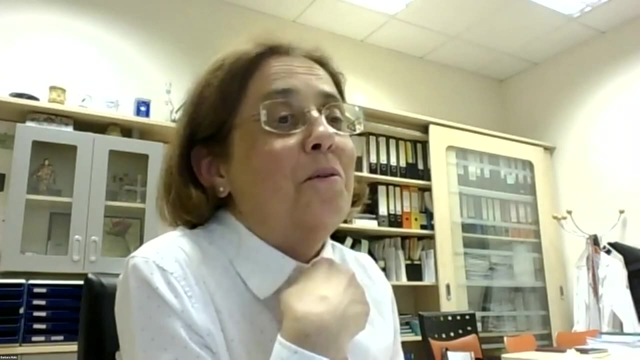 Can you read it? When does the dissolution process in CSP end and when does precipitation and grain growth begin? Same pair of slides. When do you expect saturated grain contact with progressive grain interpenetration? It's a lot of questions. Does it indicate? 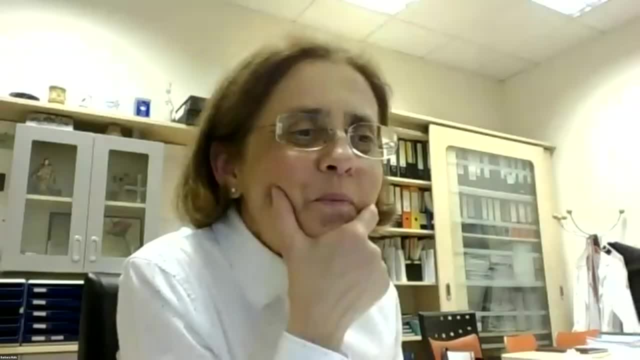 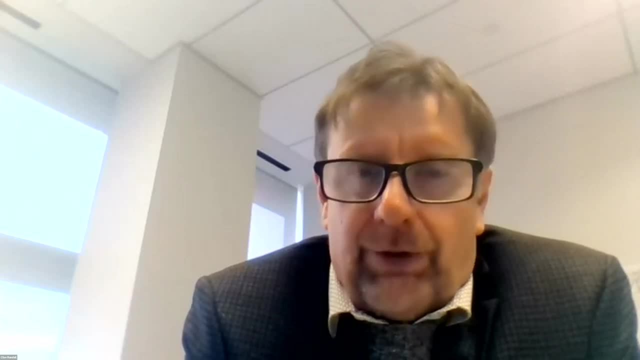 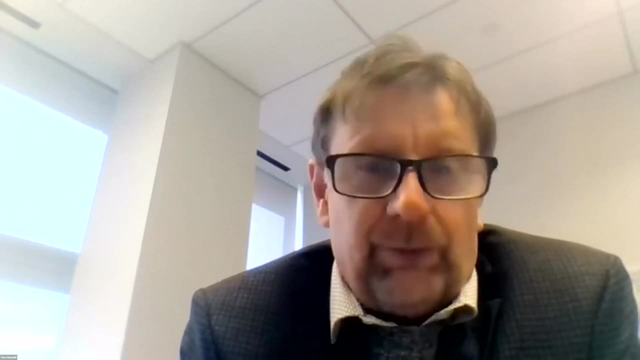 only the dissolution process and no grain growth. So without a doubt, this process favors densification over grain growth compared to other conventional methods. And if you even look at hybrid methods, where we're looking at, you know we're looking at cold sintering with, say, spark plasma sintering, and spark plasma sintering is 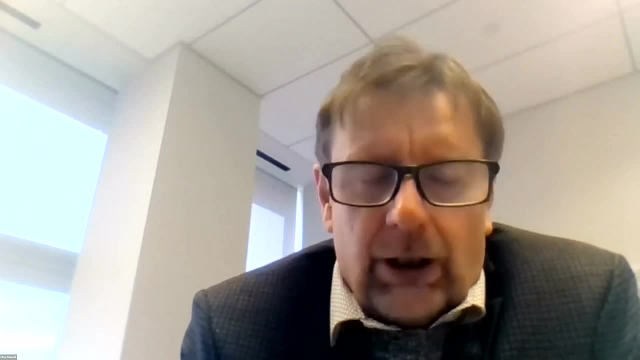 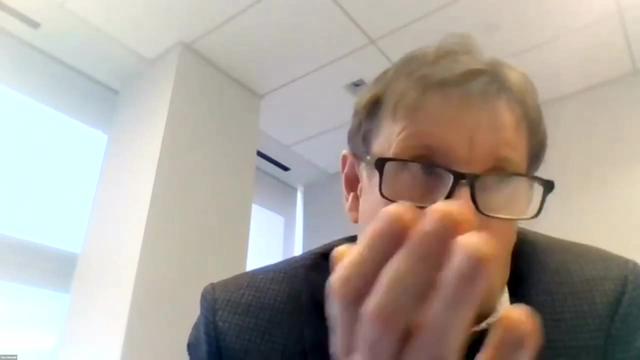 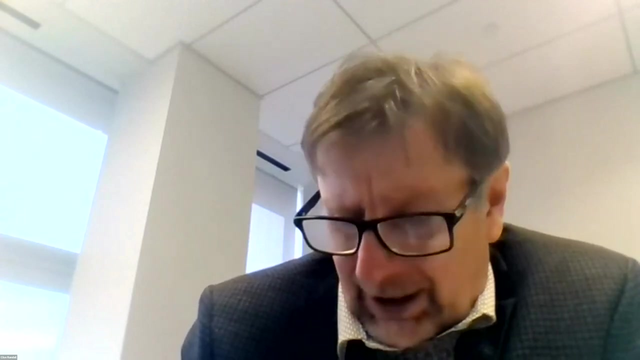 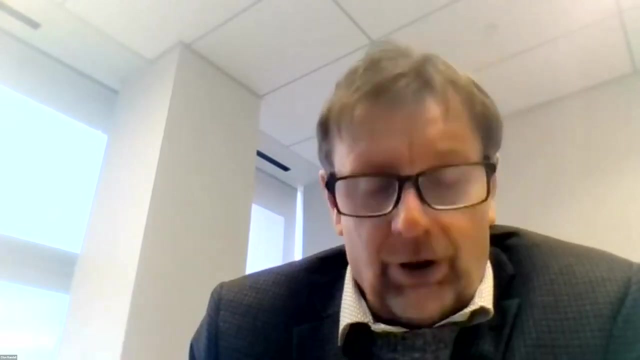 often a good technique to limit grain growth over densification. We still see that that hybrid method has a higher grain growth than in the straight cold sintering case. So yeah, We think that there is a whole series of processes that are linked, always in just traditional sintering we always worry about. 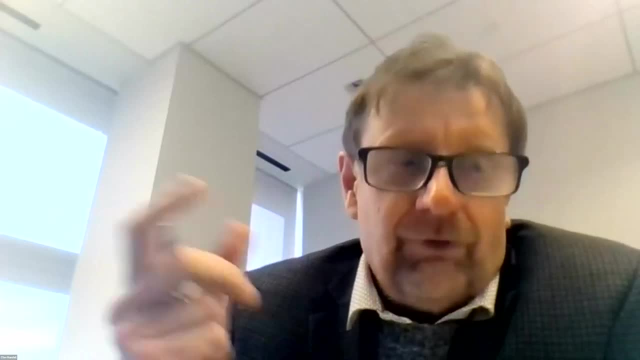 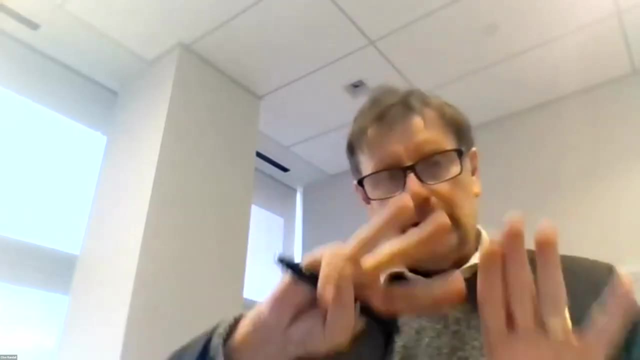 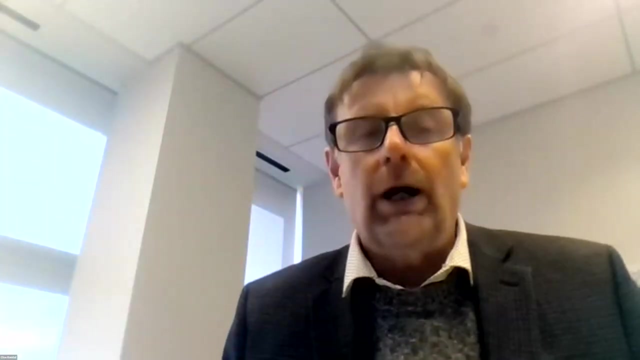 what's happening at the initial parts of sintering, intermediate and final stages. I think the complexity of how each of these rate controlling processes overlap through each of those domains of initial, intermediate and final stages is going to require quite a lot of forensic. 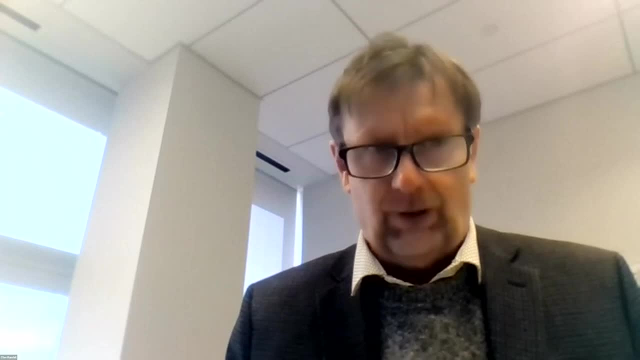 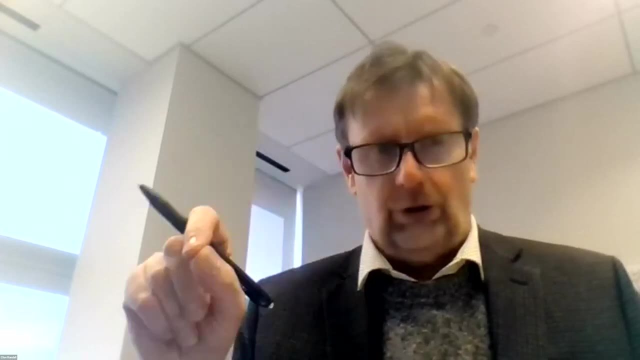 analysis and detailed analysis to be able to answer this question. but based on the question, i can tell that you're already thinking about how these things come on. it's not a simple turn on, turn off. it's how they overlap and how the transience of this all 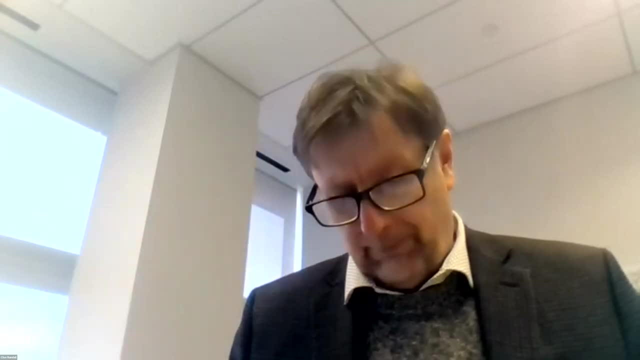 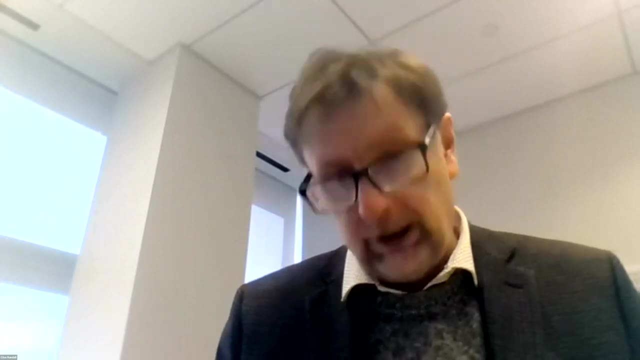 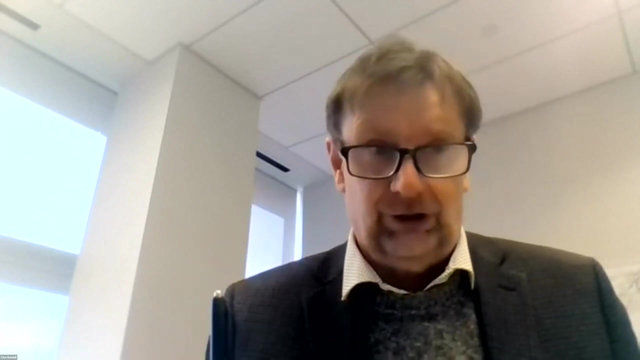 progresses from each of the stages. so, um, this is exactly where the, the understanding of the fundamentals of this need to go, um. so thank you very much for your for your question. i didn't answer it, but i re, i re-enhanced your question by pointing out the complexities of that and how. 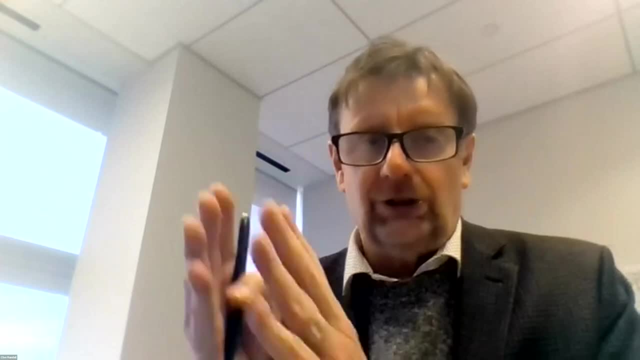 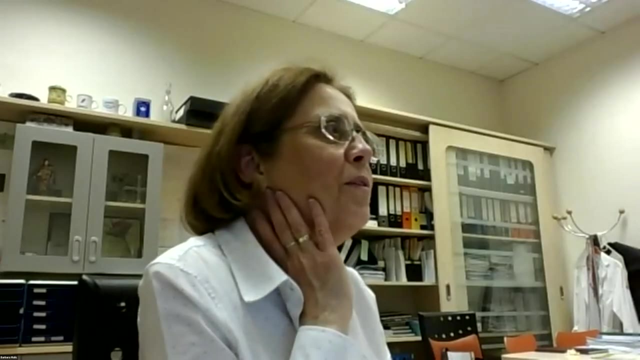 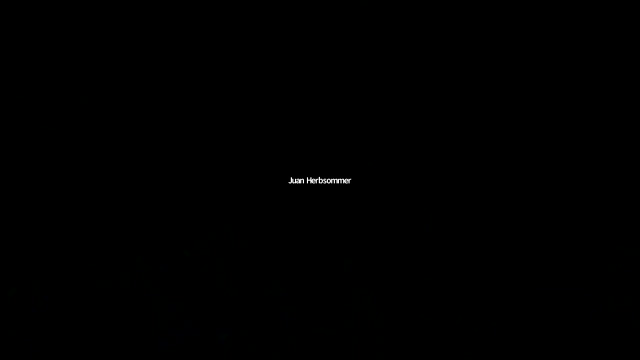 it has been approached in terms of each of these stages of sintering. okay, uh, the i i think that uh, one, herb summer, raised his hand. i i'm not sure if you can speak. yes, can you hear me? yes, very well, thank you. thank you, uh. thank you uh, professor randall. very good. 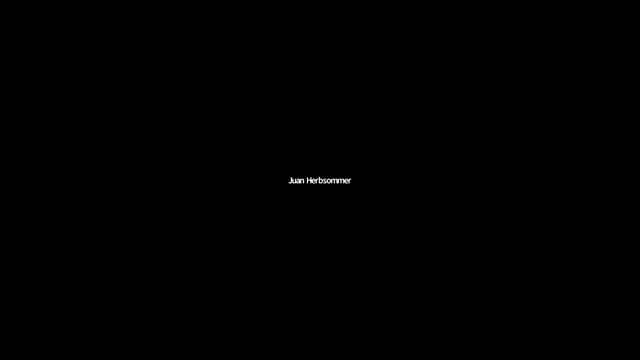 presentation. so, um you know, uh here at the texas instruments, we are uh working towards uh improving some of the uh polymers, uh doping them with nanocomposites, in particular for the application of uh creating uh interconnects for millimeter wave uh communication. okay, so, 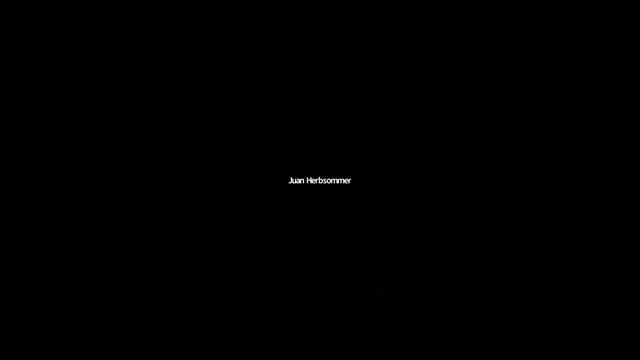 the electric wave guys and uh. we have been using variant titanate as uh as a doping for uh polymers like polypropylene and this type of materials. we optimize the size of the particle. we are right to the conclusion that as you increase the, the doping, okay, you, of course. 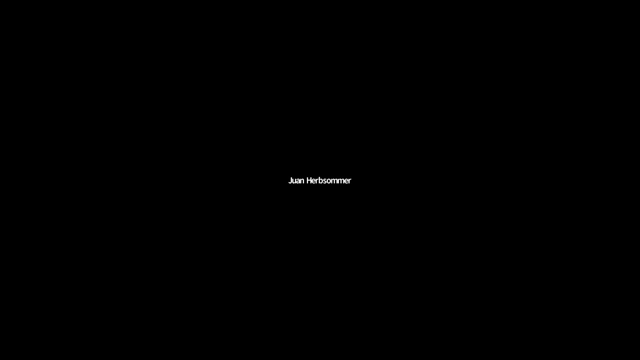 increase that electric constant, and which is what we're looking for. but uh, but essentially, we also find the problem that uh, you became the, the polymer becomes brittle with a really high concentration of uh, nanocomposites. okay, so the question is more in in general, okay, about what's. 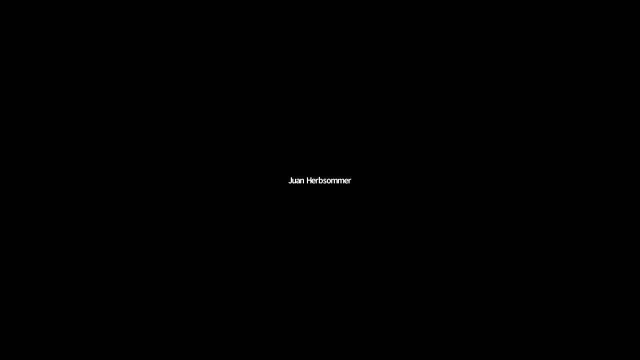 looking at your techniques about co-sintering and how you actually um do some of the things that uh, you know can make you work with nematic and other elements that you have, uh, in the field you know the last talk about in return of composites. okay, 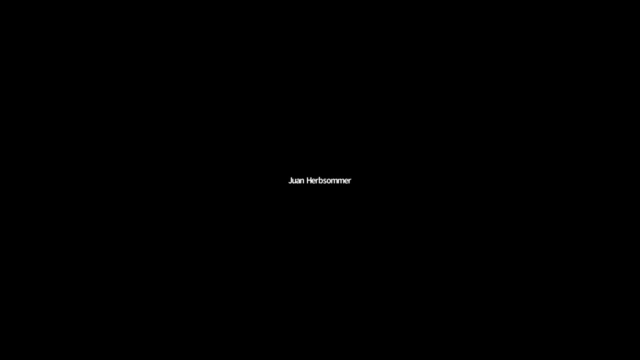 so i think that one of the things that- um, i'm not an expert on the field, of course you know, but uh, one of the things that i've been thinking is: uh, if it is any possibility or any technique available that uh allow us to take advantage of some of the anisotropic properties of this, uh, 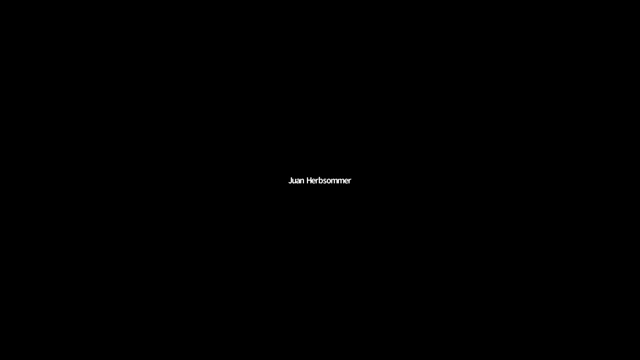 the electric materials- okay, i know that you work with powders and most of the people work with coal sintering- or either the doping of the composite materials. we somehow were able to orient these grains in one particular direction, a preferential direction, such that we could take. 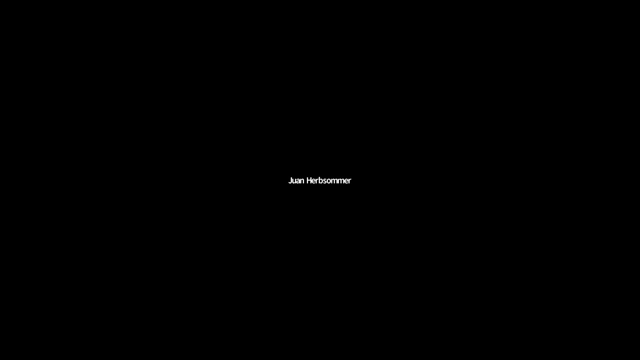 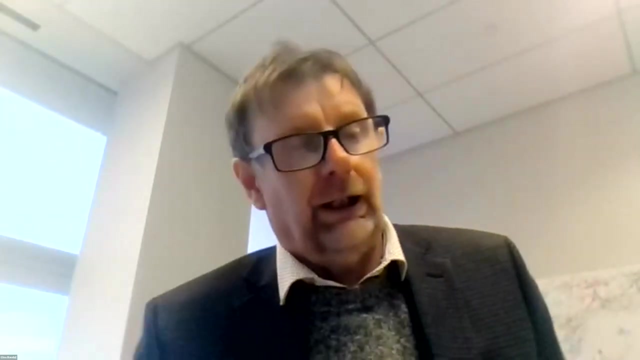 advantage of some of these anisotropic properties and maybe be able to increase, let's say, the electric constants of any material, you know, by orienting properly the grains in one particular direction. Yeah, it's a long question so I will keep it short. So the answer is yes, we are. 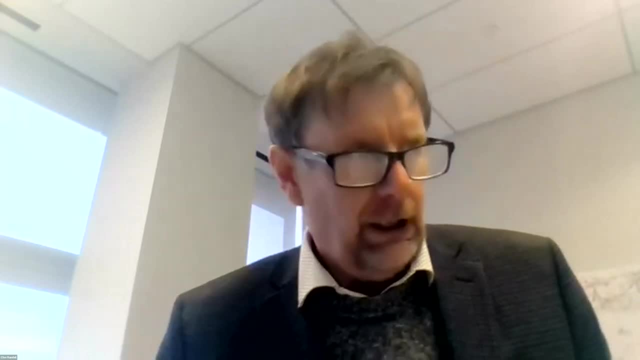 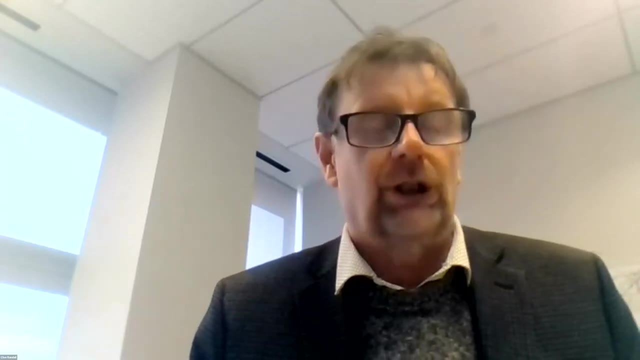 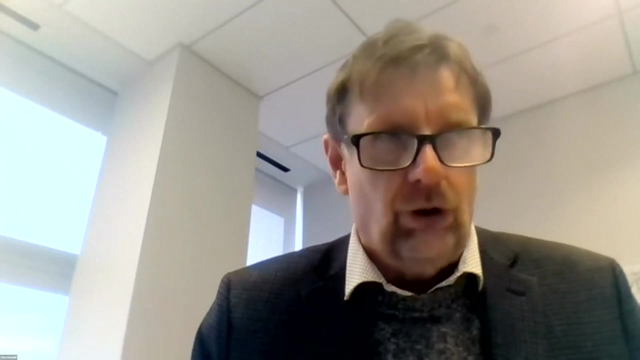 looking at anisotropy, Sometimes it comes for free because we may be working with anisotropic material and at a certain pressure we sometimes see, in the case of zinc oxide, for example, a preferential orientation of the zinc oxide. In other cases you can control the lay down of. 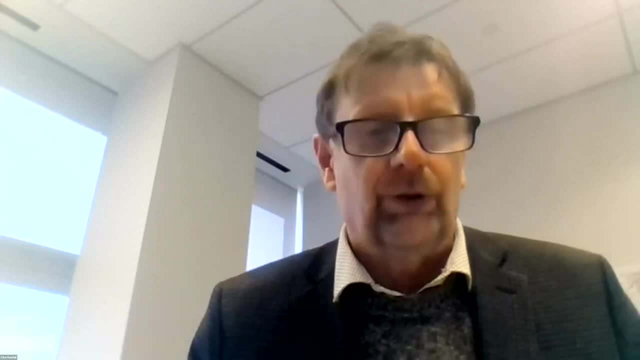 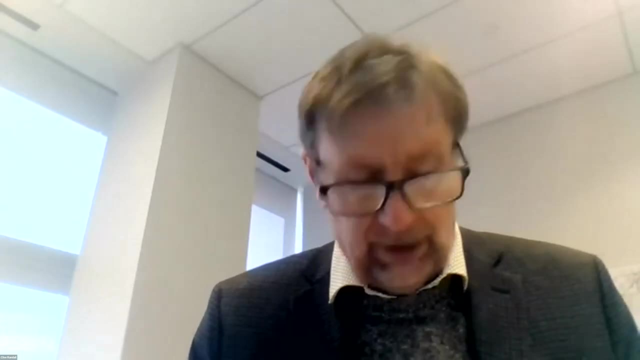 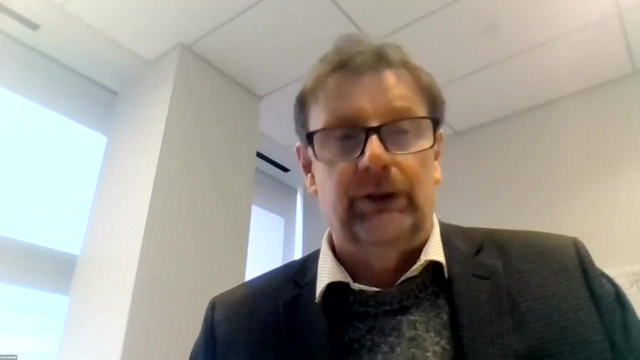 particles In the casting or the pressing process, and so, yes, again, you can control it there In the case of your application. the millimetre wave- we are also looking at that and we think that that's a very, very rich area possibly for this community, and there it's a matter of controlling, not just 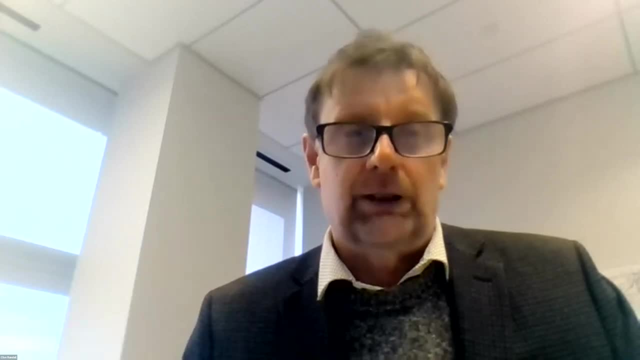 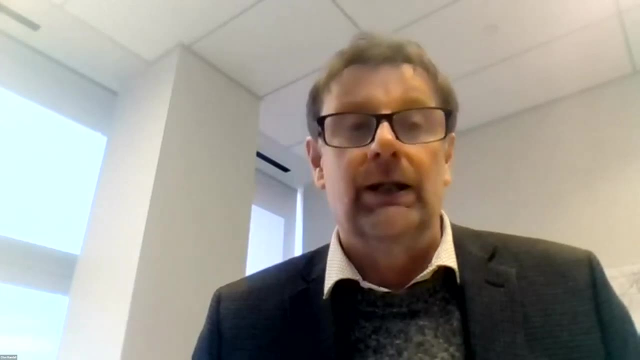 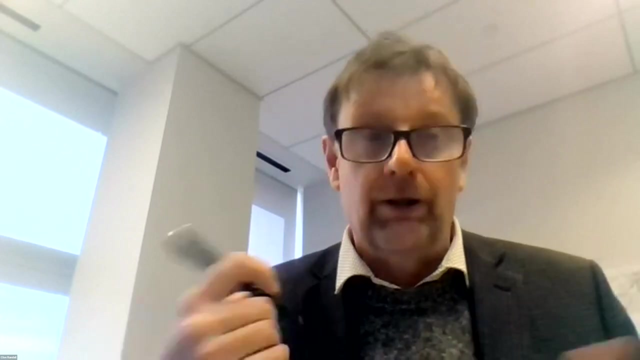 the permittivity but also the thermal properties in many applications, and so we think this is a way of also designing interesting ways of also enhancing the thermal conductivity as well with a composite. So it's another one of the functional elements of the design that can come with cold sintering. So 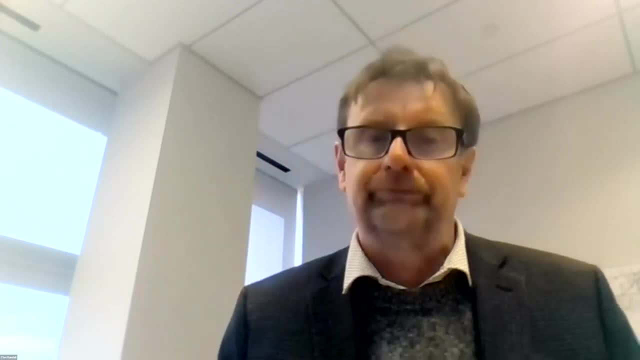 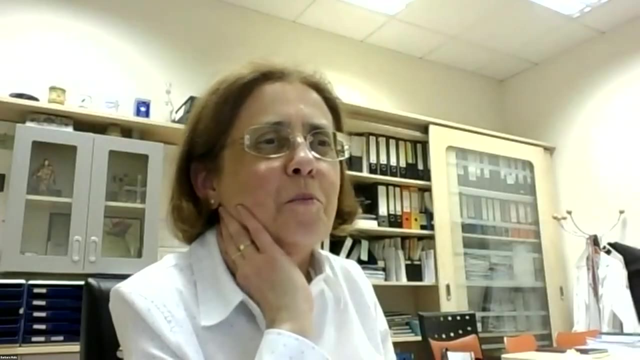 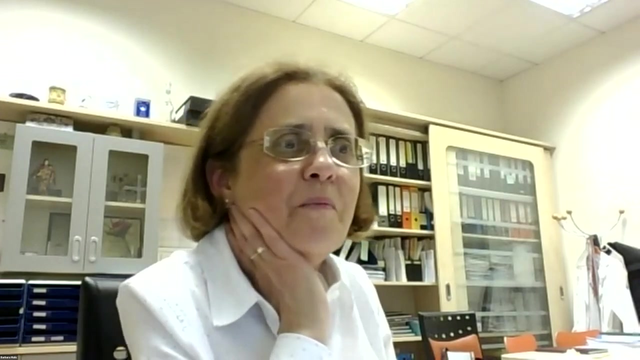 I'd be happy to talk to you about any of those things offline if you need. Okay, so the identity of the first person who asked questions is now known: it was Mojtso Tunica. And now there is another question of James Cockburn. It's when I've tested the insulation resistance of solid-state capacitor samples compared to cold-scented samples. the cold-scented samples always tend to have lower resistance. Is this something that you've noticed and have you got any ideas on overcoming this problem? 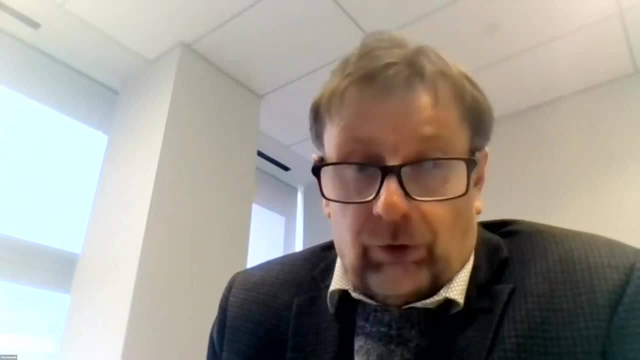 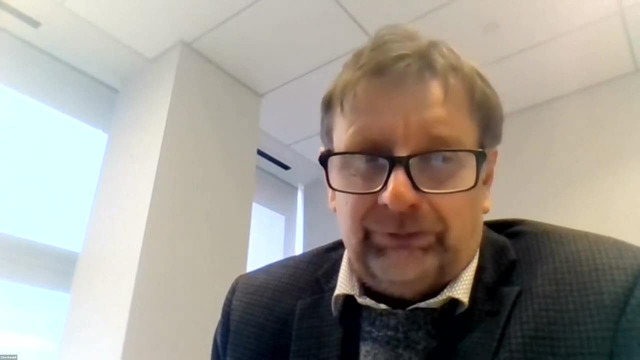 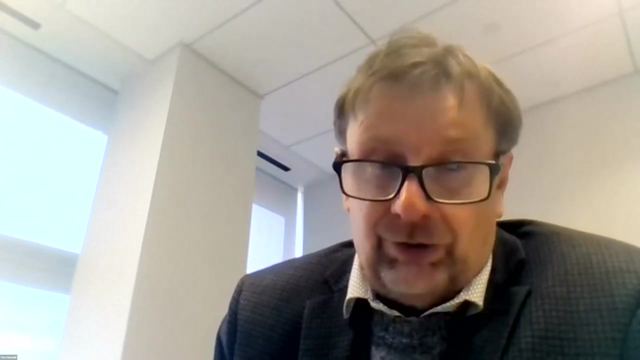 So the answer to that is yes, you've got to be careful about that. Yeah, we can also have insulation resistance problems in cold-scented, But when you're starting to add a polymer to the grain boundaries or you are doing special surface treatments. 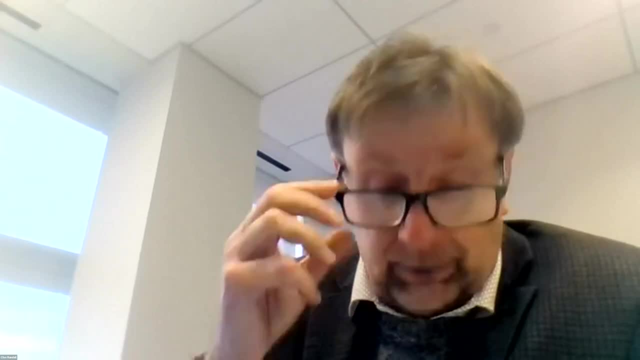 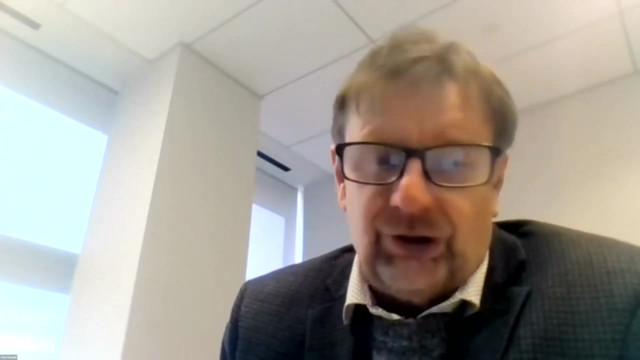 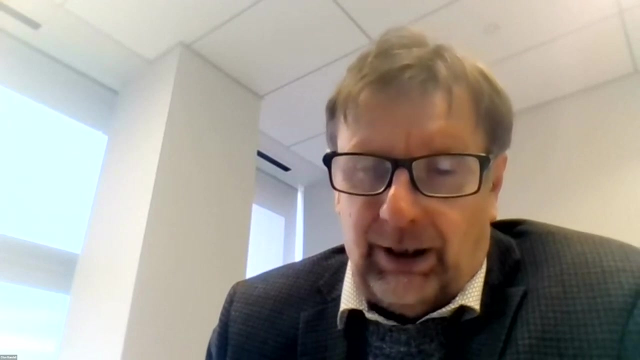 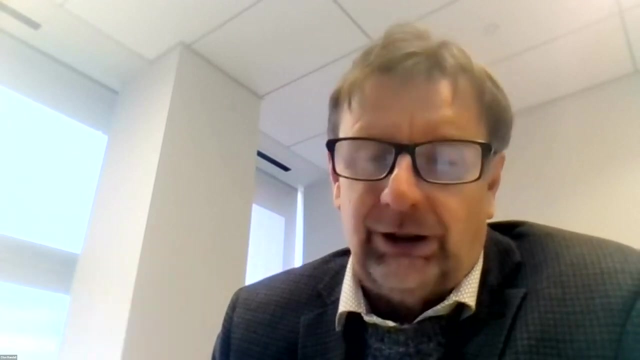 then we are seeing and learning all the time that we can suppress the TAM delta and the conductivity. But very recently one of our visiting scientists from Japan has recently shown me with the KNN that with a certain treatment of the surface he can reduce the TAM delta quite substantially. 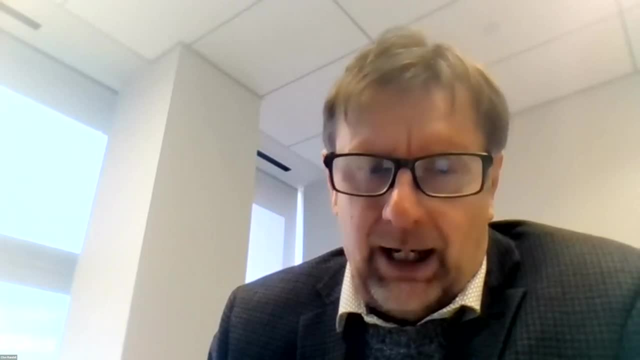 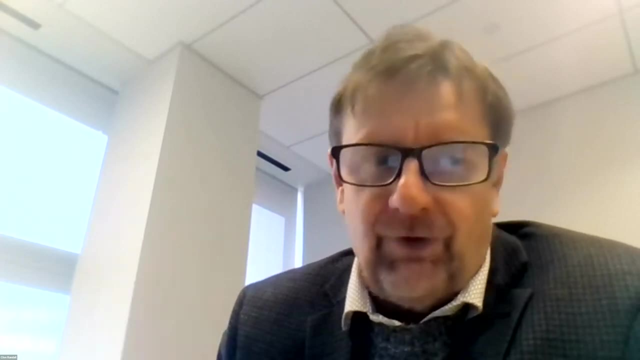 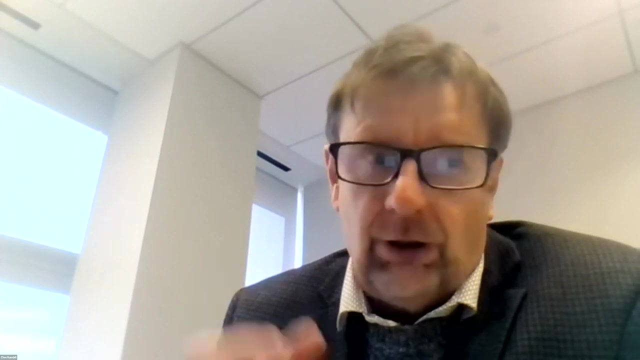 And so I think we're still learning, And the devil is in the details, And this is a very rich area for chemists. That's why I love the fact that Barbara is involved in this type of thinking, because you need a heck of a lot of knowledge on not just ceramics. 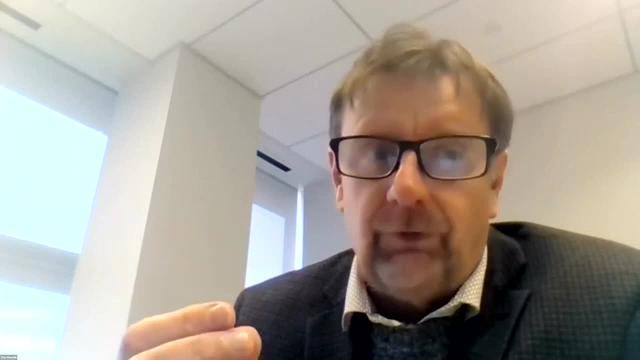 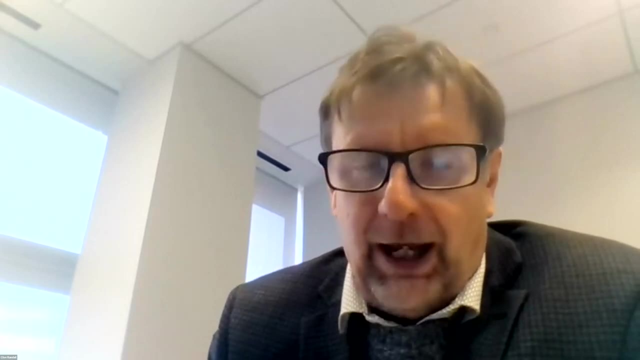 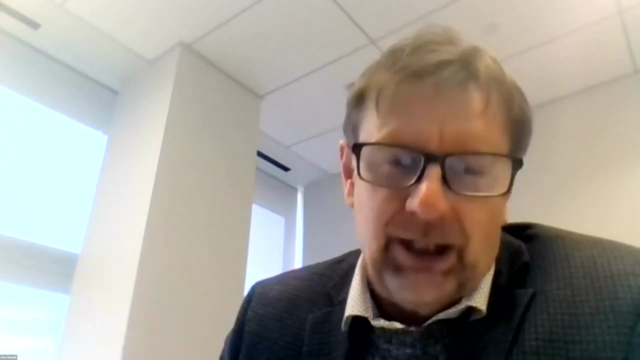 and not just dielectric properties, but we also need to understand fundamentals of chemistry, And this is something that all of us, at least myself, have a path to then continue to learn from. And so, if this is not easy, mix it, bake it, fire it. 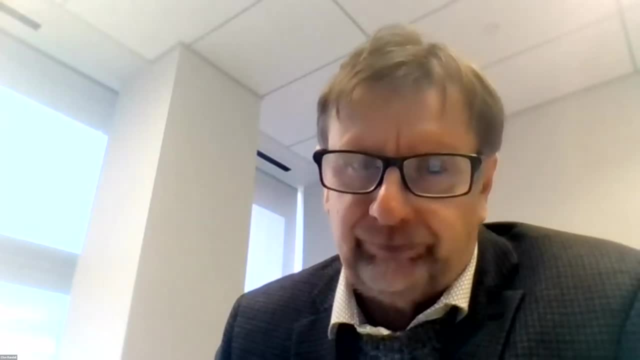 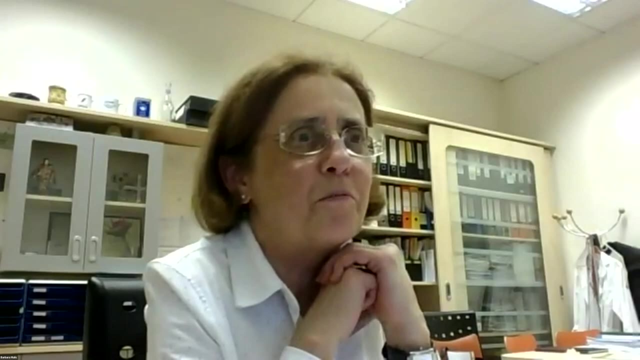 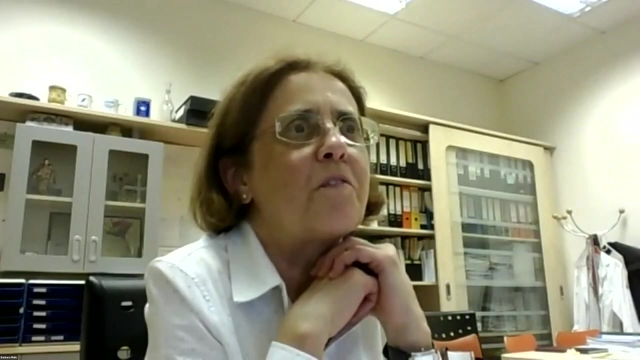 We also have to understand the subtleties of the chemistry And probably geology. A very brief last question. It's the second part of Mojtas. It's a question It's about KNN, which you showed. You mentioned that the calcination process causes defects in the particles. 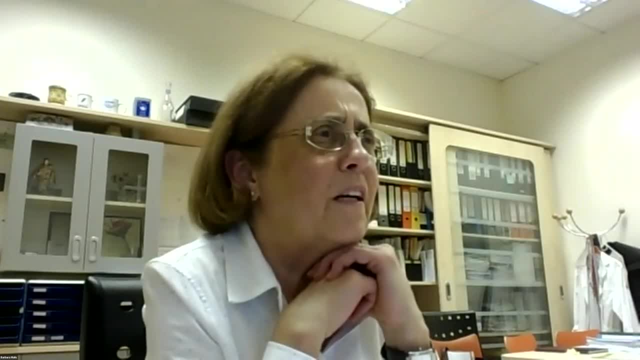 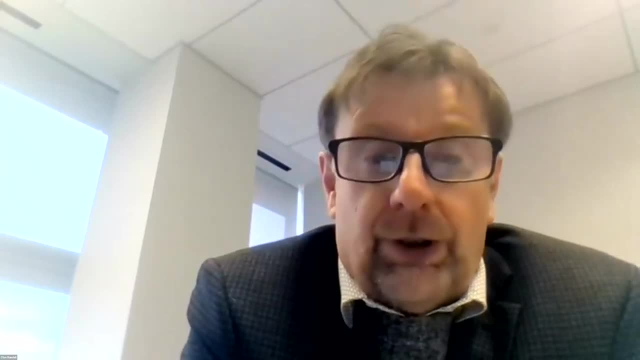 But have you got a proof for that? We're working on that for sure. We know that in our attempts to either mill things or we may be too aggressive from that, So I'm not sure if it's coming from the milling. 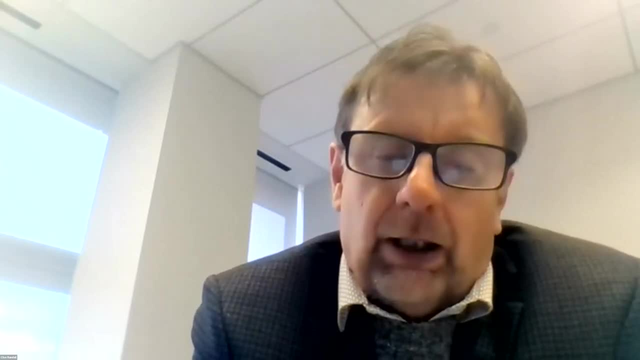 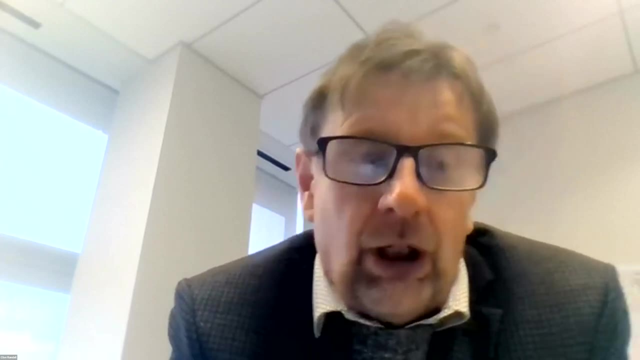 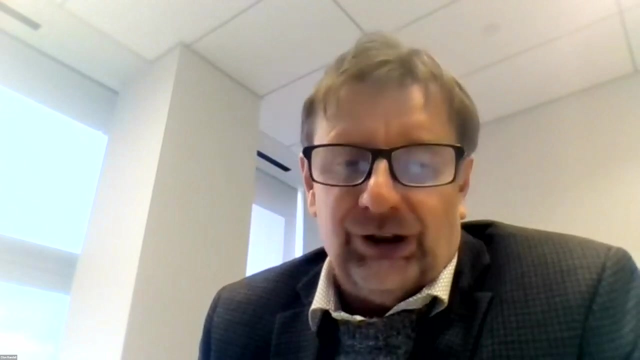 if it's coming from an incomplete or not well-controlled calcination stage. There has been, since our work. there's been a really nice paper coming out of China which has got some really nice properties. I can't remember the reference off the top of my head, of course. 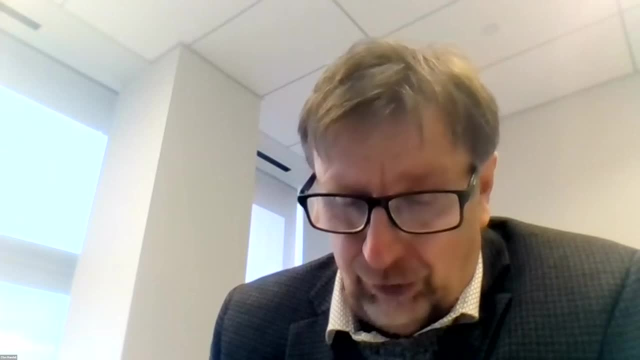 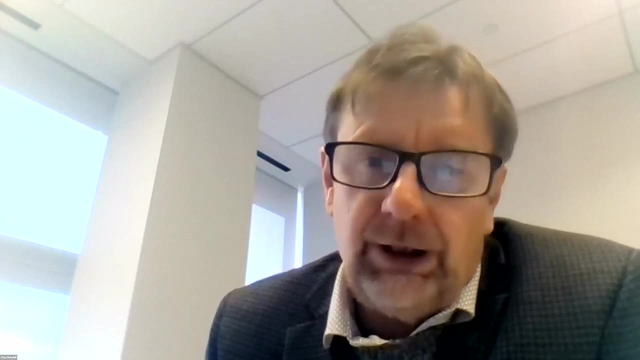 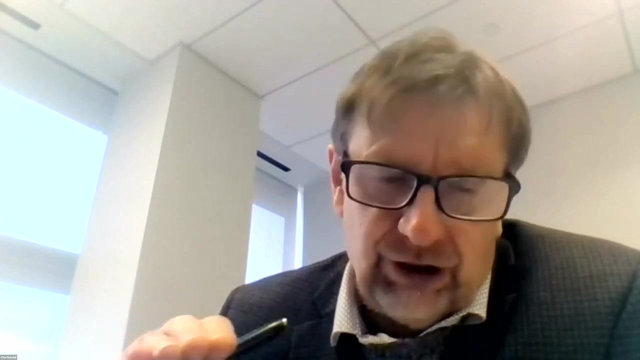 But I think if you basically do a search and you'll find it on KNN called sintering And this particular group used an intermediate thermal treatment and the temperatures were low enough. They were like mid 500 to 700. And that sort of testing would also give you clues. 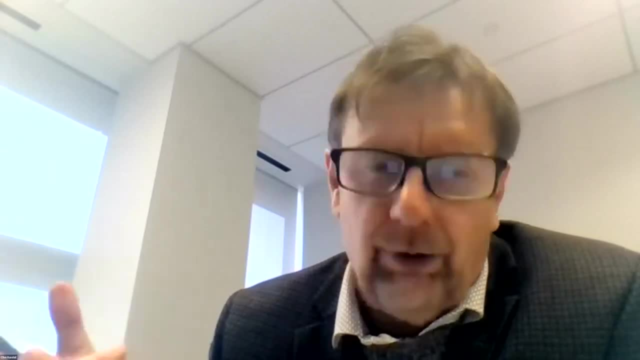 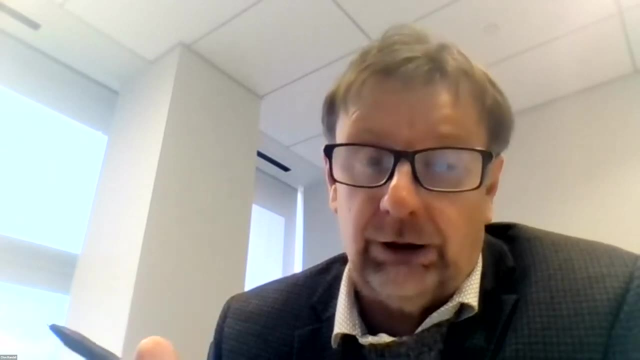 because those temperatures would also be too low to wipe out any dislocations. They would still remain in the material. So in their particular case I think they had better calcined particles to start with And they overcame some of the grain boundary problems in the system. 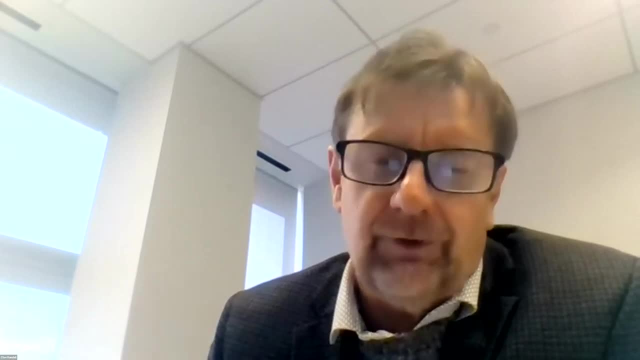 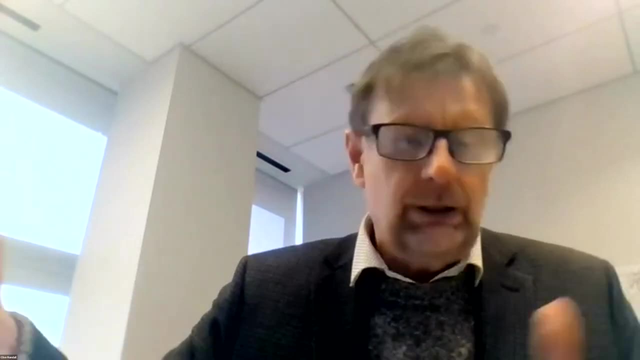 with the annealing. So I think what's really different compared to conventional sintering is that you just don't have that grain growth component going to sort of re-drive boundaries through defective and smaller grains, So you're always going to be limited in terms of piezo properties. 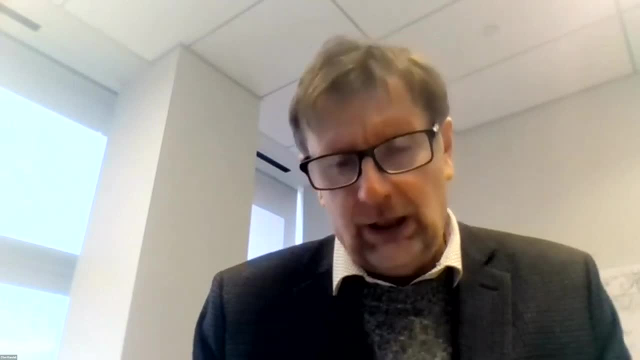 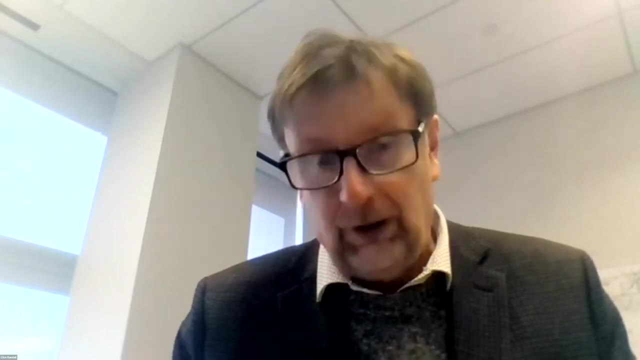 to internal microstructures, internal heterogeneities and also smaller sizes, because the densification favors densification over grain growth. So you don't have the luxury that we'd like to have. You don't have the luxury that we normally have in the conventional sintering. 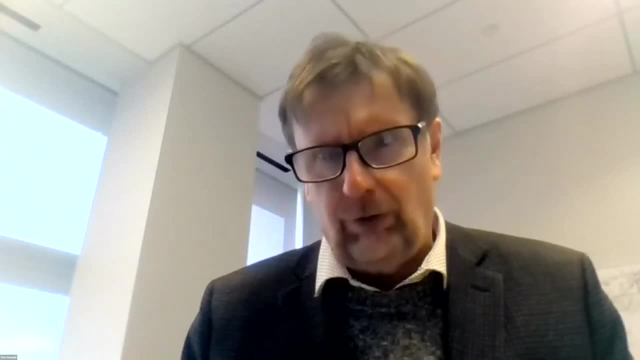 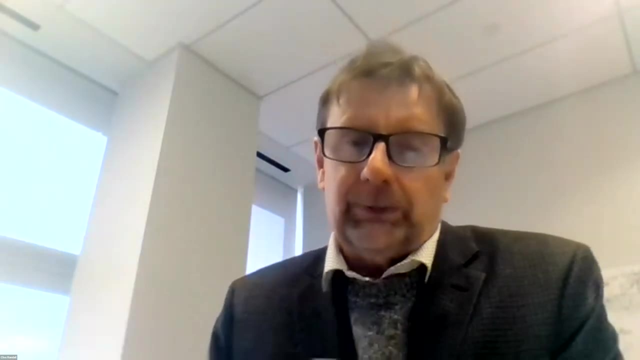 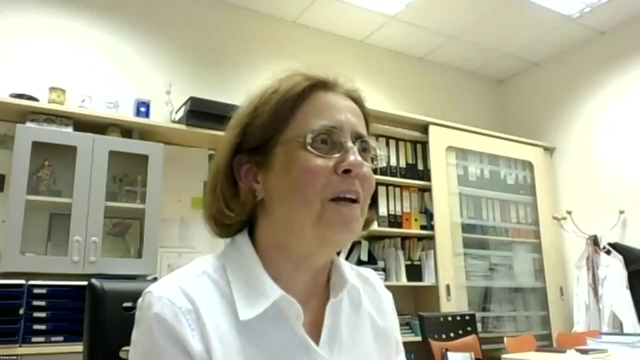 where we will drive something by a factor two, three, four in terms of grain growth, even for the most better controlled finer grain microstructures. Okay, Thank you very much. As you said earlier, the details should be very carefully checked. 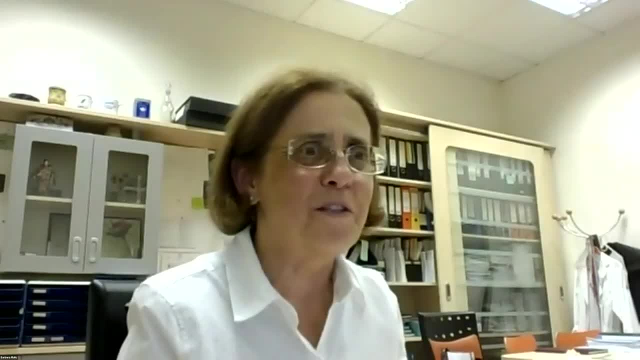 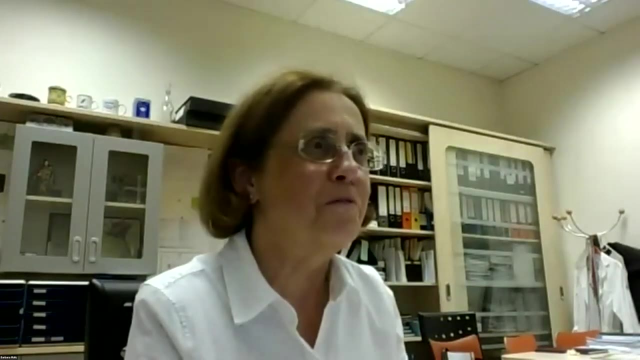 It's impressive how much you have learned in only five years, And I'm sorry to stop the discussion because You have now a defense, as I understood, and there is no time, But I hope there will be in near future chances to talk in person. 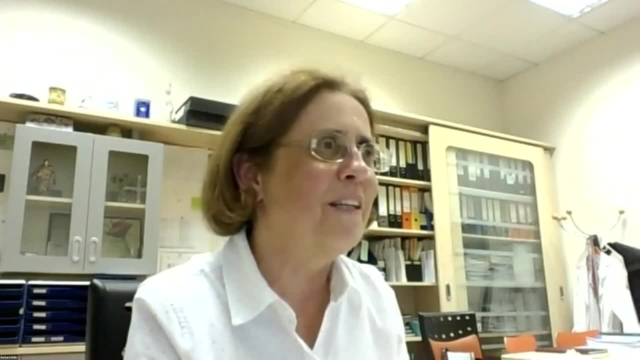 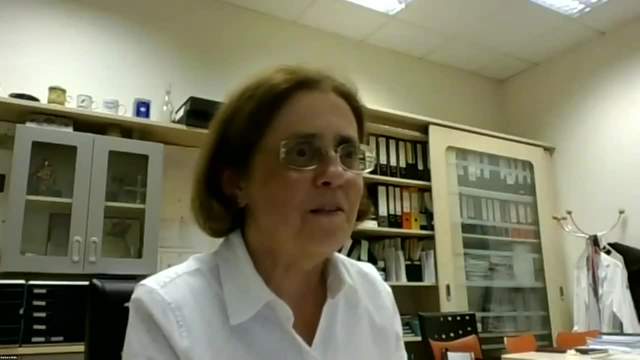 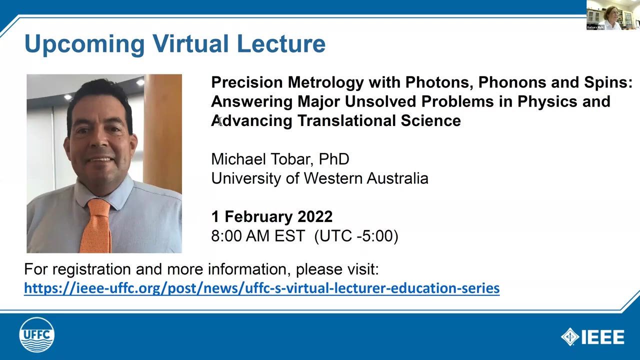 So, Clive, once again thanks a lot for this really interesting lecture and hope to meet you soon in future. And as we are now closing the session, I think it's the time to Remind you that there will be another lecture and 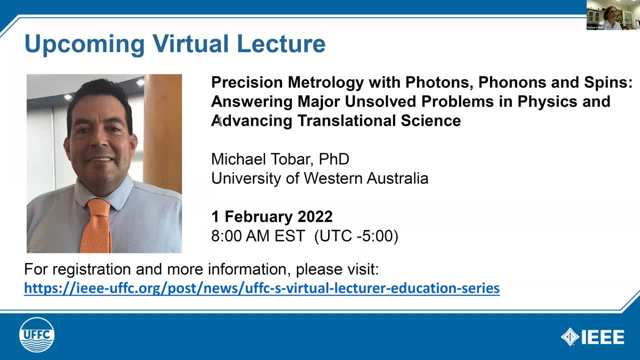 Well, more lectures, And the next one will be on the 1st of February and it will be from Michael Tober from University of Western Australia. It's a long title. Please read it by yourself. So thanks everyone. 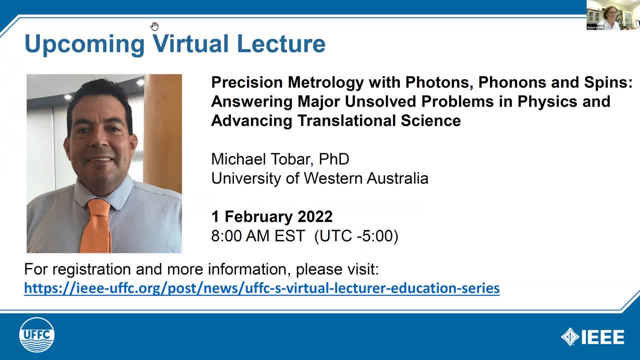 Thanks, Clive. I hope you're not already running to your next task And thank you for listening to this lecture. Thank you very much, Barbara, Thank you organisers and thank you audience for participating. Great Bye-bye, everybody. Bye.